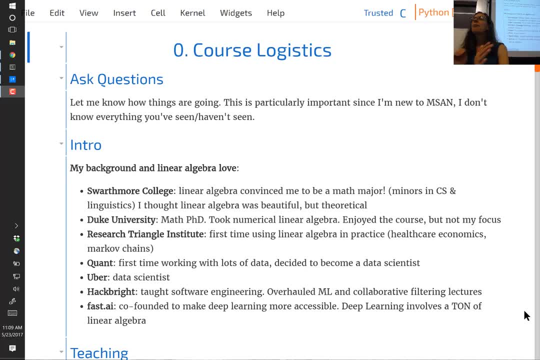 And it was still. it was a great course. I'll be kind of teaching with a very different approach and focus, though, from a traditional course. I wanted to highlight: I had an internship My last year of graduate school in healthcare economics, and I think that's the first place where I was really using linear algebra in like. this is a business where these people are using linear algebra every day. 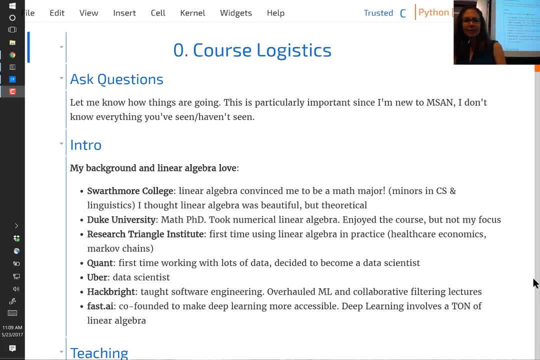 And we'll actually see an example pretty similar to some of the stuff I did in a moment. Yeah, I worked as a quant for two years. I was: oh question, Oh, that was Stephen Marr. Oh, oh, that's awesome. 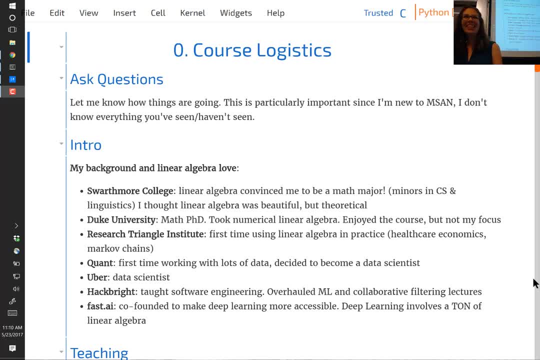 Very cool. Yeah, that's so great. So yeah, I was a quant for two years, which is a lot of working with data And I would say linear algebra, kind of yeah, having tables of data, And that convinced me to become a data scientist. 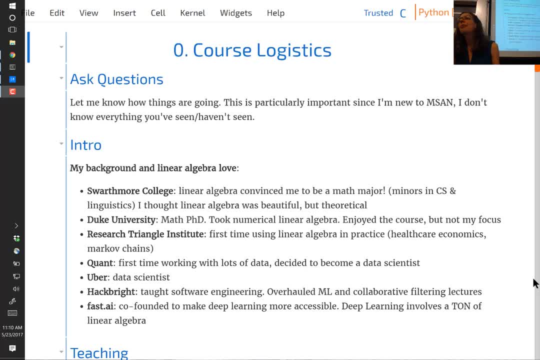 I was at Uber and I taught software engineering at Hackbright That's, it was mostly software development. I did get to overhaul their machine learning and collaborative filtering And I did some of my engineering lectures, which was exciting. And then one year ago, Jeremy and I started fast AI to kind of make deep learning easier to use. 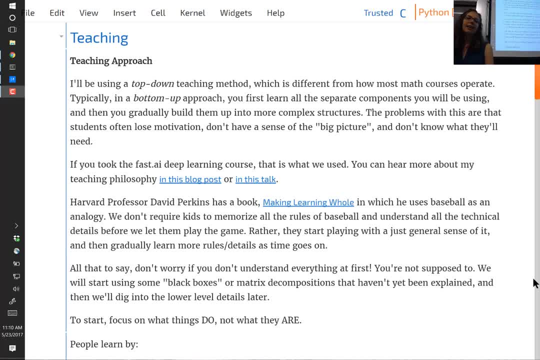 Yeah, so going into teaching this is a different. it's a different approach than most math courses. It's going to be top down, So in a bottom up approach, which is kind of the more common one in math, that's where you first learn all these separate components that you'll need. 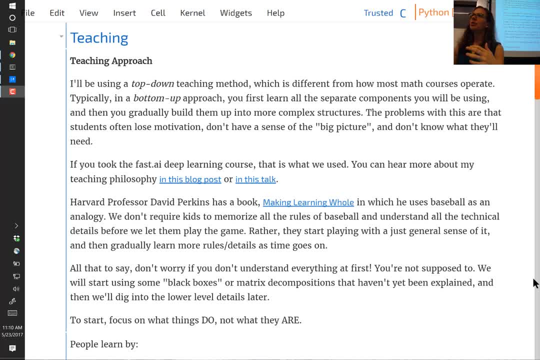 And then you kind of build things of increasing complexity, Yeah Yeah, Yeah Yeah complexity as time goes on and you know more components, and that's kind of tough because people lose motivation, they don't have a sense of the big picture, and what I'll be doing instead is kind of starting with, kind of doing. 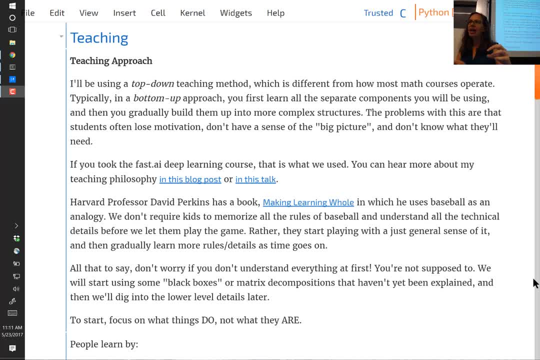 interesting things using algorithms, and then we'll kind of go into more depth and break down the pieces, and I apologize if you heard I give a talk on this at the Friday seminar a few weeks ago, so sorry if this is repeat, but there's a wonderful book called making learning whole, where a Harvard professor 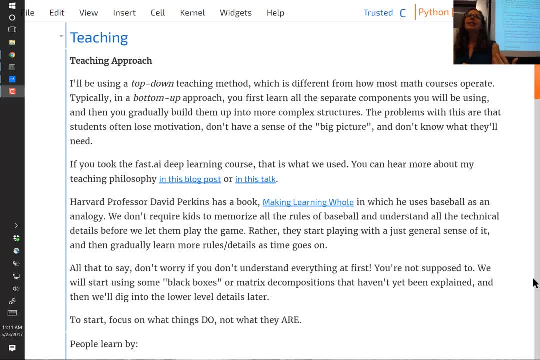 uses an analogy with baseball and says: you know, we don't require kids to learn all the memorize, all the formal rules of baseball before they're allowed to play. you know, we let them play and then over time they learn more and more of the formal rules. yeah, and so I kind of don't worry if at first you don't understand. 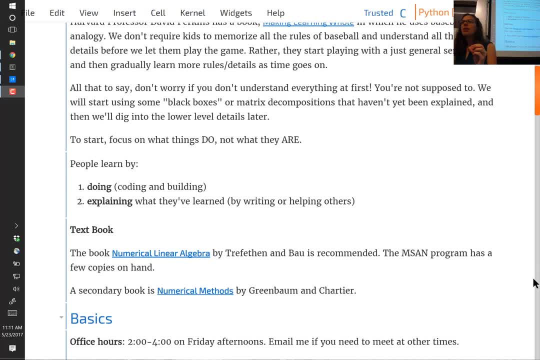 everything that's going on. that's kind of the point, and focus on what things do as opposed to what they are. so with these matrix decompositions, it's really important to know what's going on and what's going on and what's going on and what type of matrices are you getting back from the decomposition. and then 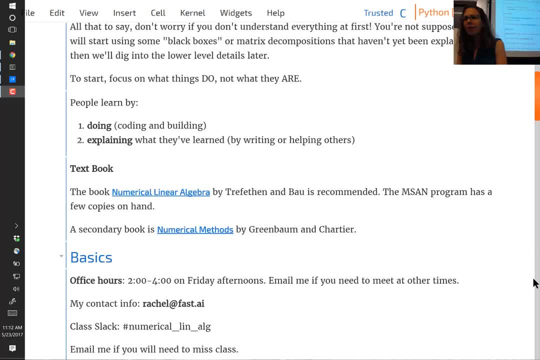 over time we'll kind of get into how would you program them. so for the course I have two textbooks. neither of these is required and I've asked Kirsten to buy a few copies to have on hand. so my number one choice is numerical linear algebra by Trevathan. it's a really well written book and I'll say kind of what I'm. 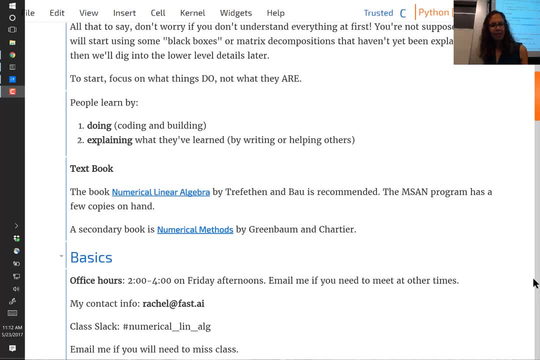 referencing parts of it, and then kind of a secondary book that I like is called numerical methods by Greenbaum and Chartier, and this is actually intended for kind of senior undergrad courses and it includes numerical linear algebra but it also includes Monte Carlo methods, numerical differentiation, and I think 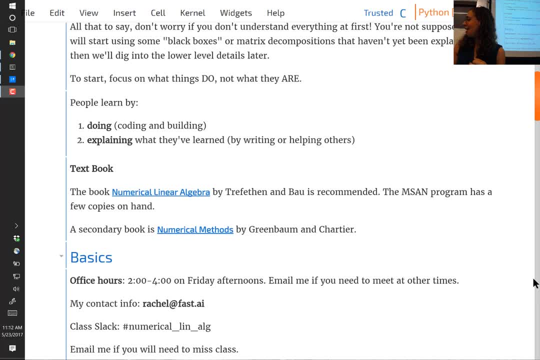 it's a really interesting book and it has a lot of applications. it's a fun fact: Chartier is actually he's a math professor, but he trained as a mime under Marcel Marceau and I saw him perform at a math conference on how to kind of use miming to teach math. but it's 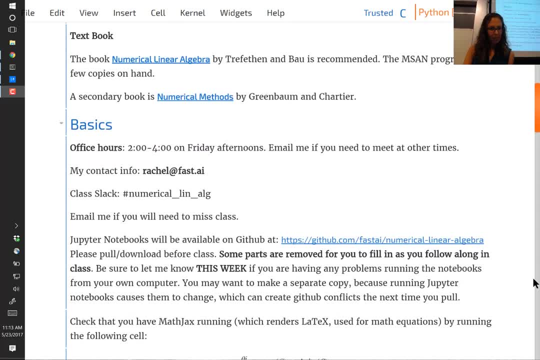 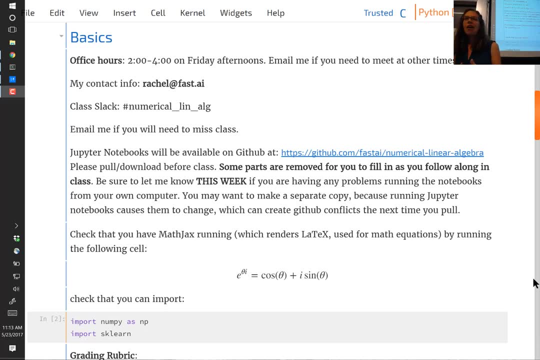 a very kind of accessible book. so I was gonna hold office hours from 2 to 4 on Friday afternoons after the seminar and if that doesn't work, feel free to email me about another time. yeah, my email is Rachel at fastai, and there's a. 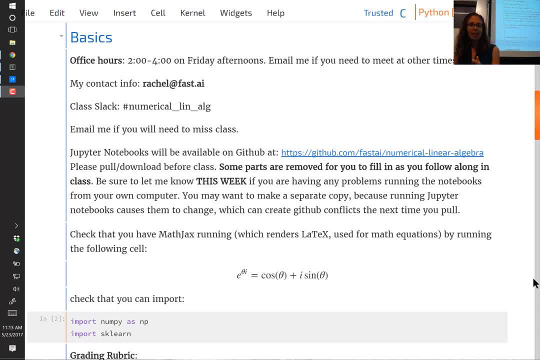 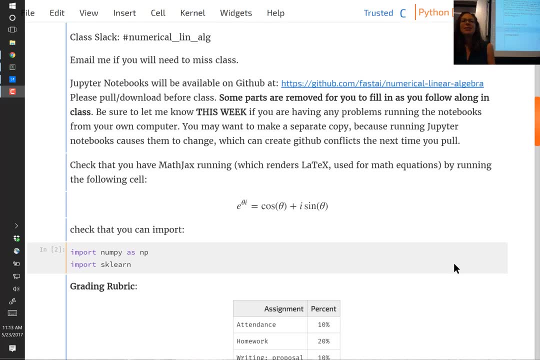 class slack channel, although I haven't done anything with that yet, but I'll send you invites. there's the link for the github, oh, and then I wanted to, so this is important to note. kind of a difficult thing about Jupyter notebooks is even just running them changes the code and so you can get merge conflicts. 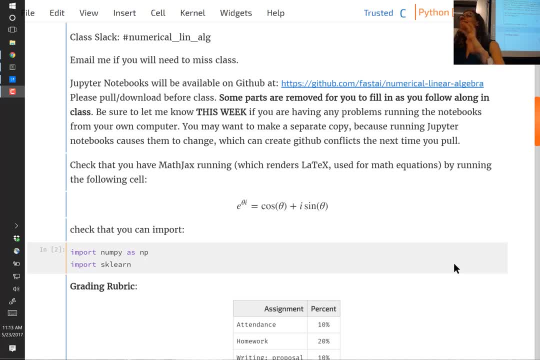 if you've cloned the repository, and so it's up to you if you want to deal with those, or it might just be easier to kind of download the notebooks, and there are places that I kind of leave blank for exercises. so the idea is you will be. 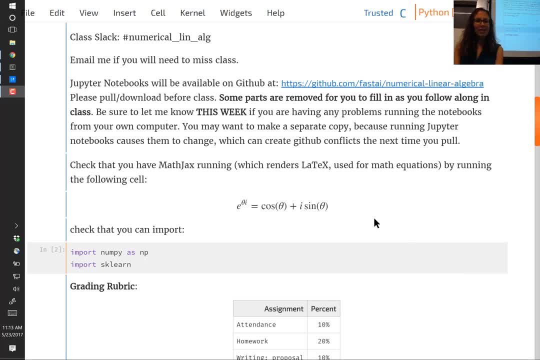 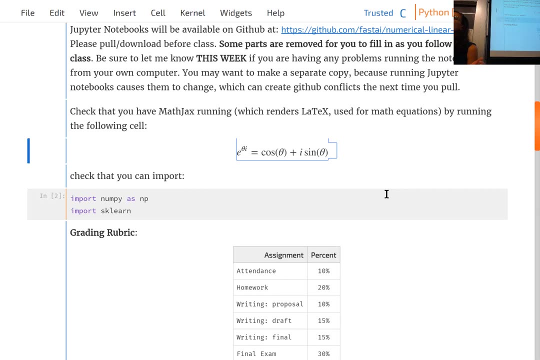 doing some coding in them as well and I just included these to check. if you have math jacks running which renders LaTeX- and I believe if you're using anaconda, that's automatically installed. but let me definitely let me know in sooner rather than later if you're having any trouble with the setup for this or any of the imports or 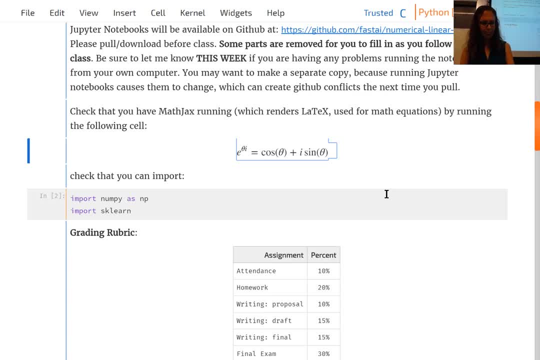 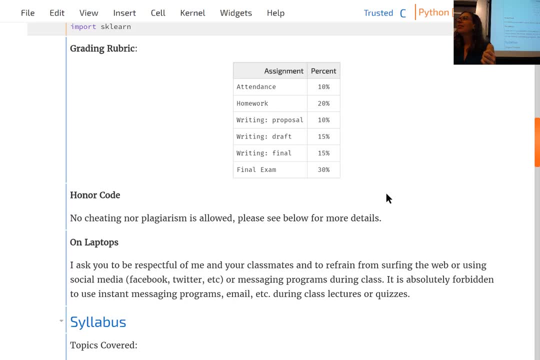 anything, because I definitely want you to be able to run these notebooks at home. so, yeah, here is a. actually I should check any questions so far, okay, here's a grading room work, so there'll be some homework assignments and I'll give you always a full week to to do the homework from when I, when I give. 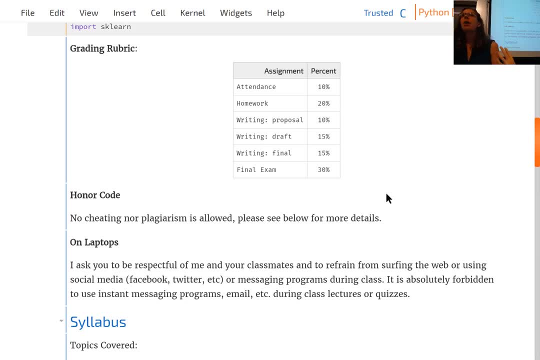 it I want. there's gonna be a writing assignment for this course and you can choose the topics- and actually I'll say a little bit more about that in a moment. but that's kind of broken into three pieces: just your proposal, your draft and then the final, and then there'll be a final exam. 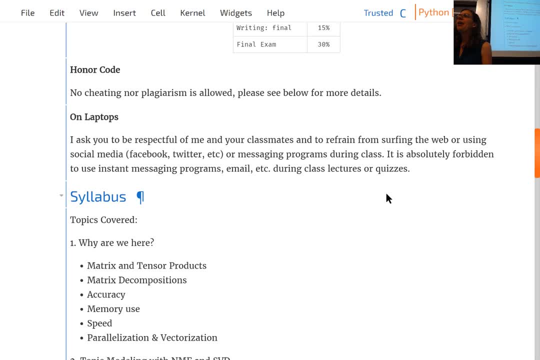 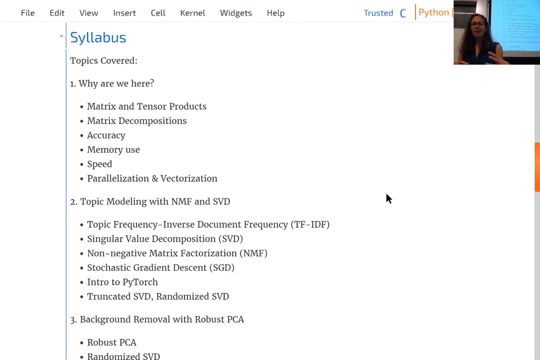 so, um, no cheating or plagiarism is allowed and um, you know we have the standard honor code from USF, which I'm sure you're really familiar with. from this point, um, for laptops, please avoid surfing the web or using social media or messaging during class, cool. and then here's a, a syllabus. I'll just say, kind of the um, the way it'll work is kind. 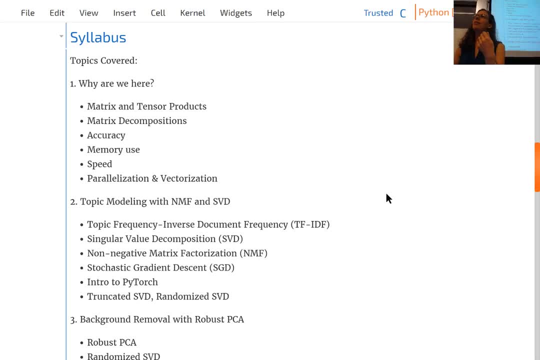 of each lesson is mostly centered around an application and then we'll kind of dive into the algorithms and tech or techniques that are used for that application. but it's kind of this: almost application first, uh approach. so we have the introductory lesson, which is a little bit. 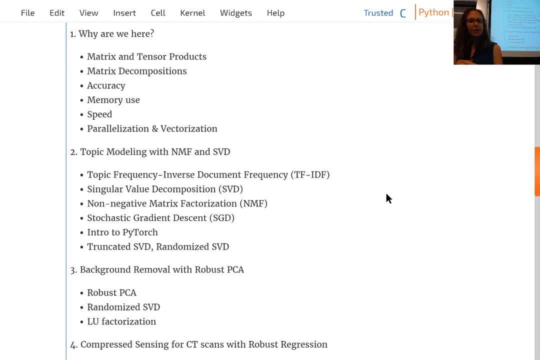 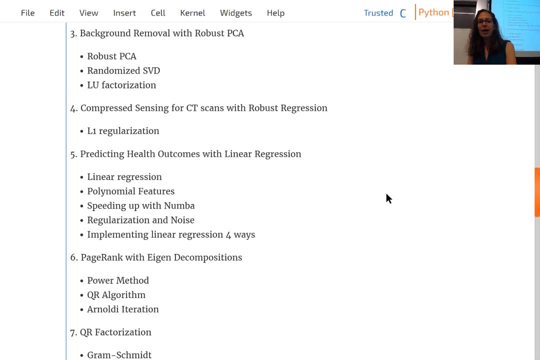 unusual and that'll be less code and it's more kind of introducing concepts. but then we'll talk about topic modeling using nmf and SVD background removal with robust PCA compressed sensing for CT scans, which are kind of some really interesting looking uh kind of CT scan like pictures. 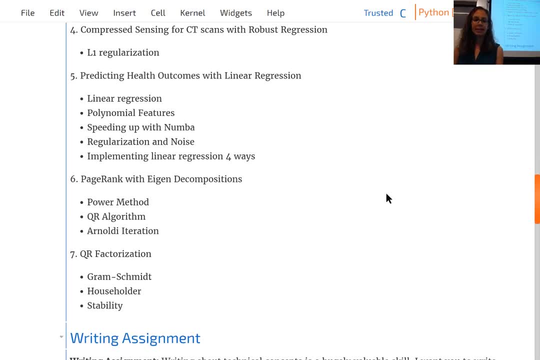 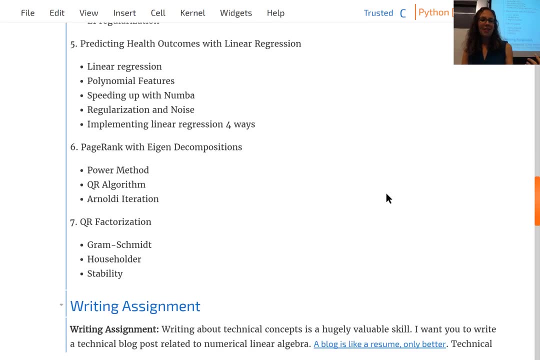 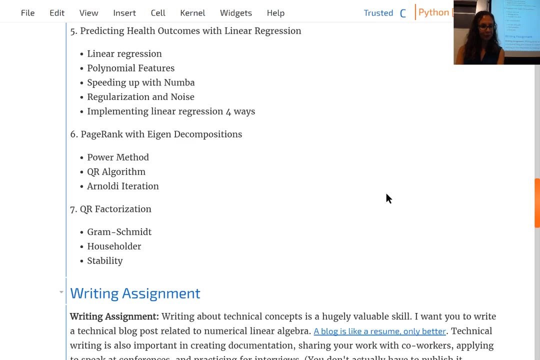 um predicting health outcomes. this is on a diabetes data set page rank to go through eigen decompositions and how you program those, and then, finally, the QR factorization, which will have shown up in almost all of the previous lessons as a tool. okay, so about the, the writing. 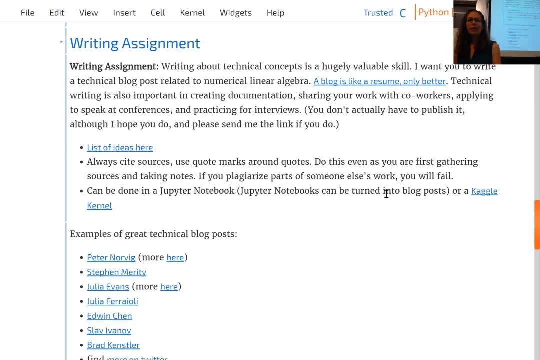 assignment. um, yeah, writing about technical concepts is really valuable. I hope that you'll publish it as a blog post. you don't have to. um, if you do, it's a really good name to kind of get your way to get your name out there, something to show to future employers or when you're applying for jobs. um, technical writing is. 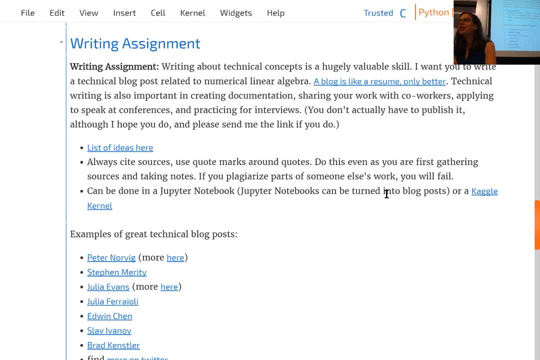 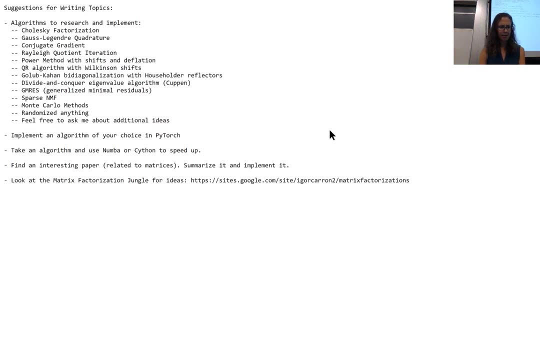 also important when you're creating documentation at work, kind of explaining and sharing your ideas with co-workers, applying to speak at conferences and practicing for interviews, kind of just even practicing, like, how do you explain what you're doing? um, so I have a list of ideas, oh, and I actually 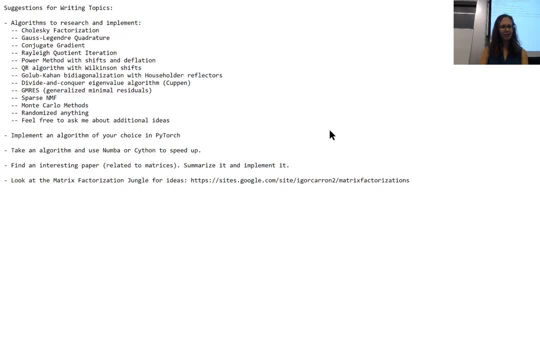 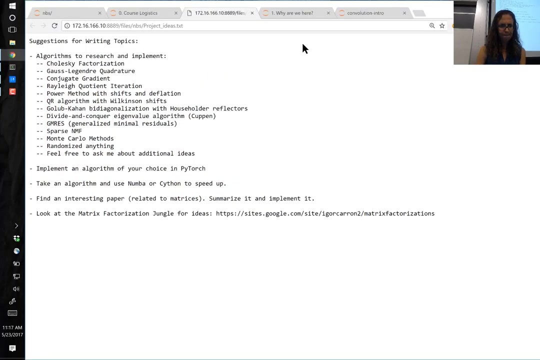 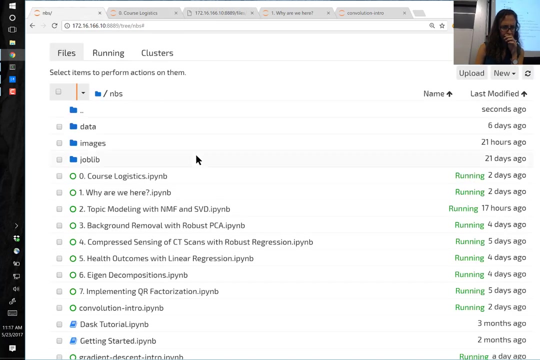 um, oh yeah, is this? I might have an updated version. hold on a moment. yeah, this is the old version. yes, well, escape is not taking me out of full F11, oh okay. well, I'm running this from a different repository. let me just go here. oh no, that's the issue, uh. 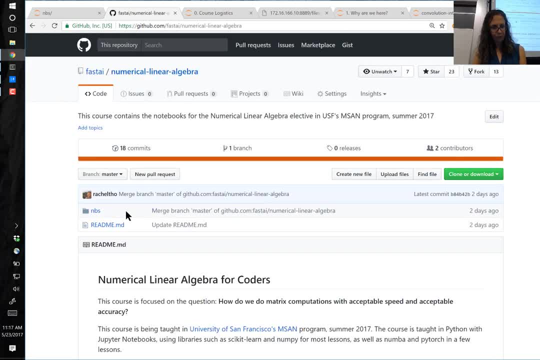 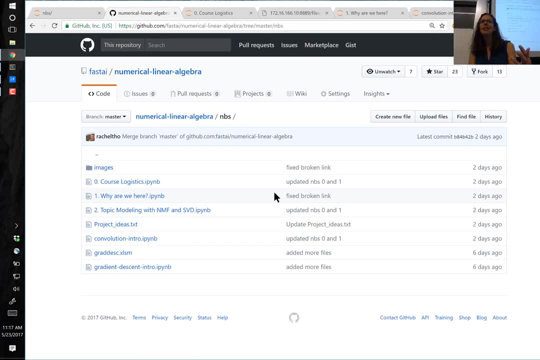 foreign. um, and with all these ideas, these are just suggestions. if you have a different idea that's not on the list, feel free to ask me um about it. I really want it to be another topic. one second and yeah, this is all I have. um, yeah, thank you so much for being here, thank you so much for having me. um, I really wanted to apologize for all the questions that you posted and, um, it's been a six hours and a half, um, I know I'm doing great. that's, that's a great thing, um. so, thank you so much for listening and I appreciate it and I hope you have a great most of the time. I know I'm not. 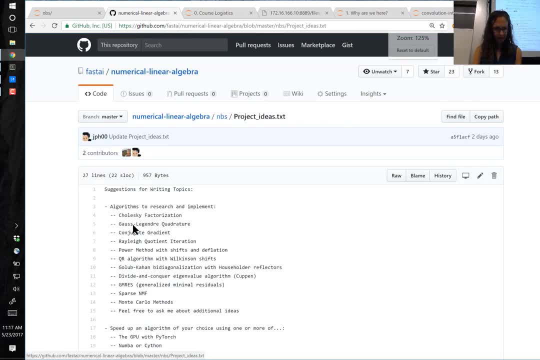 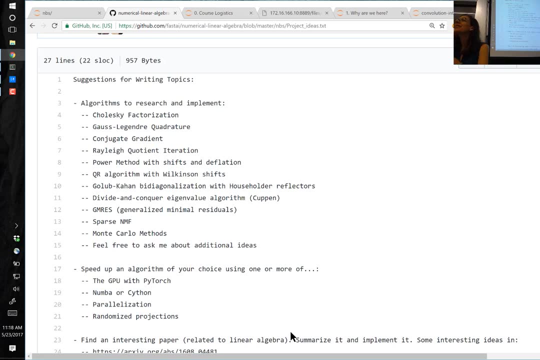 it to be something that you're interested in learning more about, so I have a list of. there are so many numerical in your algebra algorithms, and so we'll get into most of the core ones, but there are a lot that we won't have time to cover, so you could choose one of those. so here's a list of several of. 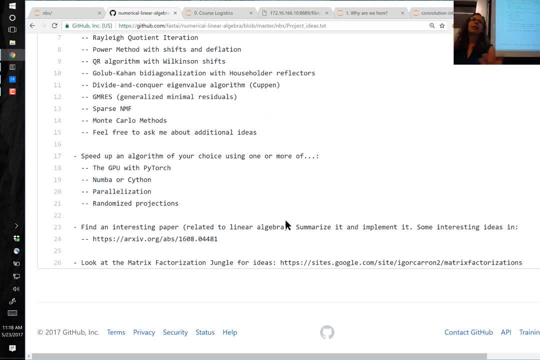 them. you could also speed up an algorithm of your choice- and that could either be something that we've covered in the course or not- using the GPU and pie torch, and we'll be talking about how to do that in the first lesson, number scython, which will cover parallelization or randomized. 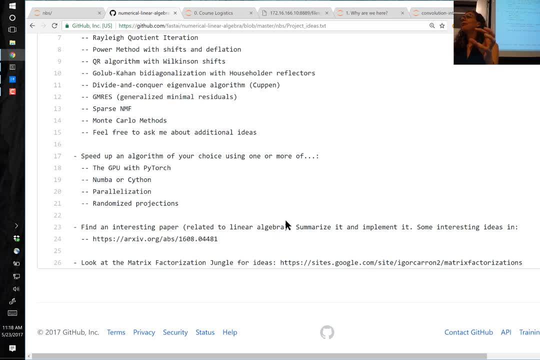 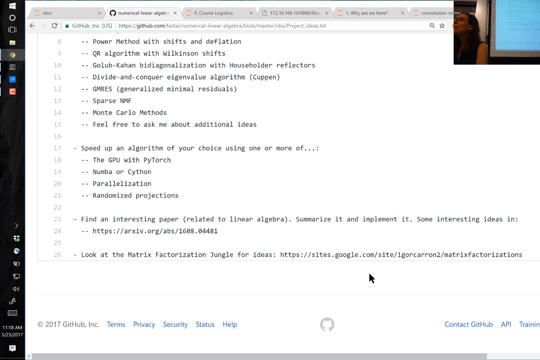 projections, so randomized algorithms are a really interesting area that give you a kind of a lot of speed up. you could also find an interesting academic paper that you've been wanting to read and summarize and implement it, and then here let me go to this link, and there's something called the matrix. 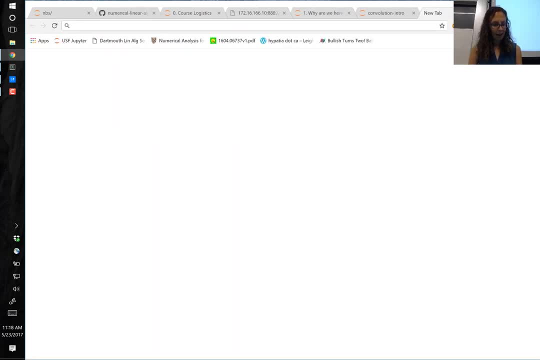 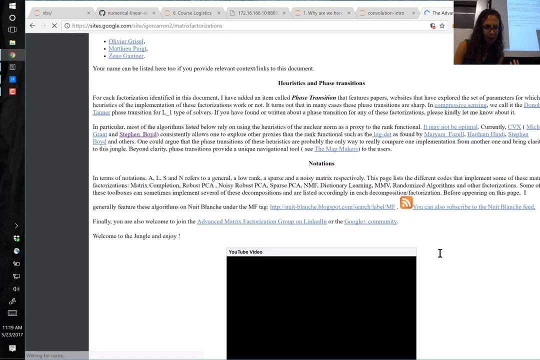 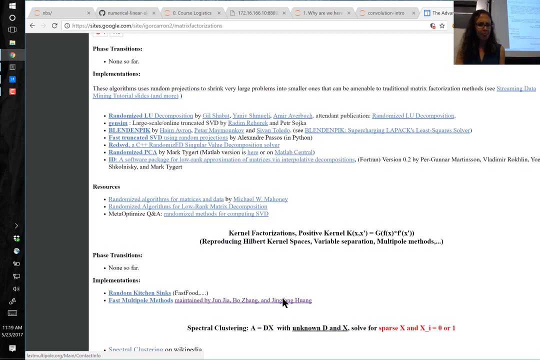 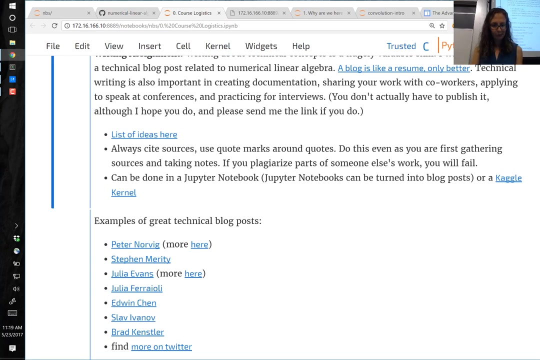 factorization jungle. it's just a handy web page that someone put together with kind of a list of a ton of different matrix algorithms, and so if you scroll they're kind of whole sections on different concepts, logistics, oh, and then I posted a link to oh one. 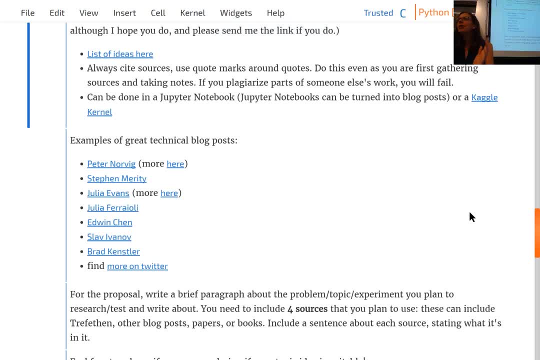 other thing I wanted to say: so you can do your blog post or your writing assignment as a Jupyter notebook. I mean, you can also do it as a Kaggle kernel and you can Kaggle kernels, kind of our Jupyter notebooks. but that's another kind of great way to share your work and you can also share data sets. 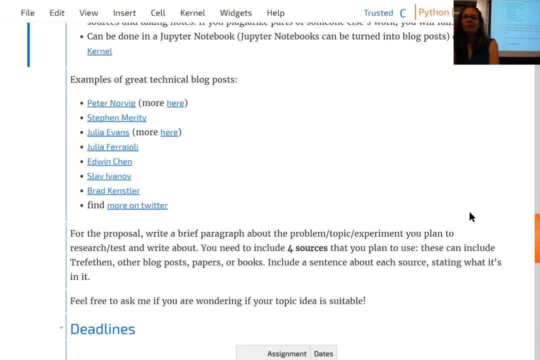 that way, and then I've linked to several number of technical blog posts that I like and I think that's something that's kind of good to get into the habit of- and maybe after you graduate and have more time- but just kind of reading, reading other people's blog post. 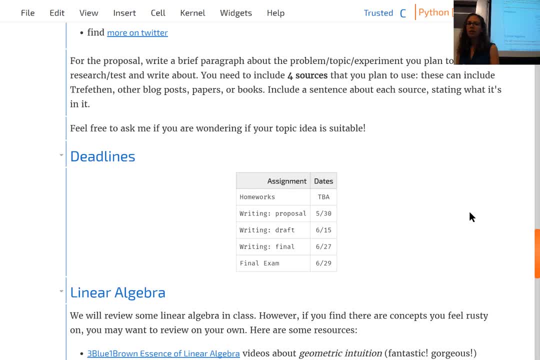 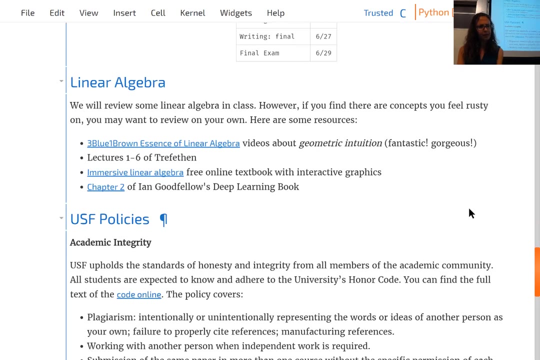 and so for the proposal, that's just gonna be a brief paragraph about what you want to do. I should also say it could be like an experiment you want to do like, if you're curious, you know, how does- I don't know- changing this factor affect this algorithm? you can propose that. and then for sources, any questions? 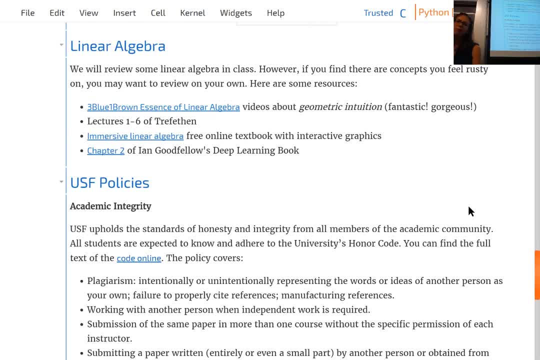 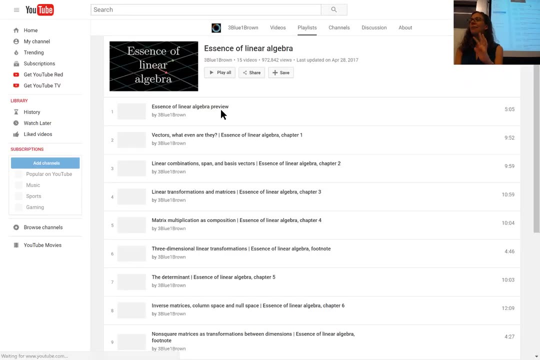 okay, so I'll try. I'll try to review some linear algebra in class if there are things that you feel like you need extra review in. these are some resources I recommend. one is three blue, one brown. this I would recommend to everybody for any reason. it's just the really fantastic videos. 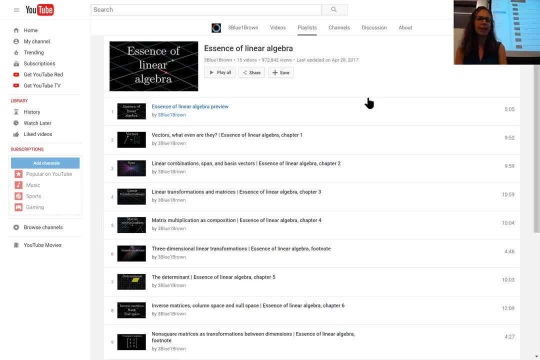 and I'll probably show one in class and in a later lesson. but it's a very, very kind of geometric and visual perspective on linear algebra and so it's very different from how most linear algebra courses are taught. the guy who created these wrote his own graphics library because 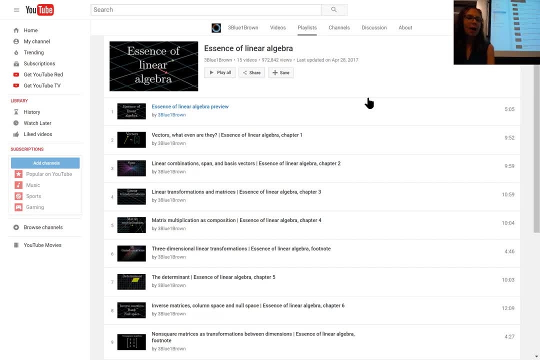 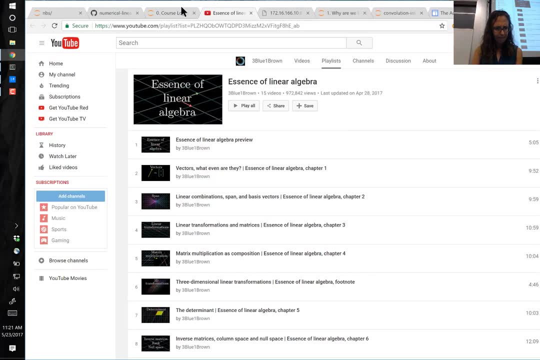 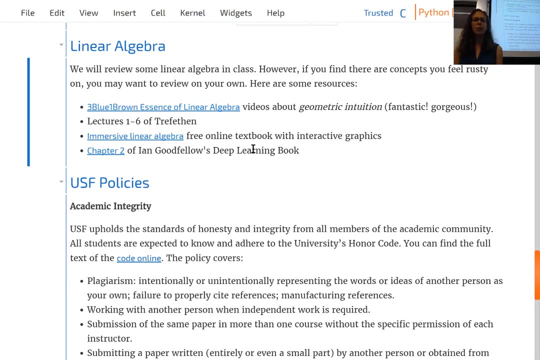 and you wanted to do things that he wasn't able to do otherwise, and but they're really beautiful, and so if you're a visual learner, I would definitely recommend them. there's also an immersive linear algebra free online textbook. chapter two of Ian Goodfellow's deep learning book is all about linear algebra, and that's kind of 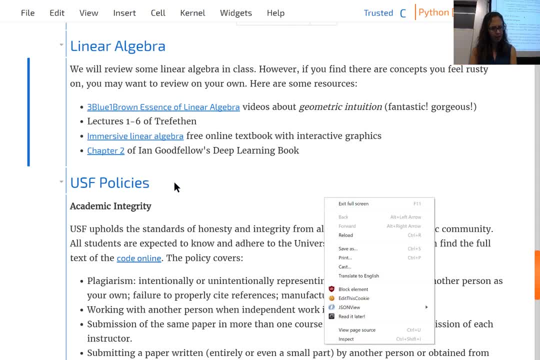 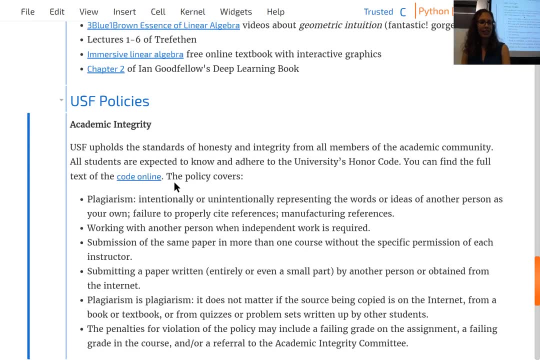 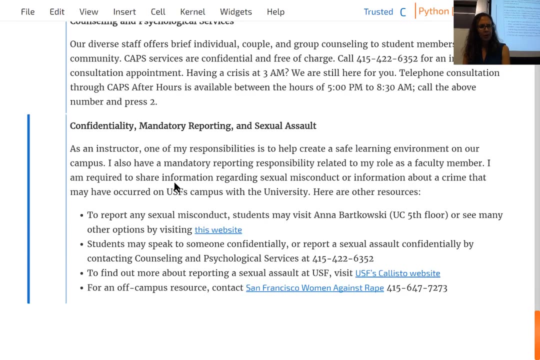 coming from a machine learning perspective. yes, I think that's it to. then the usf policies are in here, but again, you should have seen these, I think, in most of your courses about academic integrity, accommodations for disabilities and so on. 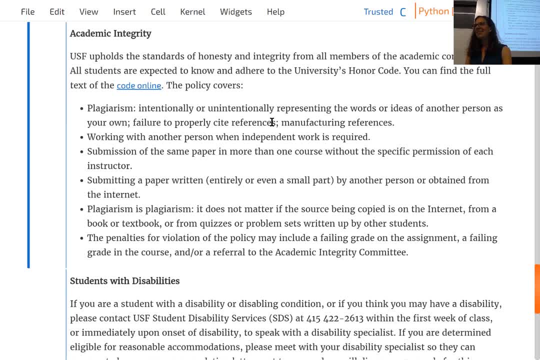 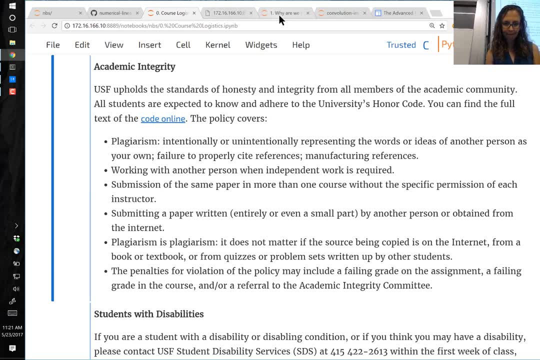 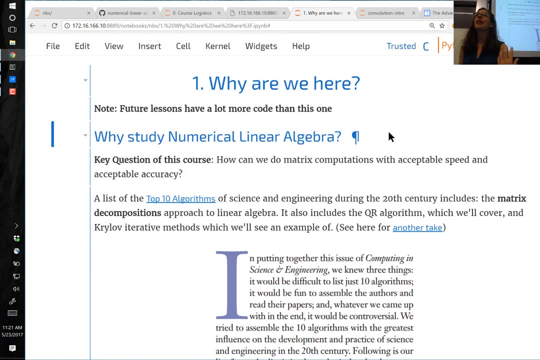 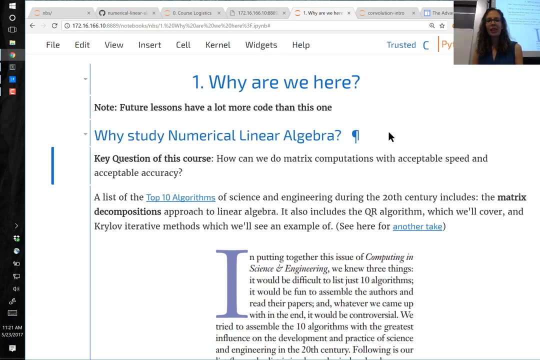 All right, you guys ready for the first lesson. And again, this is going to be less codeful than future lessons, but it introduces some really interesting concepts, I think. So, kind of, why are we setting this? Let me go back to full screen. 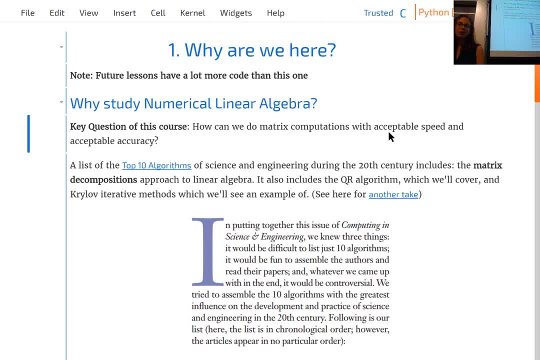 So the key question of this course is: how can we do matrix computations with acceptable speed and acceptable accuracy? And this is from a news algorithm or not a news algorithm, a channel. It's a journal article that came up with the top ten algorithms of science and engineering. 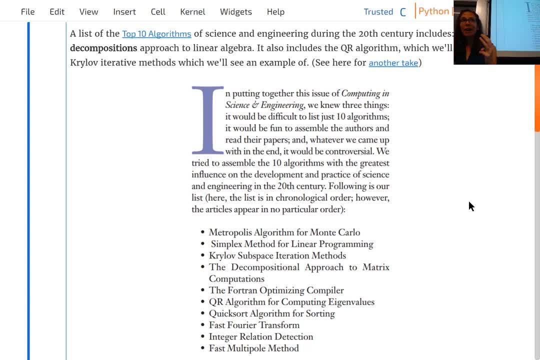 during the 20th century And three of the things on the list we will cover in this course which is exciting, And one is the idea of matrix decompositions as an approach to linear algebra itself, because it's such a powerful idea. So a lot of this course is about breaking matrices into other matrices that are going. 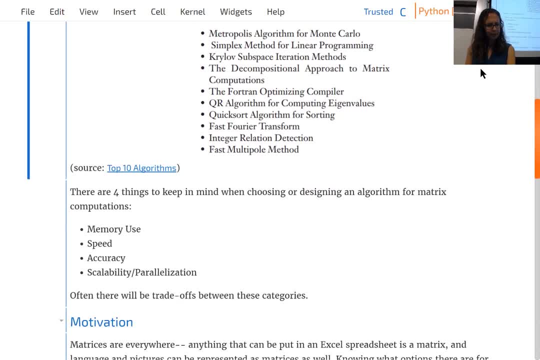 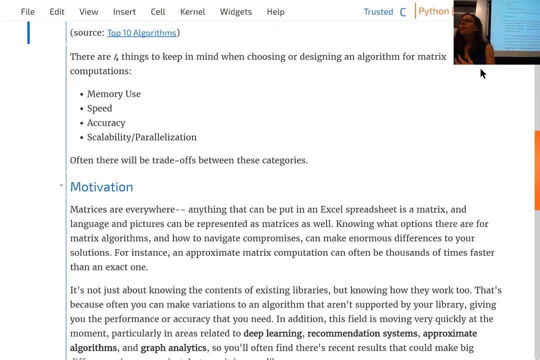 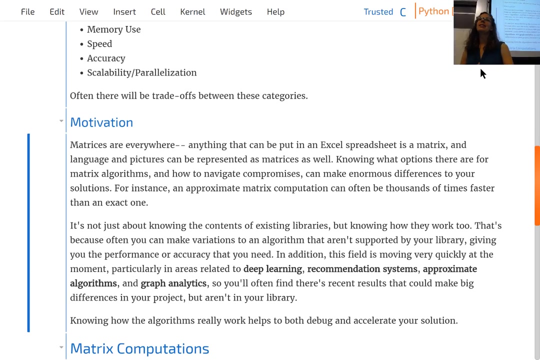 to be easier to work with, And so there are going to be four things to keep in mind. We're going to go into each of these in a little bit more depth: Memory use, speed, accuracy and scalability. And then kind of on the motivation of doing this. 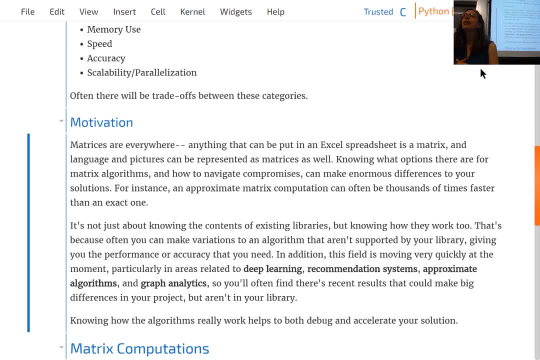 So a lot of the things we'll talk about could be done in Scikit-learn or SciPy. It's really great to know kind of how those libraries work. In case that you're interested in learning more about this, you can go to our website. 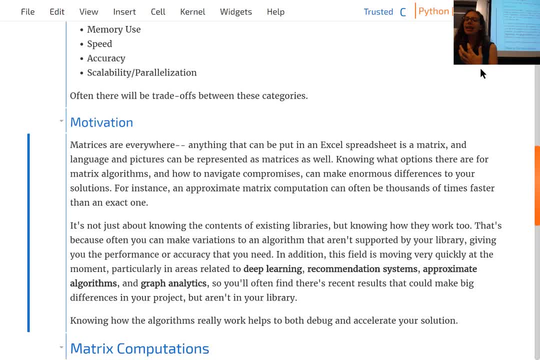 and you'll find a lot of information there. So if you're interested in learning more about this, you can go to our website and you'll find a lot of information there. In case you want to do a variation that's not accounted for, knowing the tradeoffs that, 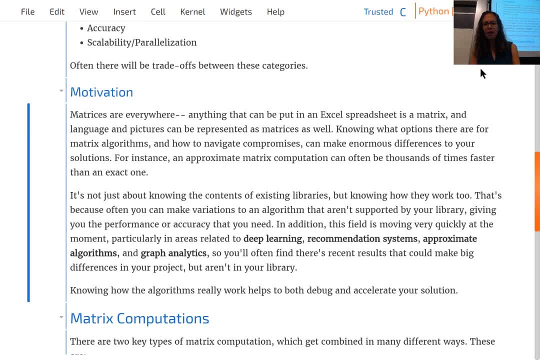 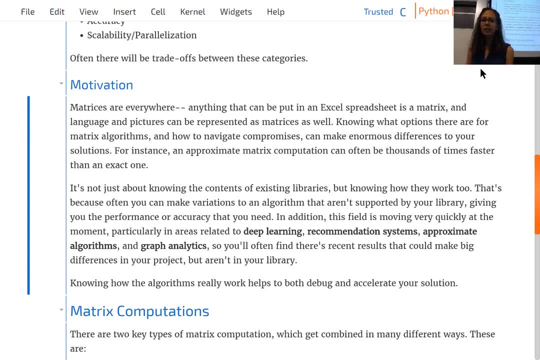 you're making when you choose between different options. Also, a lot of these fields are moving very quickly, and you might find new results that haven't yet been implemented in one of these libraries, particularly the areas of deep learning, recommendation systems, approximate algorithms and graph analytics. 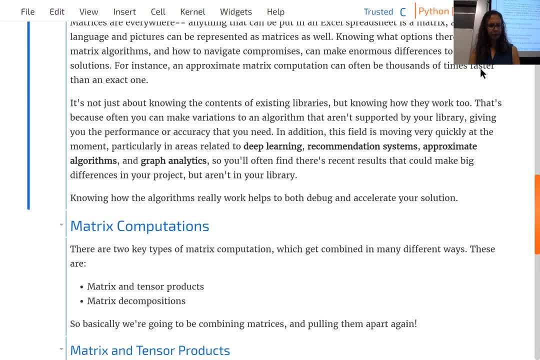 There's a lot of research happening in all of those right now, And so, yeah, Knowing how to debug all of the graphs, All right, So that's a good way to go about it. And then the other thing about the rhythms. 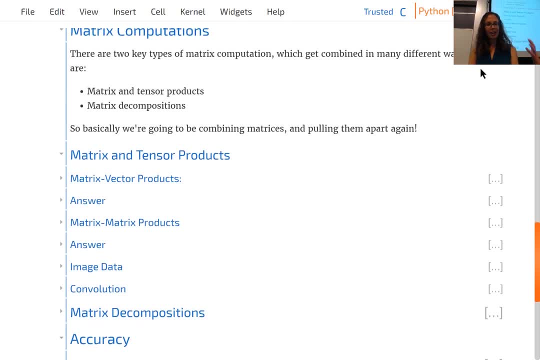 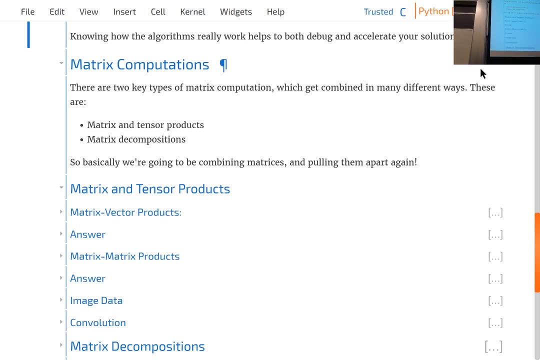 The rhythms can really kind of accelerate your work. Sorry, Knowing how they work helps you debug them, but knowing how to debug them also helps accelerate what you're doing. But you can make them look faster. Let me drink, So in this part we'll probably review. 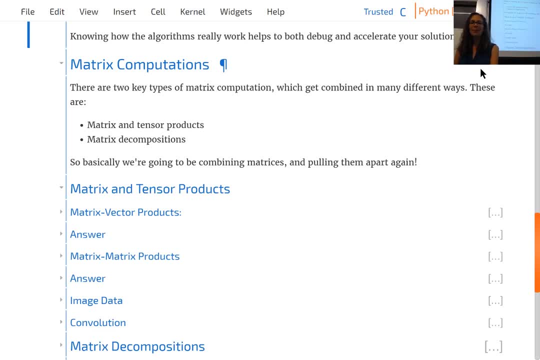 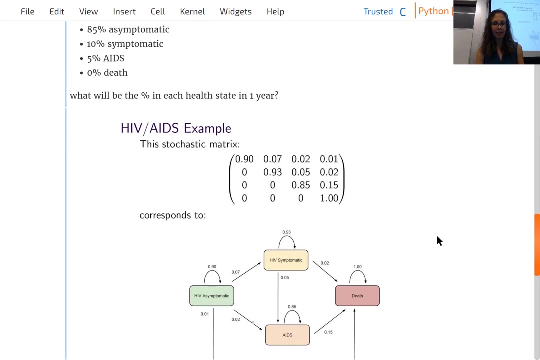 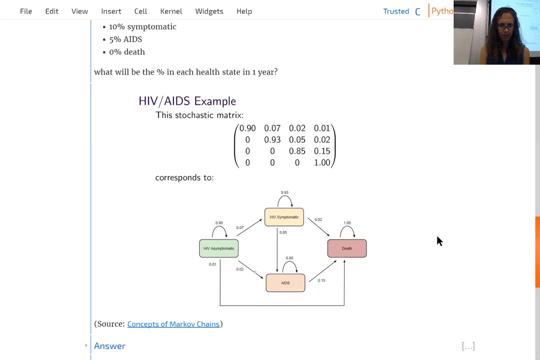 I just wanted to say there are two main types of matrix computations, which are taking products and then decomposition, putting them together and then pulling them apart. So for an example here this is a matrix. let me make this a little bit smaller, just so it can fit on one screen. 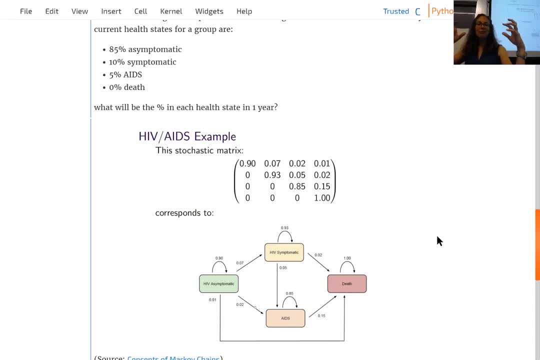 This is a matrix of- or sorry, yeah, well, it's a matrix of probabilities, but this is a Markov chain with different states of health, And so there's kind of an asymptomatic HIV stage, symptomatic full-blown AIDS and death, And these are kind of the different. 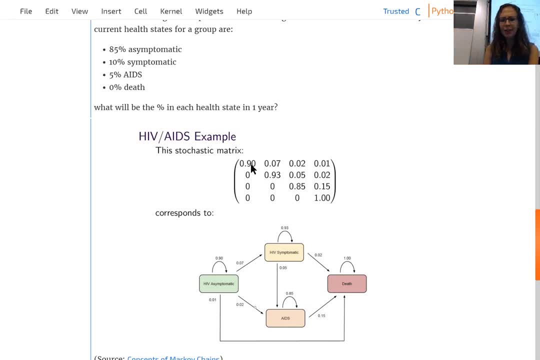 states of the Markov chain. And then this matrix of probabilities is saying what are your chances, if you're in one state, of moving to each of the other states. And so you'll notice, each row sums to one, since they're probabilities, And that's kind of the row. 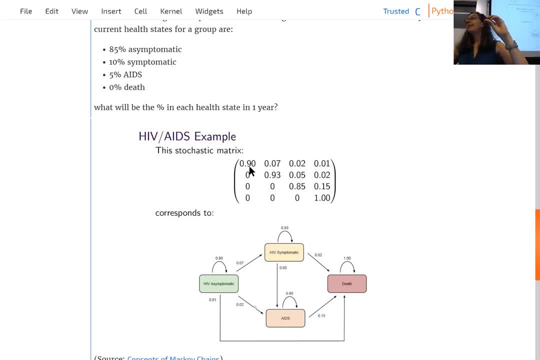 that gives you the state you're starting in The column gives you the destination state you're moving to. So I mentioned earlier, I had an internship while I was in grad school. that was a whole kind of research group that looked at problems like these. They would also take into account kind of the cost of 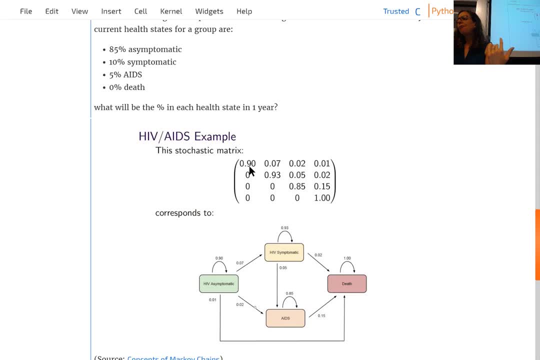 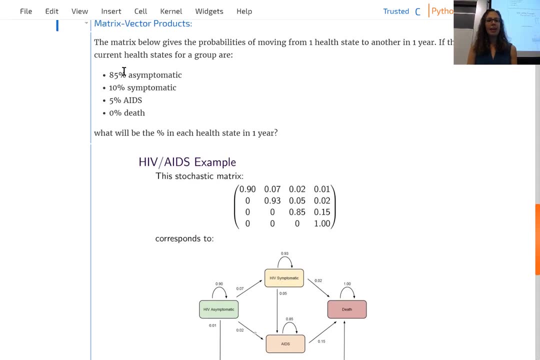 healthcare and different types of treatment and use that to kind of weigh recommendations. So here I want you to take, if this is kind of your starting vector of what you know- you have a group of people: 85 percent are in the asymptomatic group, 10 percent are. 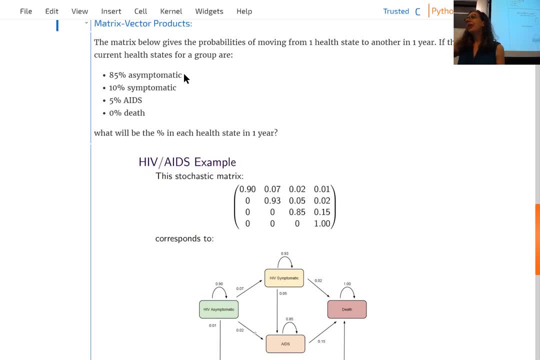 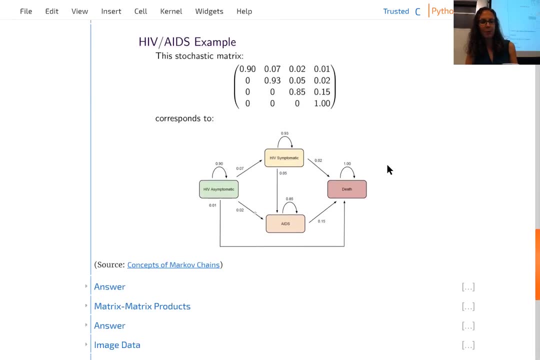 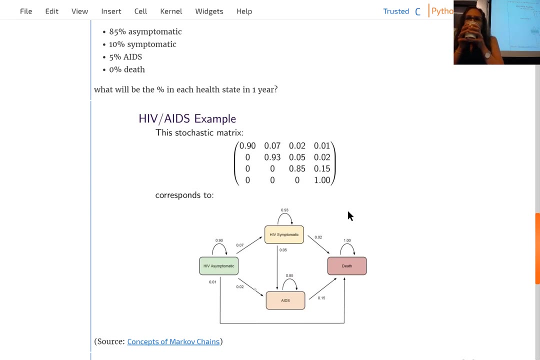 symptomatic and so on. If this matrix kind of is giving you the probabilities of what their health will be like in a year, can you tell me what those probabilities are? So take a few moments to code that, just to warm up. Yes, Although I haven't seen this one in a while. 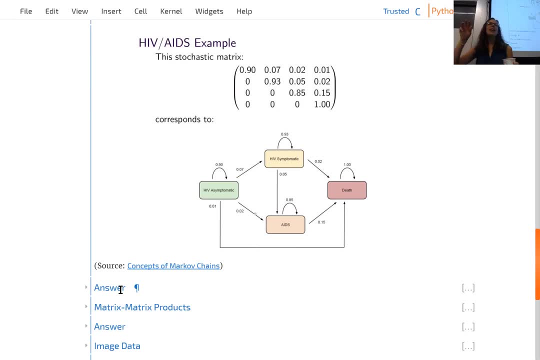 Yeah, Yeah. Yeah, I don't want to. so if you go to the answer tab, it should show up as a cell that says exercise. I'm not opening mine because I have the answer written there. it shows you what the correct answer should be. oh, oh, yes, yeah, it shows you. 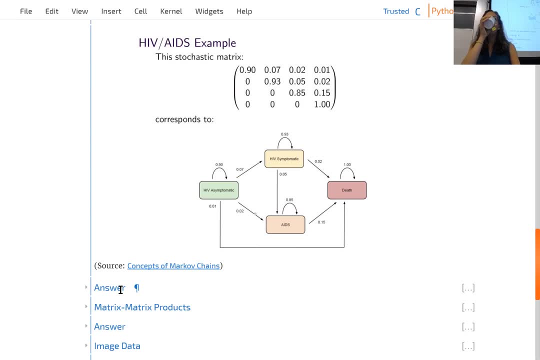 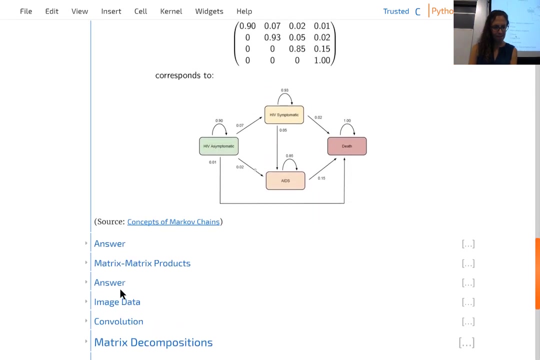 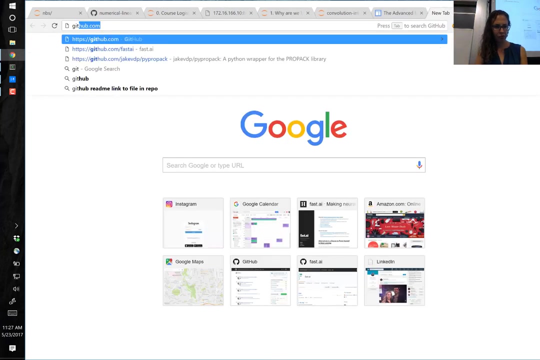 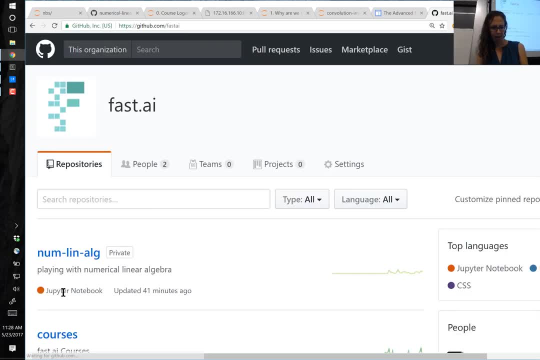 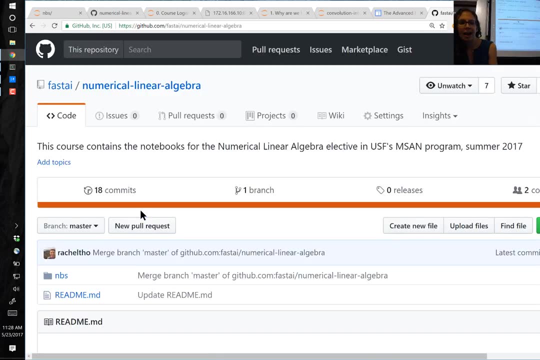 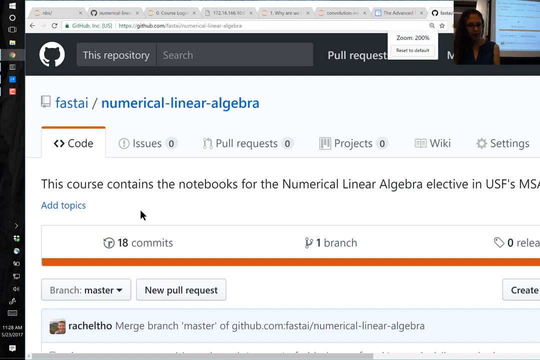 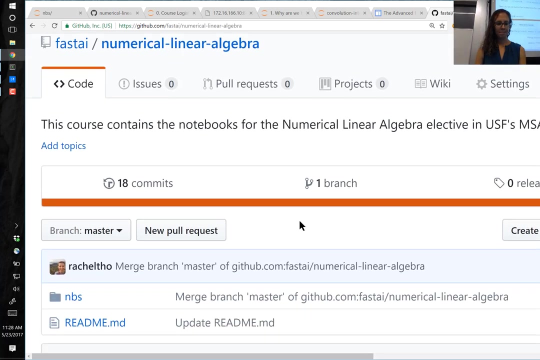 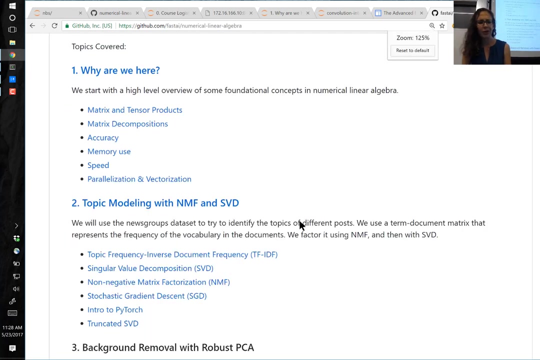 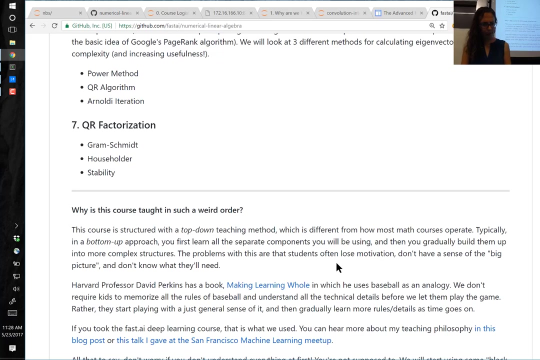 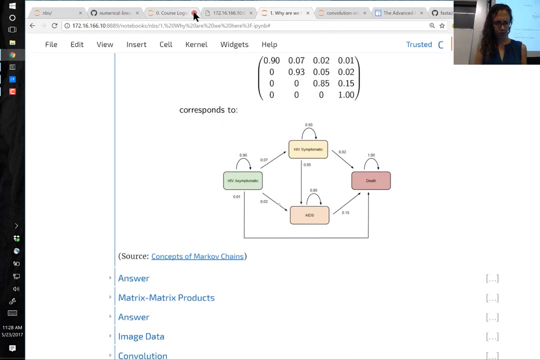 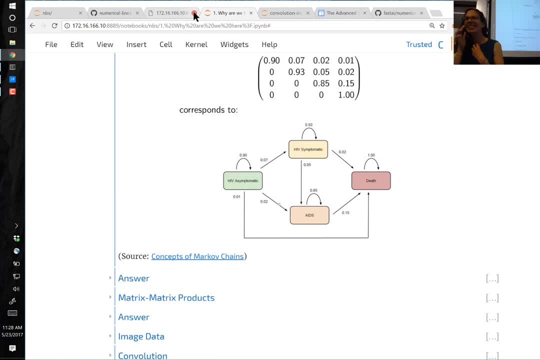 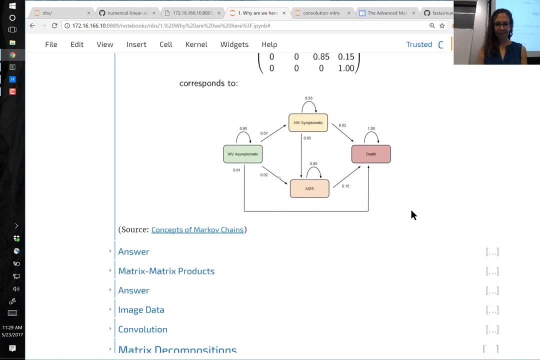 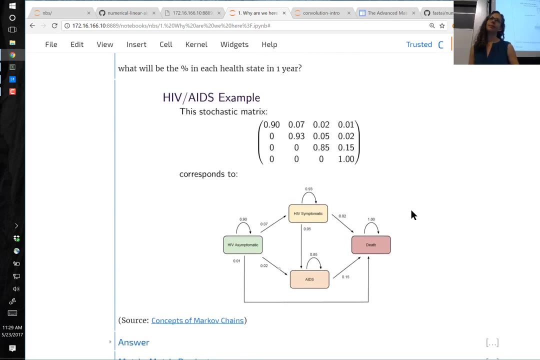 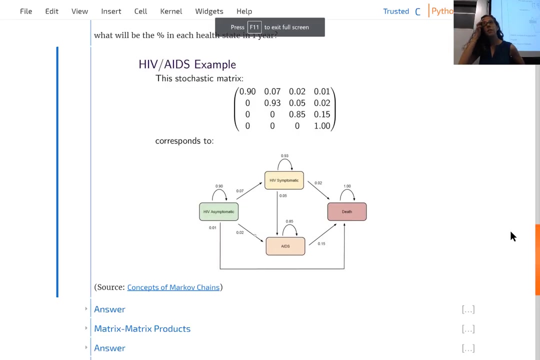 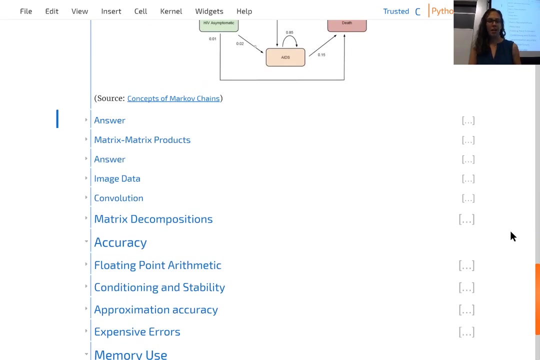 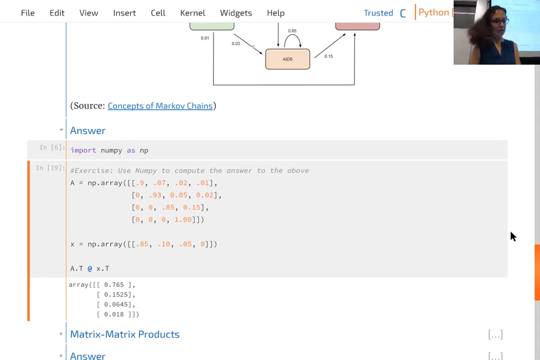 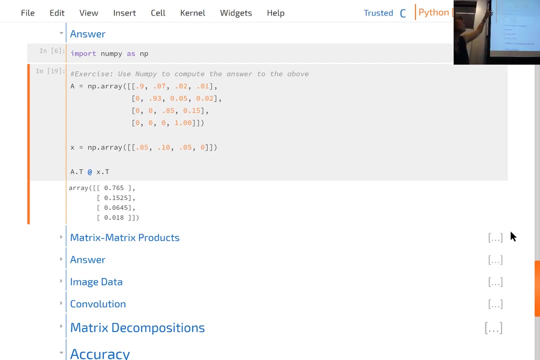 time. oh yeah, that's a great idea. ok, let's, let's look at the answer so you can use numpy to put these in as arrays. so this is a two-dimensional array for the matrix, the vectors. well, actually, I guess I put that as a two-dimensional. 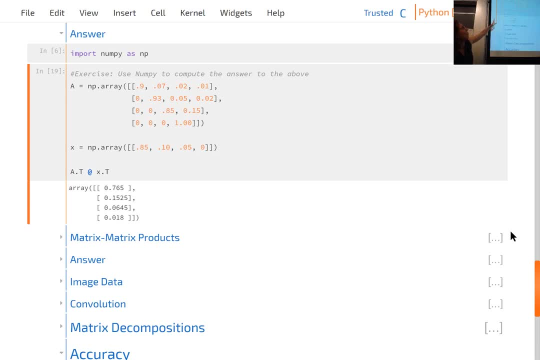 as well. so I did a dot T which is transpose. transpose: the at sign is matrix multiplication in Python 3. I believe you need so for Python 2. you could be using NP dot matmol for matrix multiplication, although I highly recommend switching to Python 3. so does anyone want to say why am I doing a transpose? 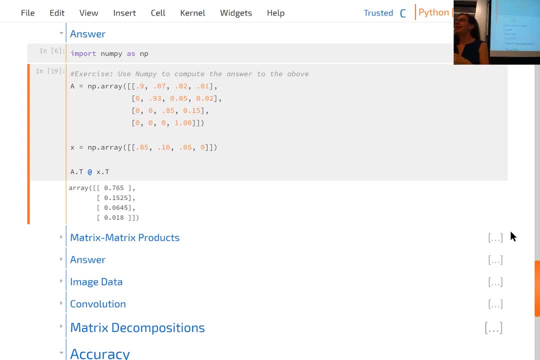 so does anyone want to say why am I doing a transpose? so does anyone want to say why am I doing a transpose? that's a good question. my strands look like they got stumbled. OK, can I get people to make the benches? yeah, actually I don't want to knock over your drink. 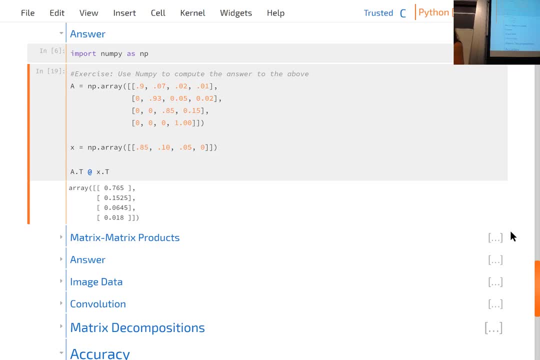 oh, hold it, hold it, OK, ok. this, OK, yeah. so with Markov chains you multiply: on the left as a row vector and on the right a matrix. so you want to get as a column vector in this case. so you just transpose the button, yeah, yeah, and so it doesn't have to come out of everything, right? Иال upавка soprattutto. 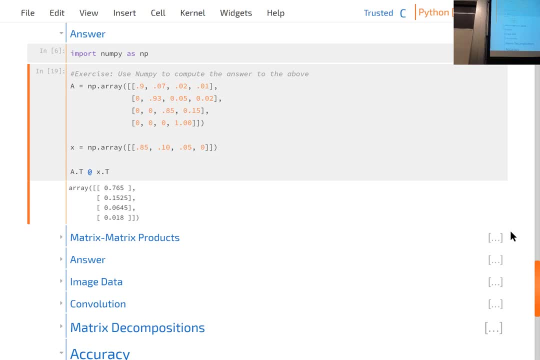 in r, and so it would have been fine if you had multiplied on the left also the other. the other way I think about it is just, by the way, the reason we're using the microphone is so we can hear it on the recording. yeah, yeah, thank you. and the other way to think about this is: 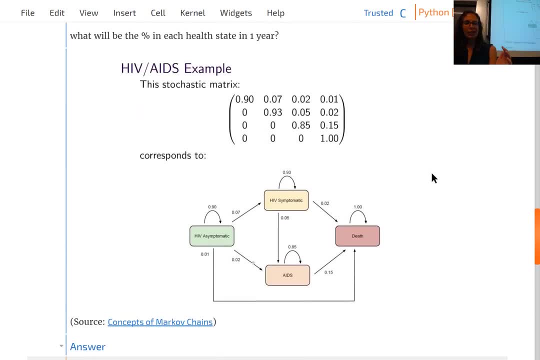 your matrix kind of the dimensions are basically point like sources, by destinations, and so I kind of think of, like, when you do the matrix multiplication, you're wanting to multiply it by the sources, and so I know, if you want the sources over here, you would need the sources to be the columns. 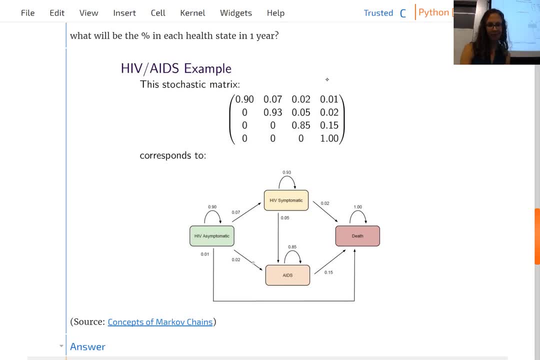 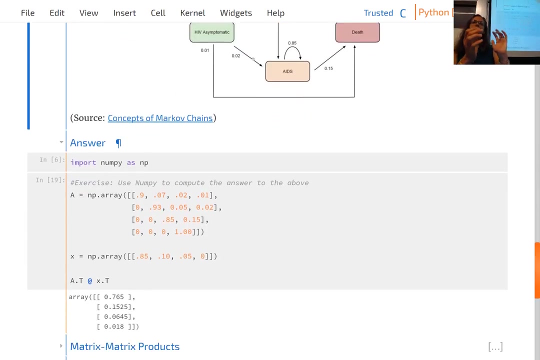 to kind of line up, if you want you know, sources by sources. any questions, Jeremy? I just why I use. I use vector at matrix and it also works. oh well, no, that that would work as well. that's, um, that's actually equivalent. the kind of taking two transposes is: I can write this: 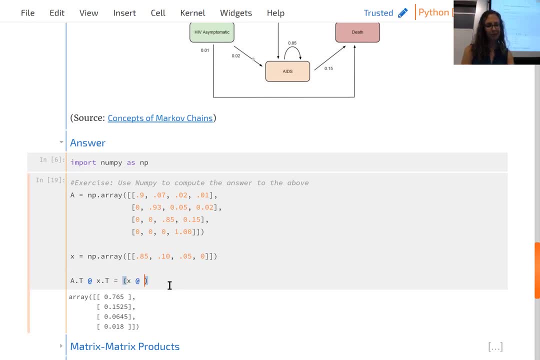 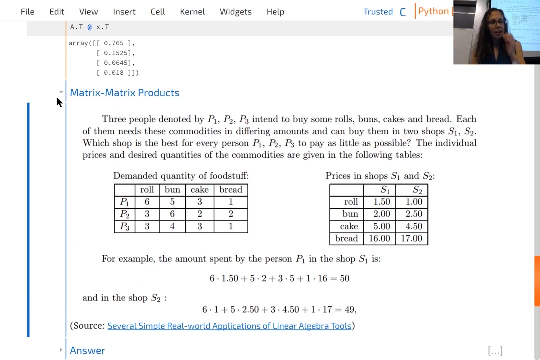 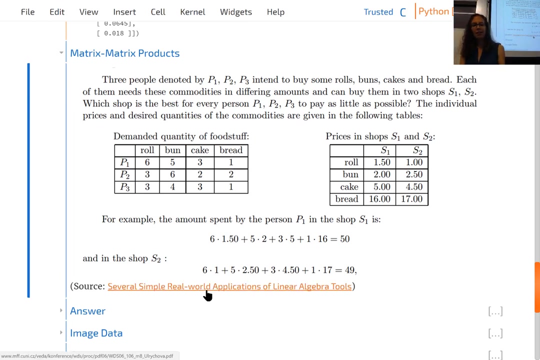 um plaisir. so now gonna take a look at some other stuff like this is equal to like that whole thing transpose. yeah, yeah, it's an app for our matrix, matrix products. this is a problem that I've taken from kind of this, uh, this back shape that has. several different linear algebra problems. this is that well, if you've got transube- yes, you have. transdestueprint has some different kinds of problems that can be more focused. you can use, when you get more, all kinds of answer factors like ah. I would like to use a. 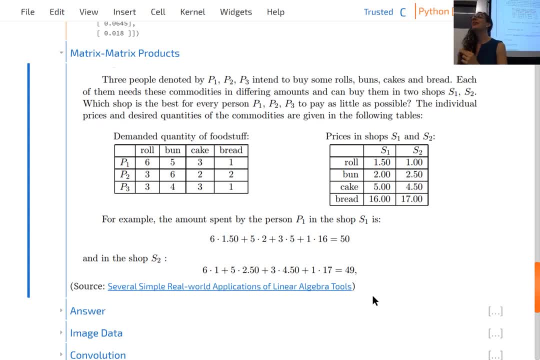 And so here this is, and a lot of them. I think a lot of times when you're doing things by hand, they look like overly simplified examples, But it's important to remember that the power of matrices is that you can do these on really large data sets and large matrices as well. 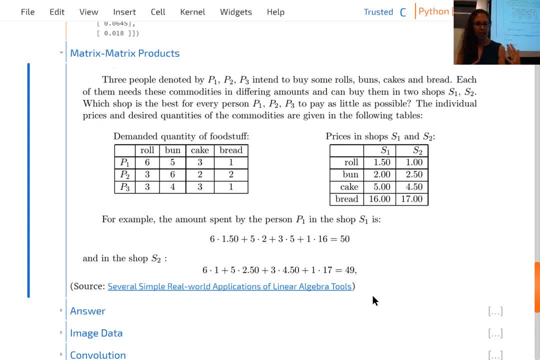 But here you've got three people who want to buy some different groceries And they have different prices for two different shops. Each person only wants to go to one shop, which is the better shop for each person to go to, So take a moment to do that. 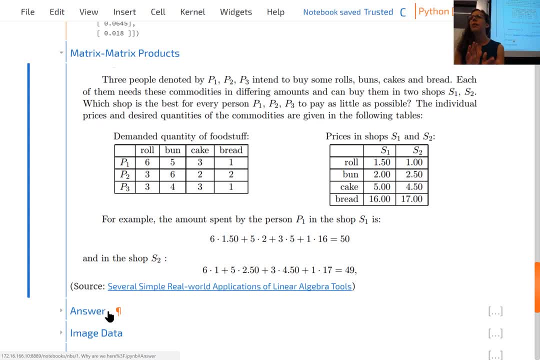 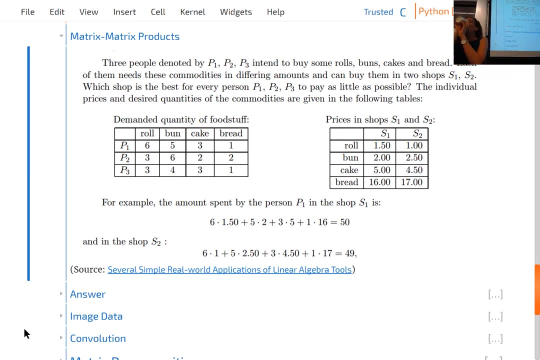 And again, if you go to the answer tab, there'll be a little bit of space and it should show you what the ideal answer is. So, if you go to the answer tab, there'll be a little bit of space and it should show you what the ideal answer is. 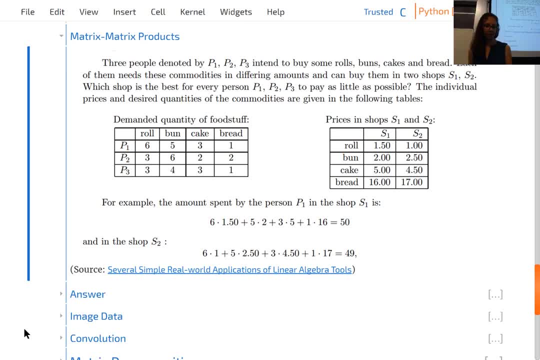 And again, if you go to the answer tab, there'll be a little bit of space and it should show you what the ideal answer is. And again, if you go to the answer tab, there'll be a little bit of space and it should show you what the ideal answer is. 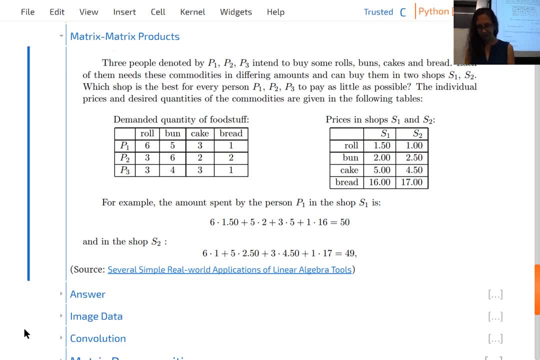 And again, if you go to the answer tab, there'll be a little bit of space and it should show you what the ideal answer is. And again, if you go to the answer tab, there'll be a little bit of space and it should show you what the ideal answer is. 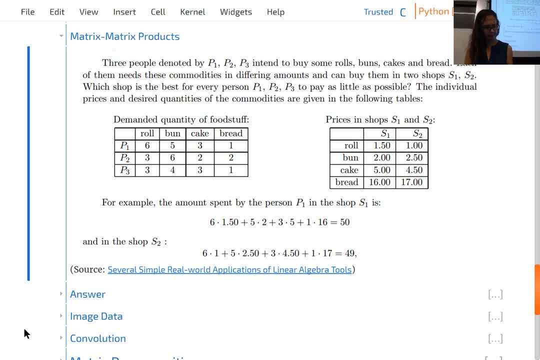 And again, if you go to the answer tab, there'll be a little bit of space and it should show you what the ideal answer is. And again, if you go to the answer tab, there'll be a little bit of space and it should show you what the ideal answer is. 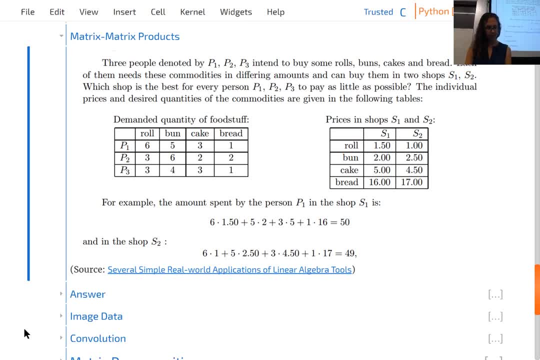 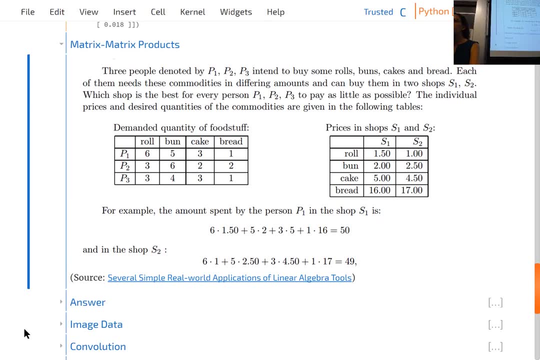 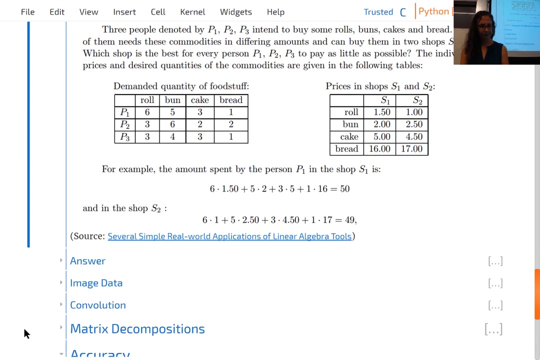 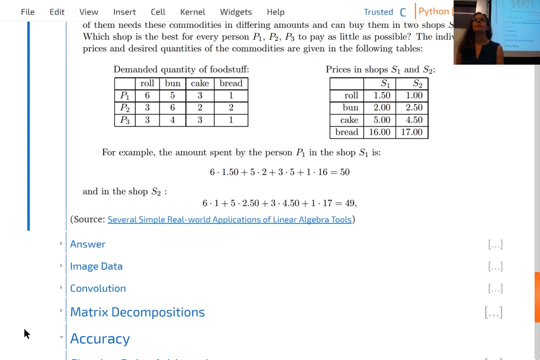 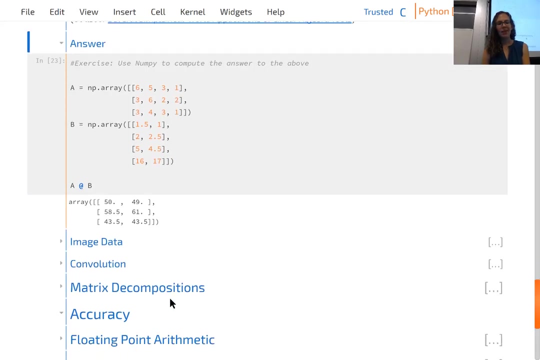 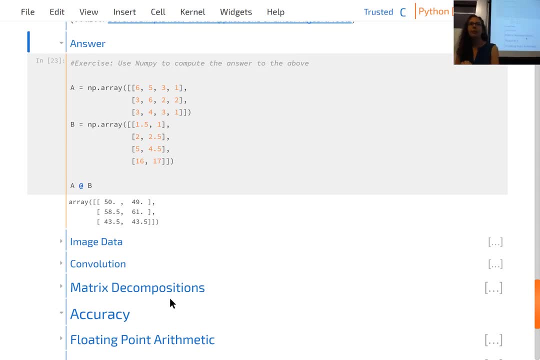 Yeah, So this is kind of pretty straightforward of entering the matrices. Yeah, So this is kind of pretty straightforward of entering the matrices. of entering the matrices C's as numpy arrays and I did A at B or you could do npmatmall if you're in. 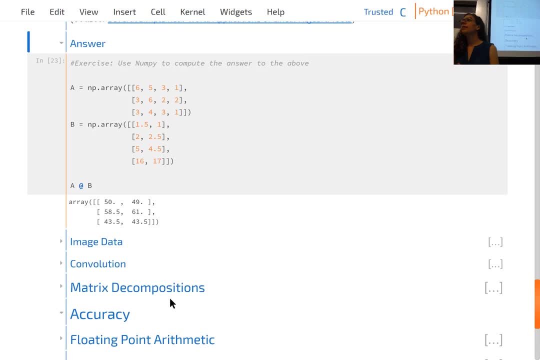 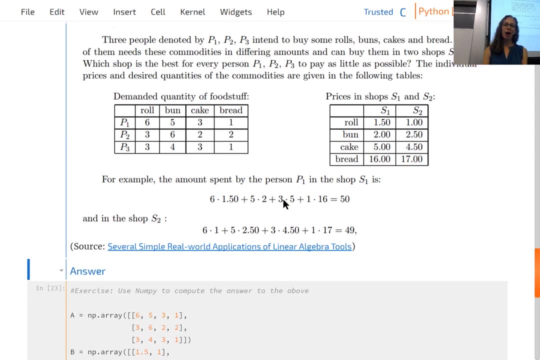 Python 2.. Any questions? And this, if you look at, I think it's even in the part I copied. it's kind of nice how they copied out this example of you know, the amount spent by person 1 is this row and we're multiplying it by this column to get. 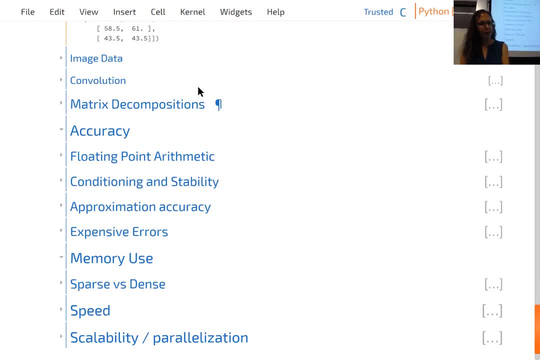 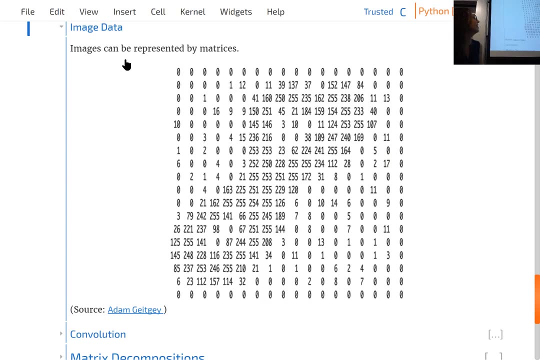 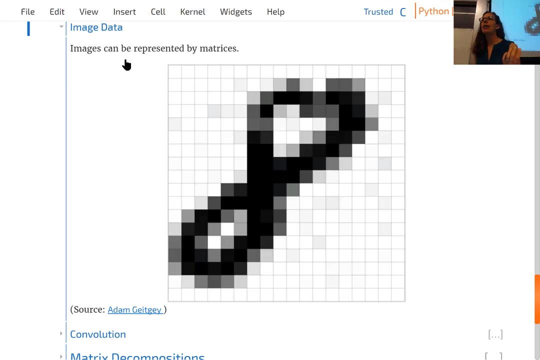 what they would spend in shop 1.. Oh, so next up is image data. So I really like this GIF that illustrates how images can be represented by a matrix of numbers, and so here, this is black and white and the values are between 0 and 255 to show. 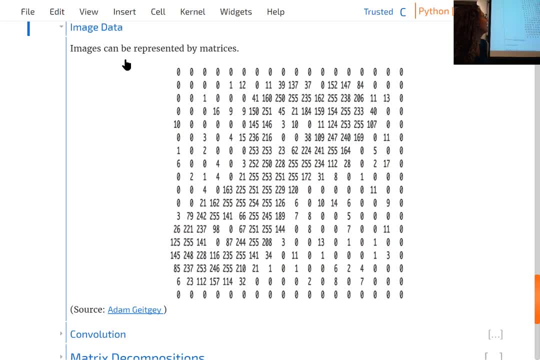 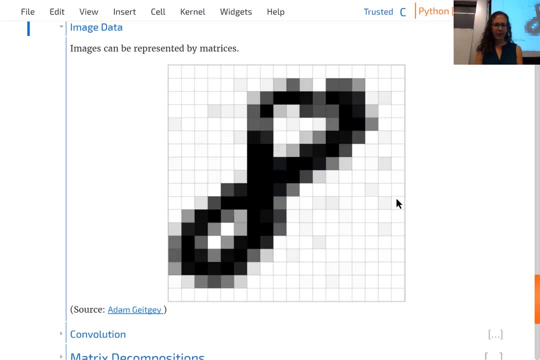 that this is the handwritten digit 8 and it could be represented by a matrix of- I'm not exactly sure if this is like 20, by 20 or so on, And typically, a lot of times what happens is that matrix might be unrolled then into a single row, but now you've got, you know, 400 numbers. 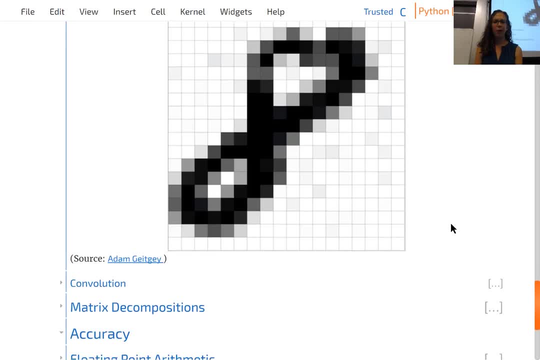 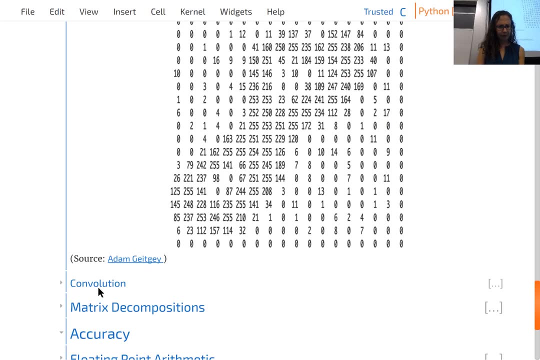 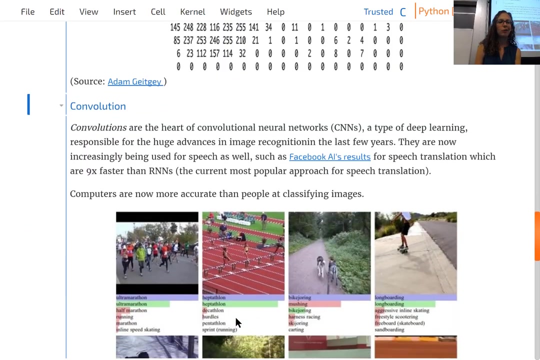 representing what that picture looked like. And for color images, you just have three matrices: one for red, green and blue. Any questions about that? Okay, so we're going to look at color. We're going to look at color. We'll talk about color a little bit more later, and 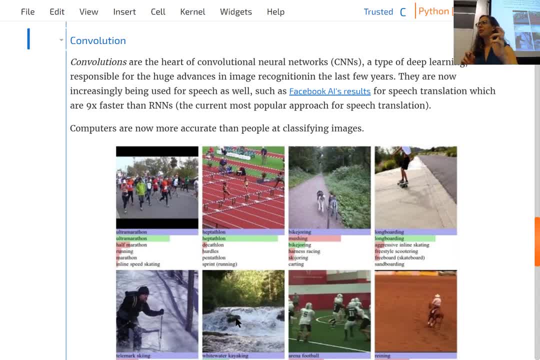 I'm just going to show you a couple of things about color. So let's talk about color. So this is pretty simple, kind of looks like this right here, So you can see that this is the larger color, So you can see the difference between the. 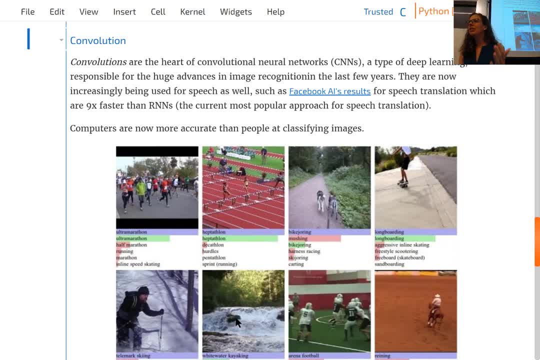 two colors here. So these two colors are the colors we mentioned earlier. So that's sort of the kind of color we're looking at right now, And so, in particular, this is a kind of a simple color function. So this is a kind of a sort of a. 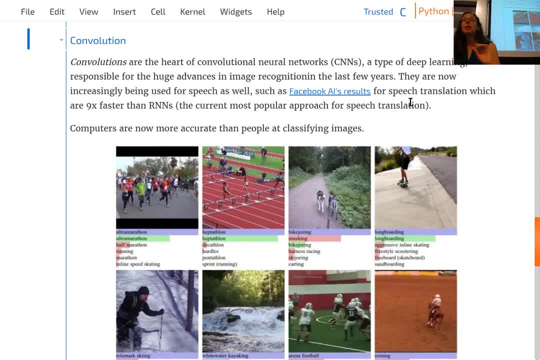 Chinese color function, So this is sort of a kind of a US color function. So this is sort of a Facebook's AI team published results for speech translation, where they use CNNs instead of RNNs, which are kind of typically what people use for language. 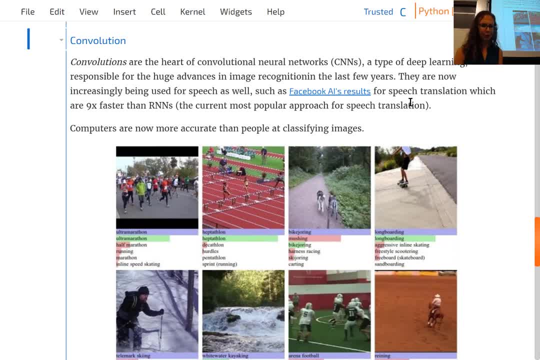 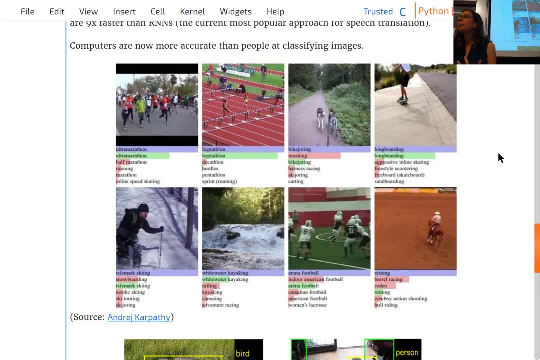 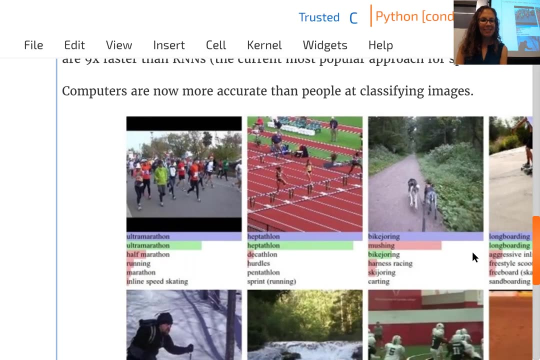 and they were nine times faster. So convolutions are very useful. So using convolutions or convolutional neural networks, computers are more accurate than people at classifying images. I should zoom in on these, So some of these I wouldn't get. 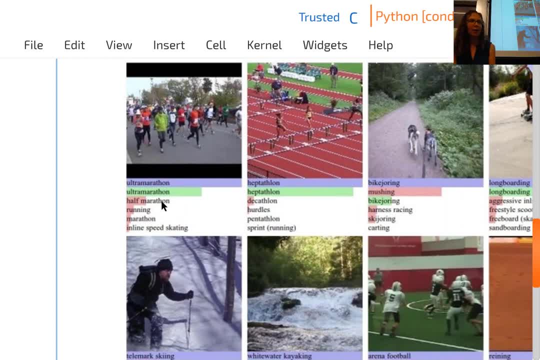 This is an ultramarathon, not a half-marathon. So the computer got that top choice was ultramarathon. Their second guess was half-marathon, Third guess was running and fourth guess was marathon. So a lot of times these are very fine-grained categories. 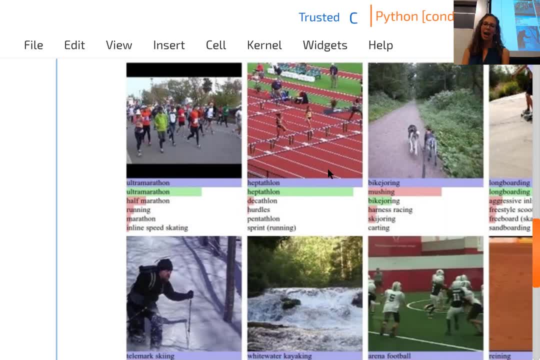 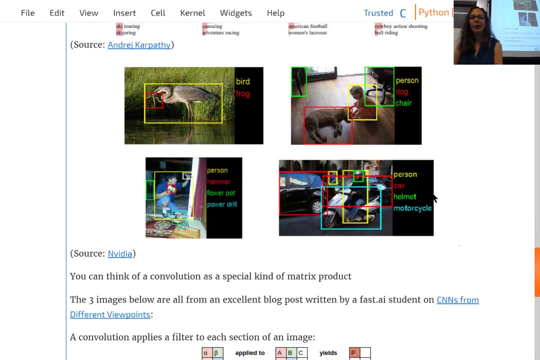 or distinctions, And again, I like this. one of this is a heptathlon, not a decathlon, Hurdles Or a pentathlon, But this is what computers are capable of. And then here's an example of an algorithm to kind of find bounding boxes for different objects. 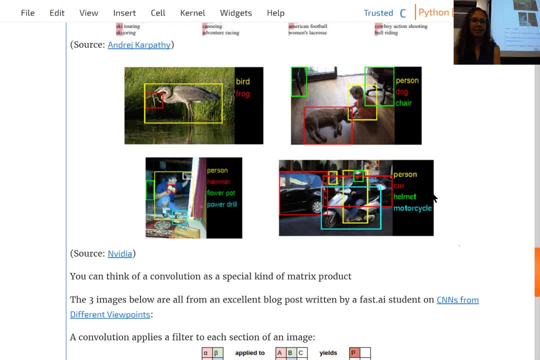 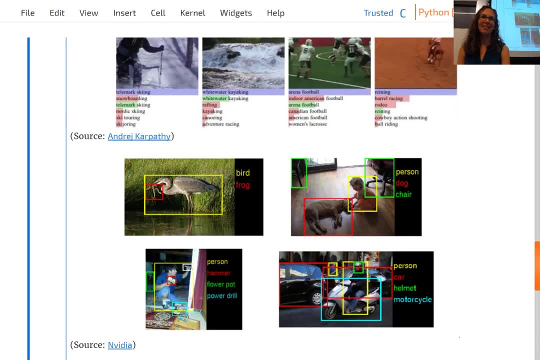 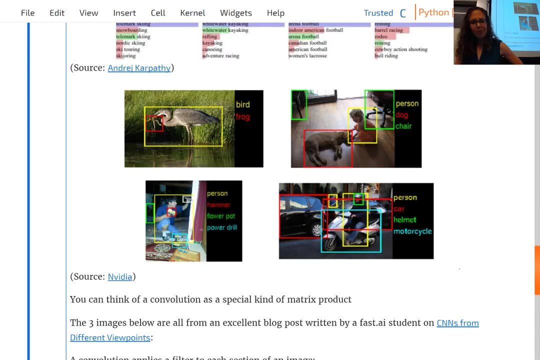 inside a picture and then identify what the object is And you can see: Oh, my goodness, okay, Wow, so that's even more impressive. I think This was done on videos is what Jeremy just said. But yeah, so this one. they've identified two different chairs. 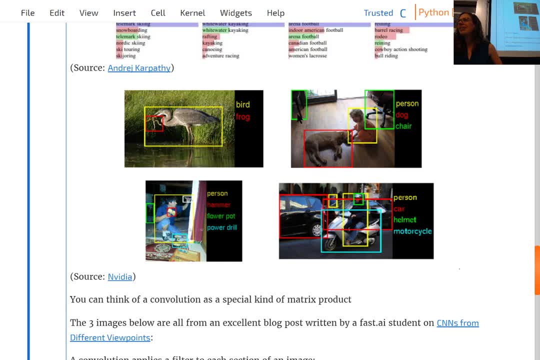 in the picture, you know, including this one which is kind of you're only seeing part of it and it's in the dark, you know, and a person and a dog, And this is pretty intricate. There are a lot of objects overlapping each other. 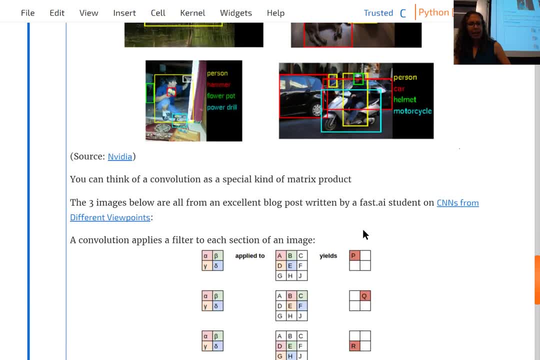 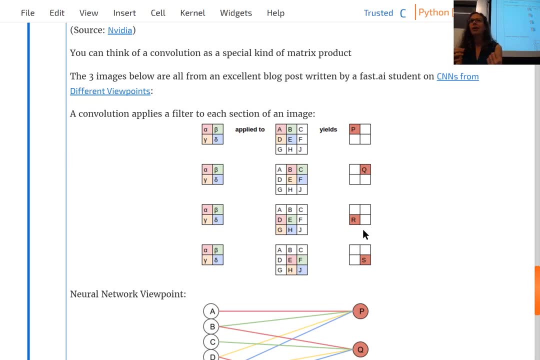 and the algorithms recognizing them, And so we will not be getting into kind of the full details of this, but I wanted to talk a little bit about how convolutions work, since there are, you know, useful building blocks for deep learning and then application of linear algebra. 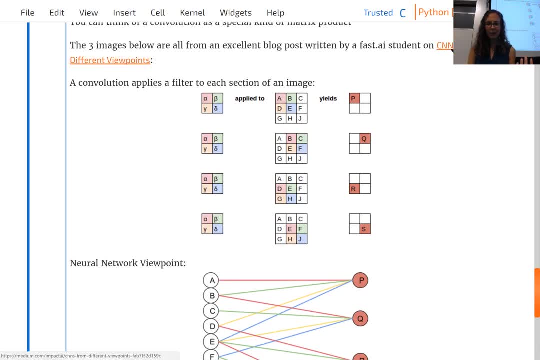 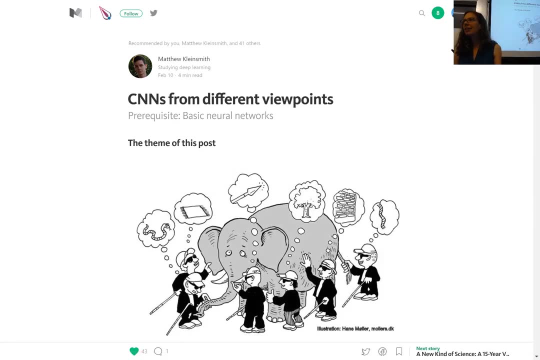 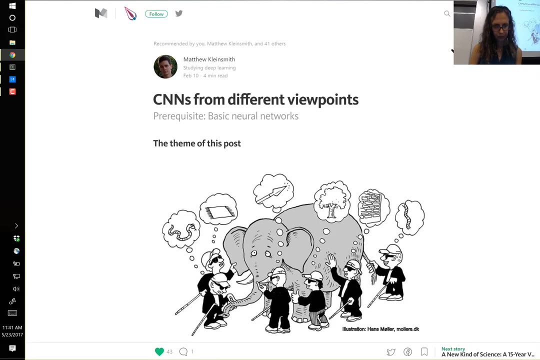 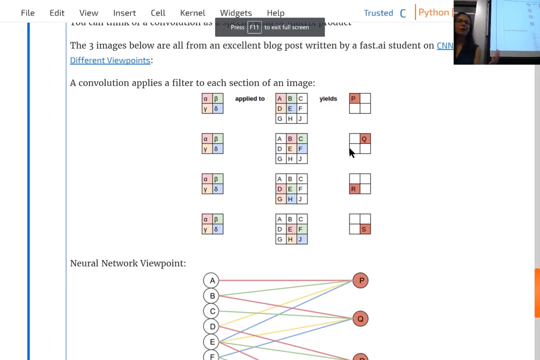 So this is some images from a blog post. Let's see if this opens. Yeah, written by a student in the deep learning class that was here at the Data Institute. Let me go back. Thanks, And the idea behind the convolution is that it applies a filter. 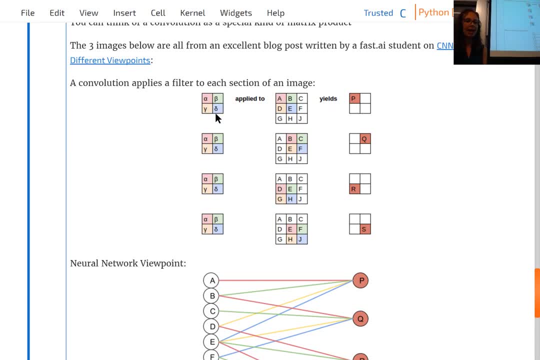 So here we've got a filter that's just four numbers- alpha, beta, gamma and delta- And it's being applied to a picture, perhaps that's just three by three, so pretty small, And you kind of put it in each location. 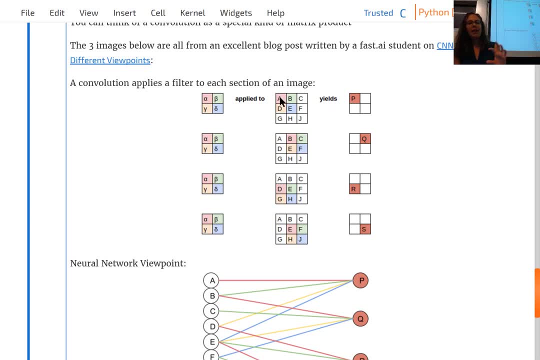 So we put it in the top left corner and then we'll multiply alpha by a, add that to beta, times b, plus d times gamma, plus e times delta, and get a single number. So that's the idea behind the convolution. 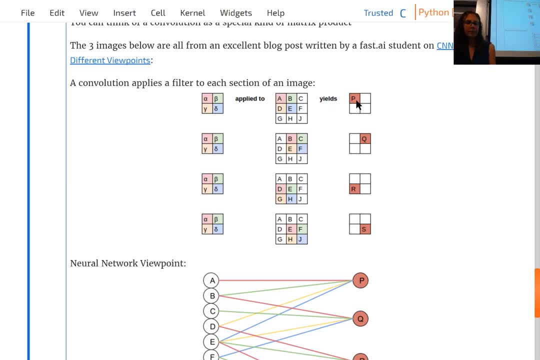 So here we've got a filter that's just four numbers- alpha, beta, gamma and delta- And so we're going to number out p as the result, And then you slide that filter across the picture and do it at each possible space. 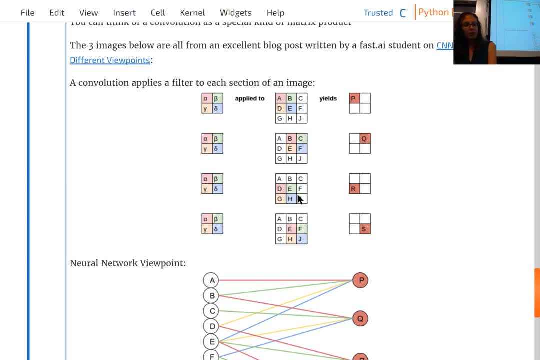 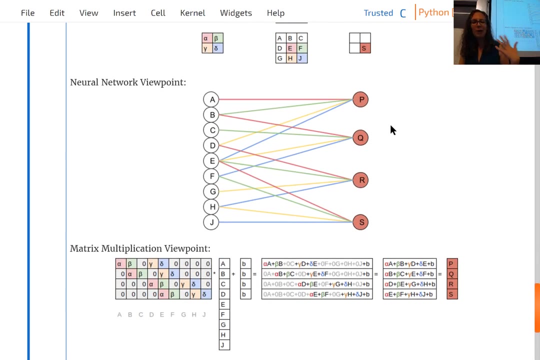 So here it is, in the top right We get out one result: Bottom left, bottom right. So this is just with a single filter on a small picture, And so that's kind of one way to think about how a convolution works. Another is- and I find these pictures less helpful- 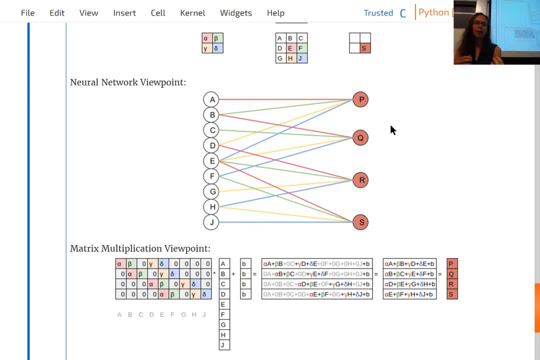 but a lot of people like to draw neural networks from this point. So this is a neural network. Here the alpha, beta, gamma and delta are the connections, And so those would be the weights on the connections. So whenever you see a red line, you know. 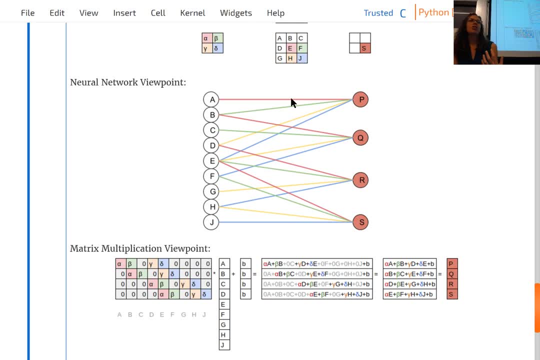 that's saying there's a connection between a and p And the weight of that connection is alpha, And so the same operation is happening that we saw before to get p. p is, you know, got four connections going into it: a times alpha, b times beta, d times alpha. 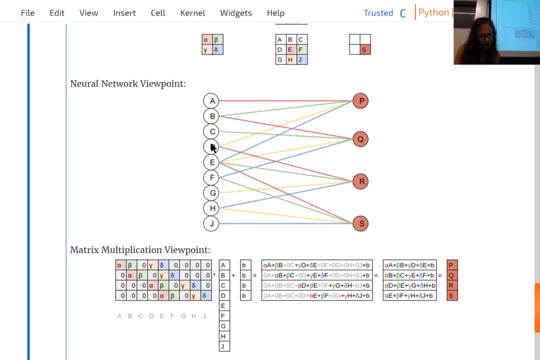 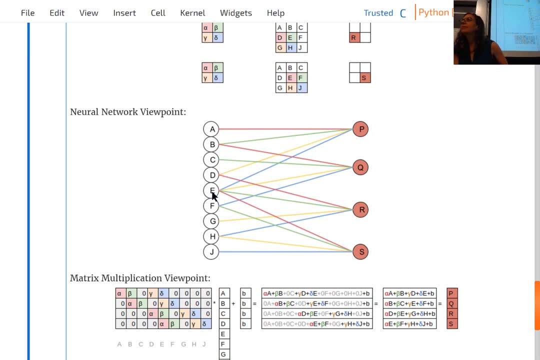 and so on and so forth. So that's kind of the idea behind it. d times, is that right? Yeah, d times gamma, and then what else? e times, delta. That's another perspective And I really like this approach of thinking about topics. 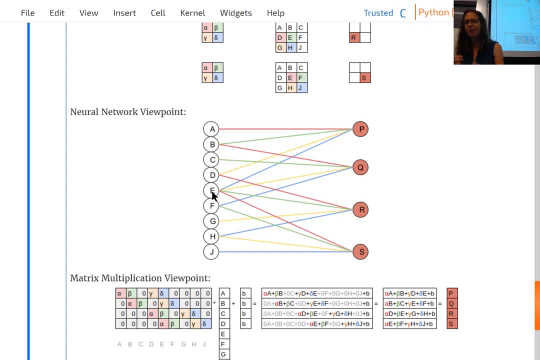 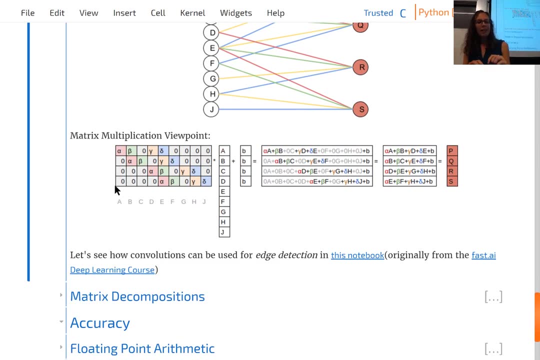 from different perspectives, because I think that kind of help you get a deeper understanding. And then this is neat: Here Matthew has kind of unrolled the filter and put it into this larger sponsor. There's two filters: matrix and shown. hey, this is actually a matrix multiplication. so now our kind of 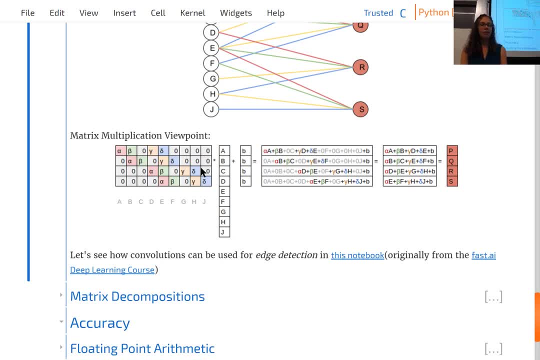 ABCDE from our picture is just a single vector and we've got this sparse matrix and that just sparse means it has a lot of zeros and those actually show up a lot, kind of matrices that have lots of zeros in a specific structure, like this one does with the diagonals, and you can do a matrix multiplication and get the. 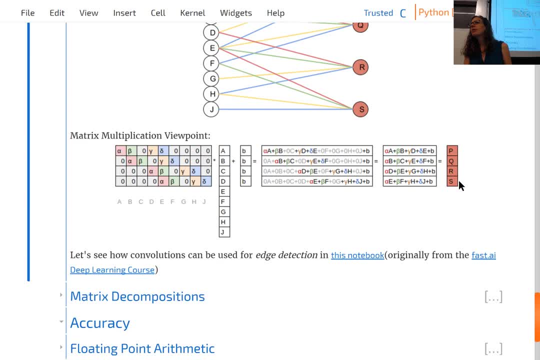 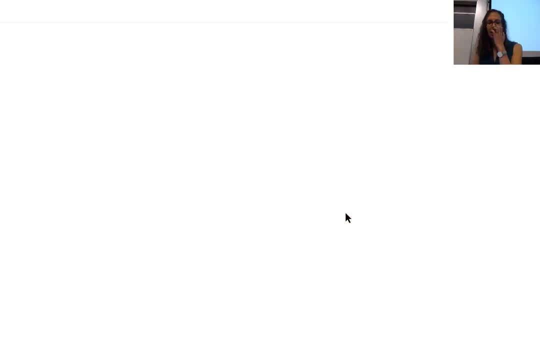 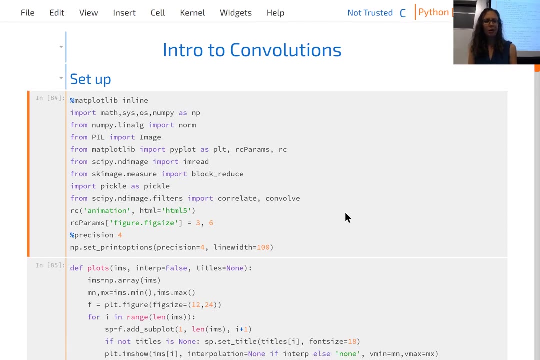 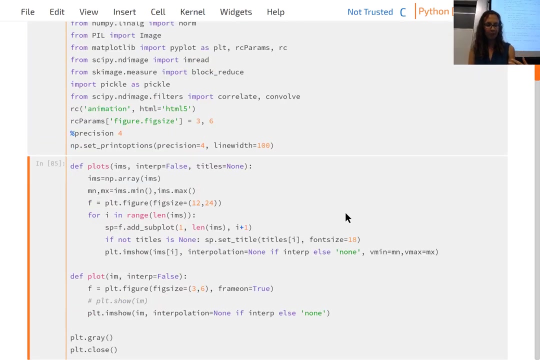 same result, any questions? okay, so now we're going to look at and how we could use this for edge detection in this notebook and this. don't worry. don't worry too much about the setup, but these are kind of the files you need to our libraries you need to import. yes, 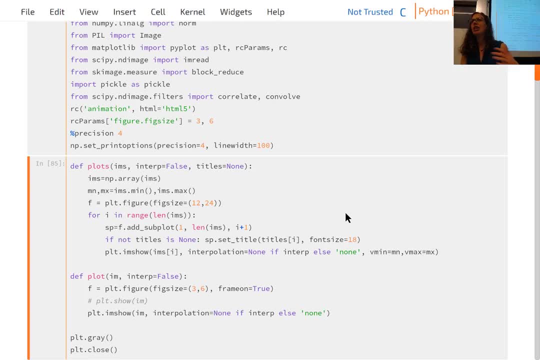 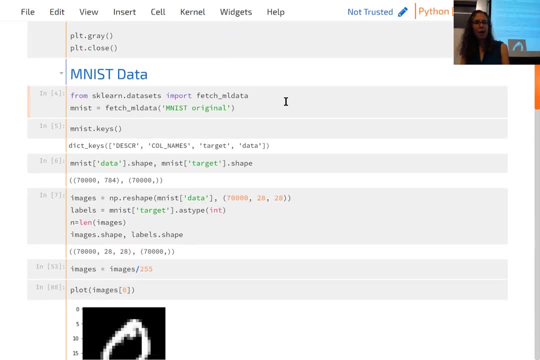 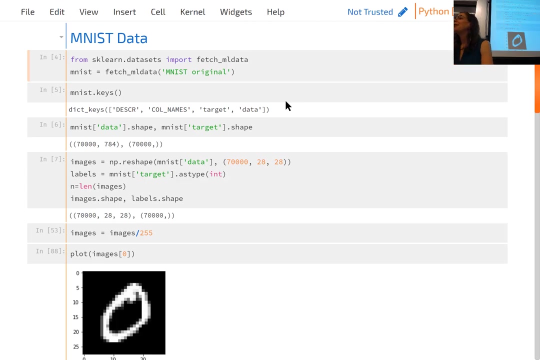 oh, thank you. this is convolution intro and this was originally part of the deep learning course, so we'll be looking at MNIST data, which is, you know, this really popular data set of lots of handwritten digits. this is very useful for banks being able to automatically identify, you know, when you insert your check into the. 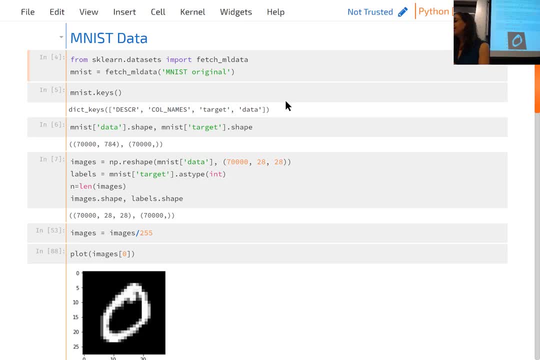 ATM what the numbers on it are. post offices automatically sort our mail by zip code using image recognition on the digits. you know when you insert your check into the ATM what the numbers on it are. post offices automatically sort our mail by zip code using image recognition on the digits. 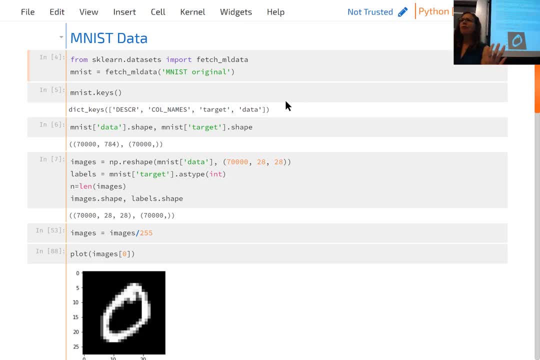 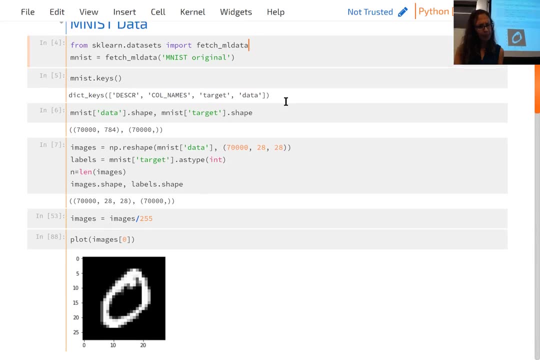 and then I should say scikit-learn has a lot of built-in data sets which are a really useful feature and we'll be using several of them in this course. yeah, so we kind of import and here we're. so for the larger data sets that scikit-learn 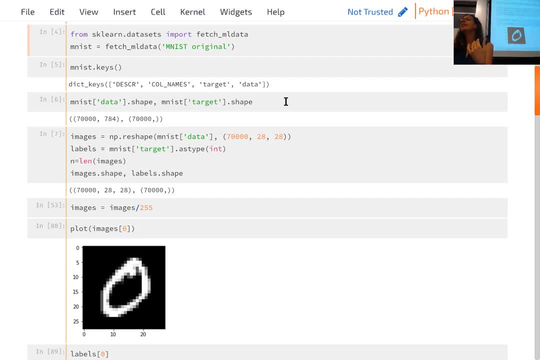 includes. it doesn't include the data set. it includes a data loading utility that you can run to get the actual data. so you run that you can kind of check what the keys are of what you get when you get the actual data. so we run that you can kind of check what the keys are of what you. 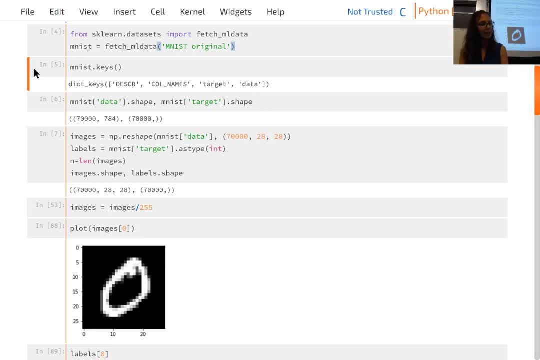 get back, because you're kind of getting back this dictionary like object. we're interested in the data and the target, and targets going to be kind of the label of saying this is what the digit is, the data itself, and then something else. that's always great to do whenever you're kind of starting. anything is just 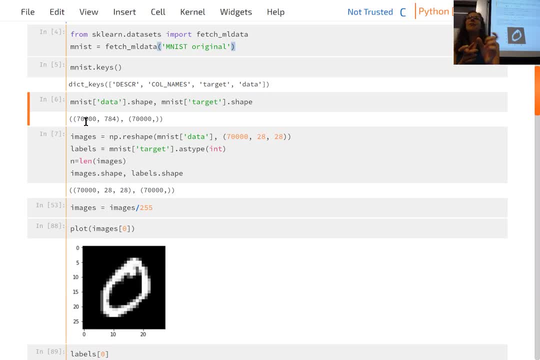 check your dimensions to see if they are what you expect, and you can often also kind of find stuff about the meaning based on the dimensions. so here this is a 28 by 28 if it was put back together. so each row is just a single digit, that's. 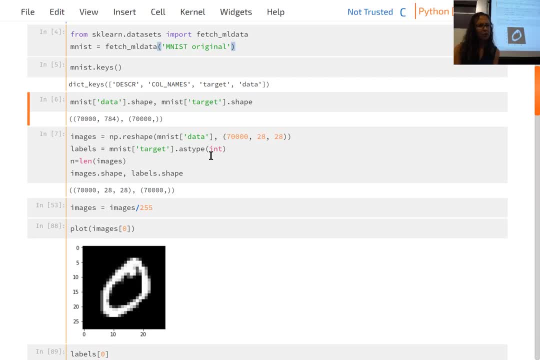 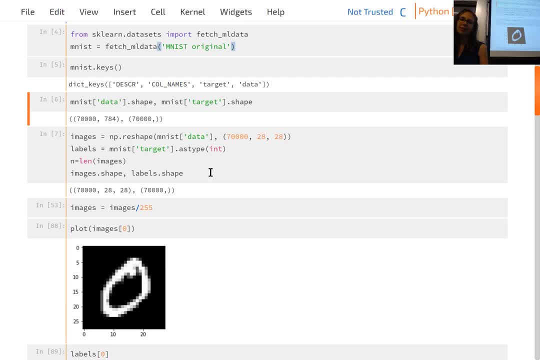 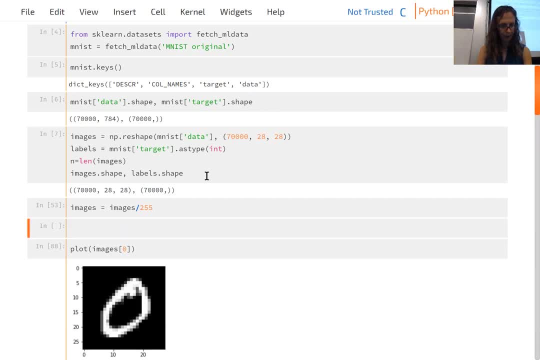 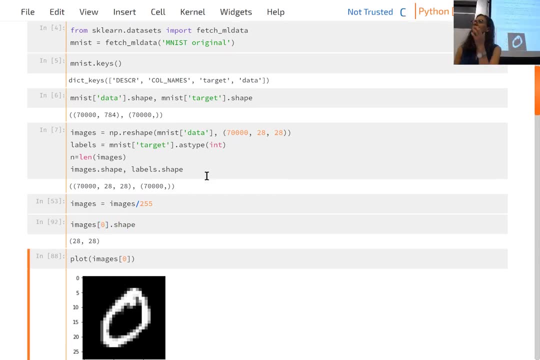 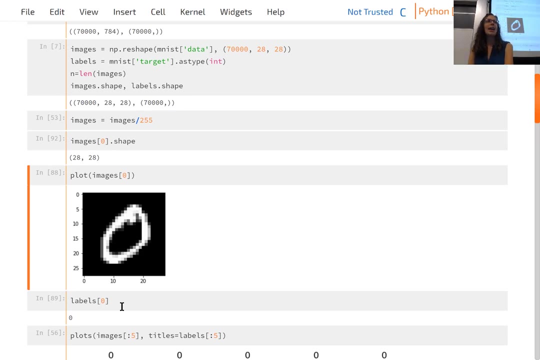 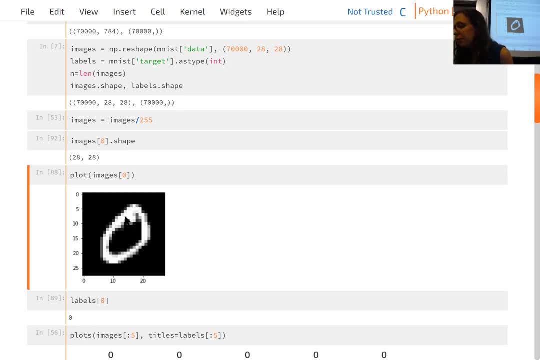 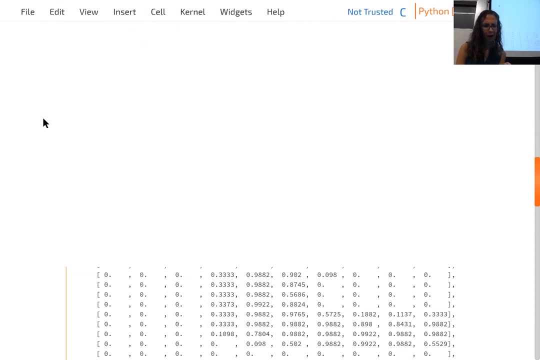 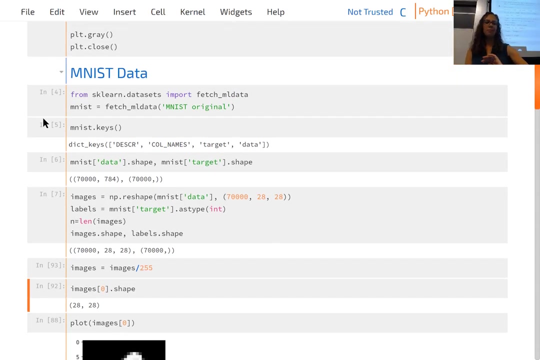 question. oh okay, yeah, the question was: why are we dividing by 255 in, I guess, input 53, which I should probably run again, and in this you, you wouldn't have to and it would still plot properly. this comes up later when, when we're using correlate, I believe. but yeah, if you plot it, if you, so we're trying to turn. 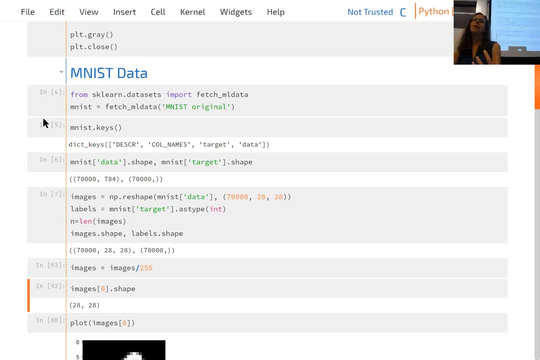 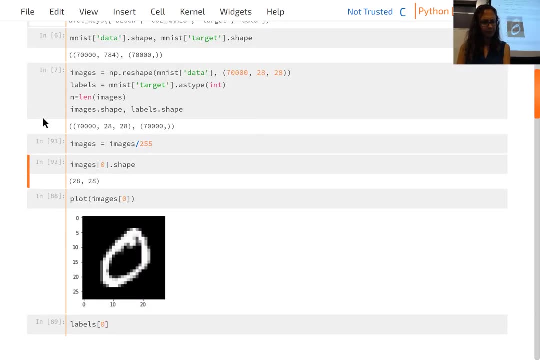 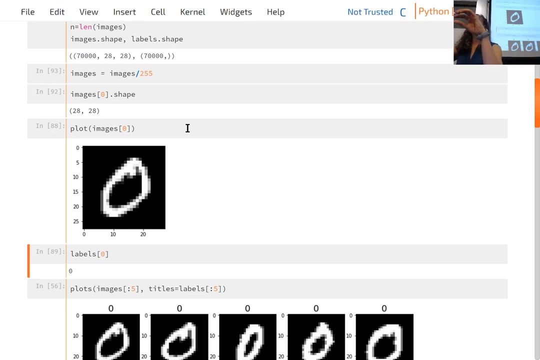 these into numbers between zero and one. it would still work if you had them between zero and 255, so kind of just a way of normalizing. or, I'm sorry, I should say the plots would still work. it would still be you when you plot it. you'd be like: this is clearly. 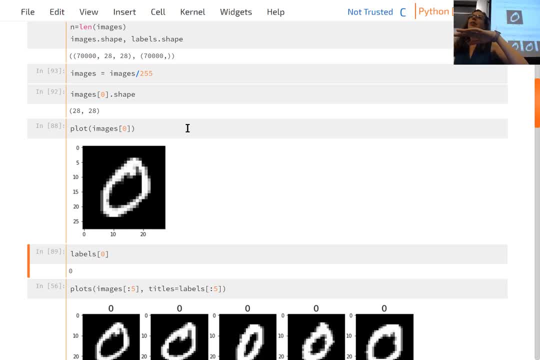 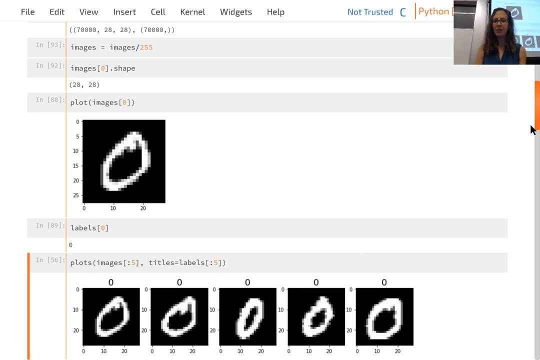 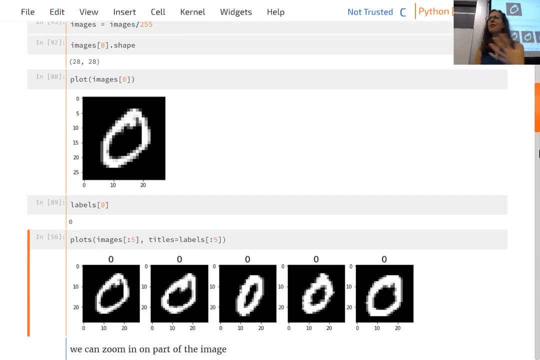 the same image some of the computations we're going to use later. we needed it to be normalized, for here. we also have a plots helper function, and so these were the methods that were kind of defined up here, although I don't worry too much about the details of them unless you're particularly interested. we're using and: 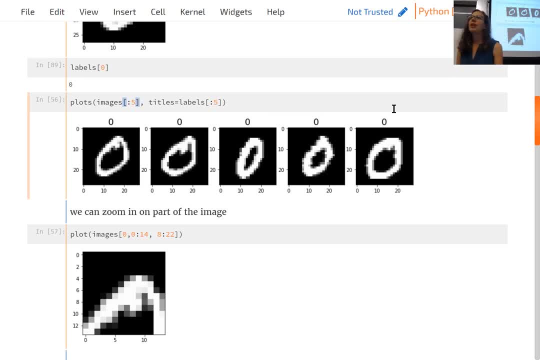 it lets us put in a whole array of images and plots them like this, which is really handy for being able to look at our data, and this is also something I would recommend. I think sometimes it can feel kind of finicky writing the helper methods to be able to look at your data. 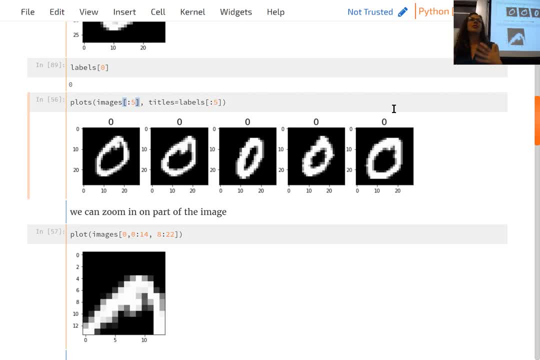 but it's pretty much always worth it because as you're doing computations, you want to check that things are what you think they are and be able to see what your results are. we can also zoom in on our images, so if you want to see just a, 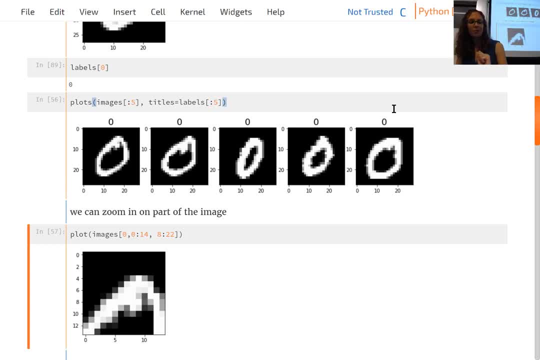 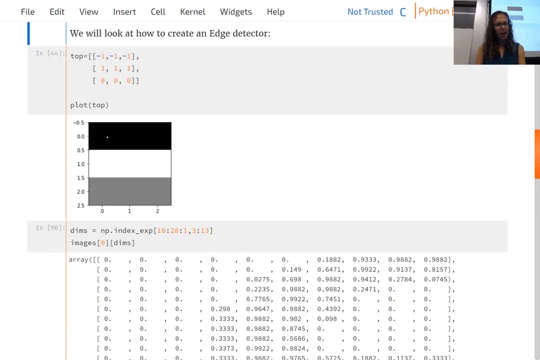 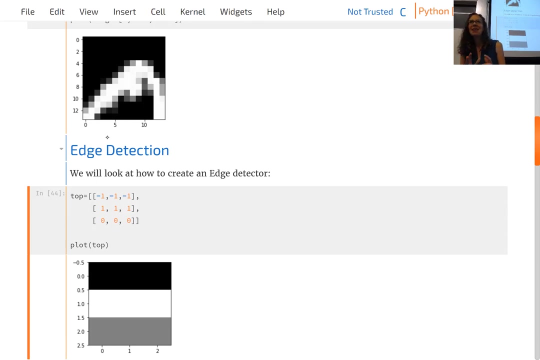 plot of part of one. here we're just getting the rows from 0 to 14, columns from 8 to 22, so this is kind of the middle top of the zero. is what this, this thing is from this picture right? so for edge detection we're gonna have a matrix with the name, that kind of. 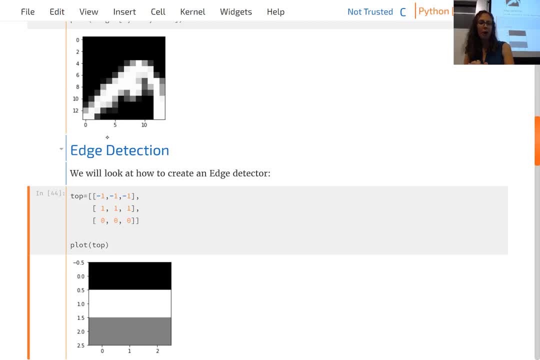 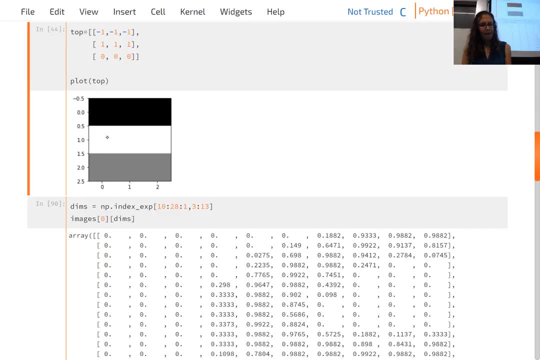 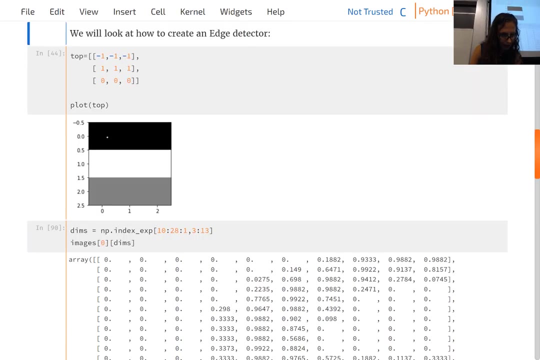 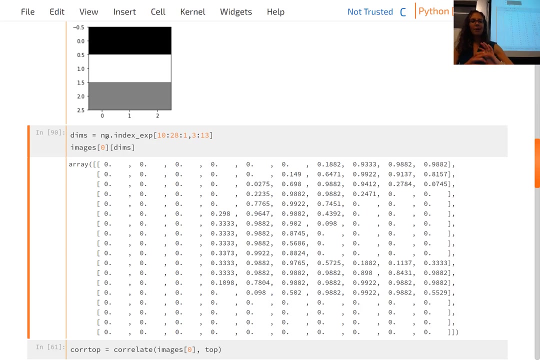 gives a lot away called top, that's negative ones along the top row, ones along the middle row and then zeros along the bottom, and this is what top looks like, and so something to keep in mind and actually out here. this is an interesting perspective and this could have been in higher up. using numpy, we can 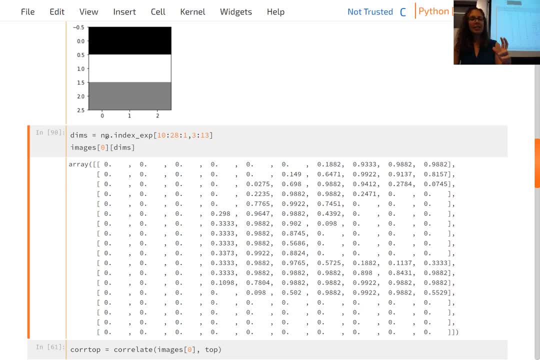 look at kind of just a part of the, the matrix, and see this is so. it's not plot plotted, but this is what the matrix looks like and here the zeros are black and these numbers between 0 and 1 are giving the intensity of the white part. 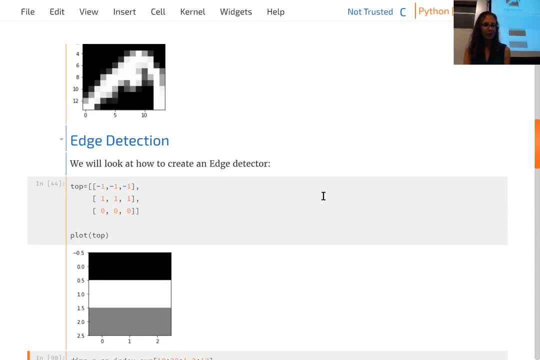 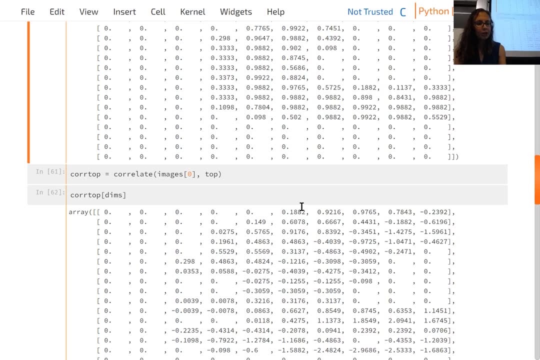 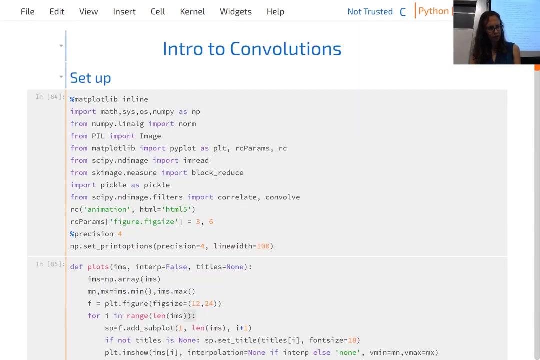 for the handwritten zero. so we're still still kind of looking at this just from different perspectives, and so we're using method called correlate, and this came from its scikit-learns image. there it is sorry. scipy's nd image filters provides a correlate correlate method. 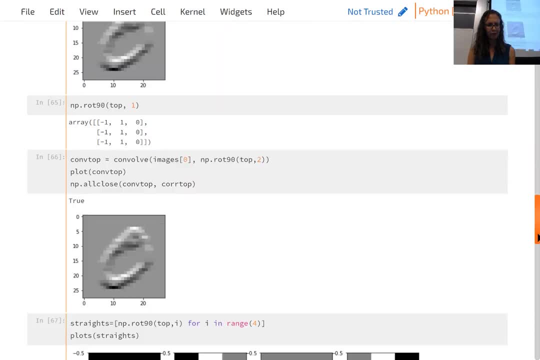 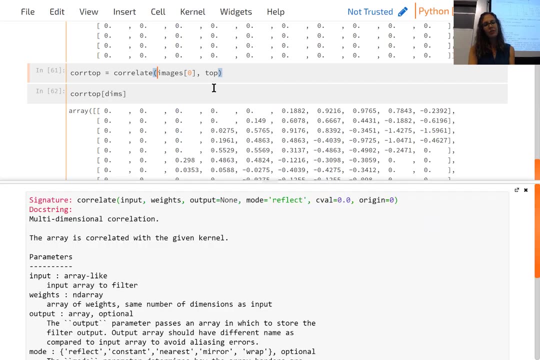 And then something you can do that's a nice feature of Jupyter Notebook is, if you're inside the parentheses for a method, if you hit shift tab a few times, it pulls up the method signature and documentation, which is nice to see, And so this gives an array correlated with a given kernel. 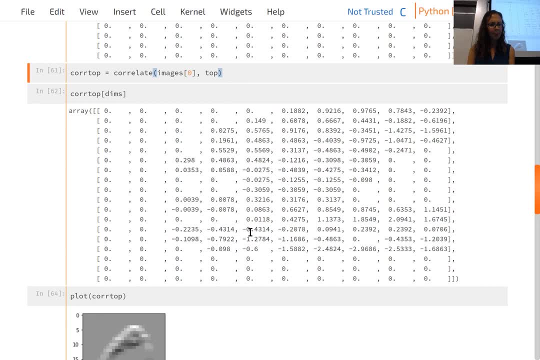 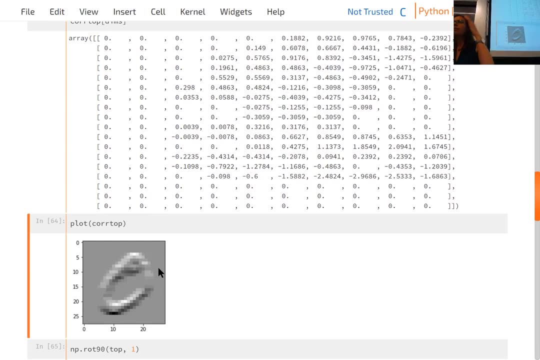 And so here we pass in images zero and top, And if we plot that, this is what we get, And so you'll kind of notice that they're white, which is the highest value along the tops of the zero, and black, kind of the lowest values along the bottoms of the edges. 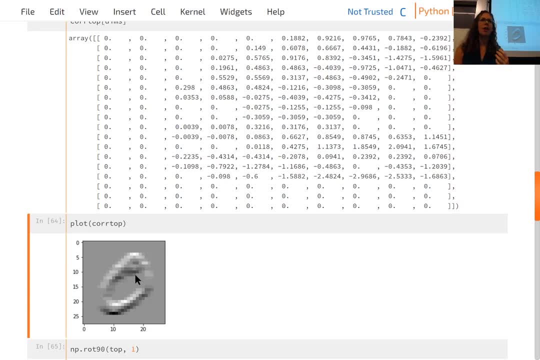 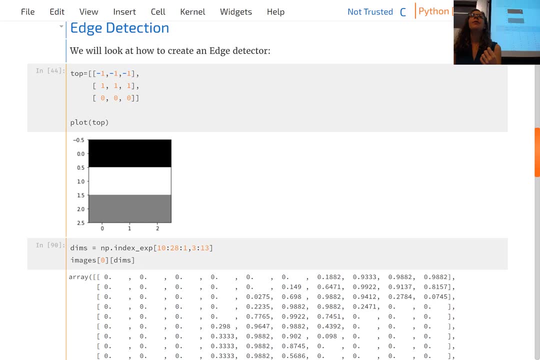 So this has picked off the edges. I'm going to talk about kind of what's going on there with this negative one, one and zero, A way to think about that that's going to be greatest When the negative ones are multiplying by zeros and getting canceled out. if we were trying to think about how could we maximize, you know, top multiplied by something else? 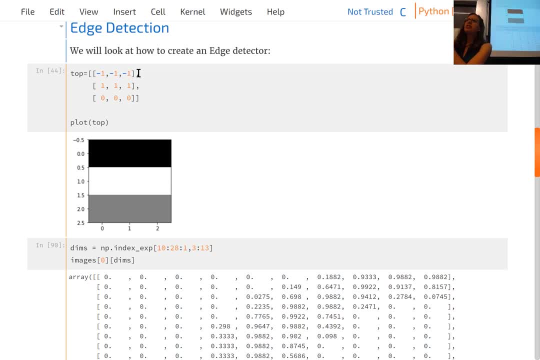 And this is, I should be clear- this is element-wise multiplication we're doing So. this is not a matrix product, but we're element-wise kind of, you know, putting the filter on top of something and then multiplying each element on what it's kind of on top of. 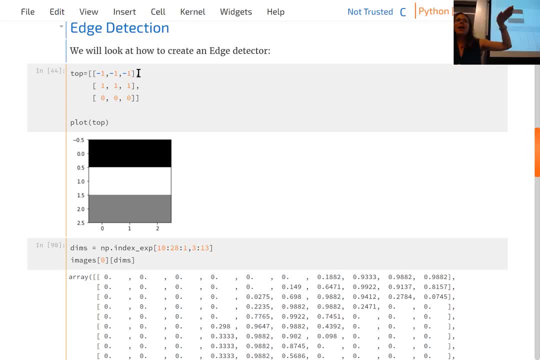 And so having zeros in a full row And then having, like, the highest value, since this is normalized, which would be ones in another row, that would give the biggest value for this, And so that's why it's picking out tops, because it's whenever you go from something small to something large, this correlation will have the highest values. 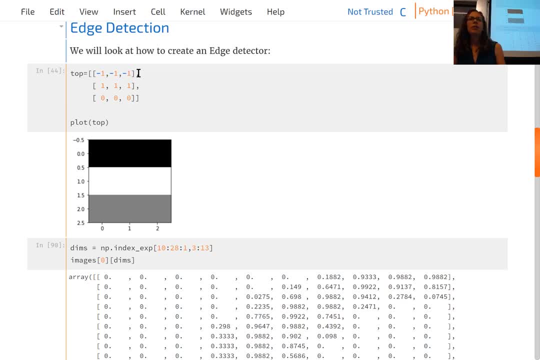 Any questions? I yes, yeah, okay. Jeremy asked the question about convolution versus, or suggested that I talk about convolution versus correlation. The key difference is just: with convolutions they're actually flipped And so this is kind of a mathematical accounting thing. 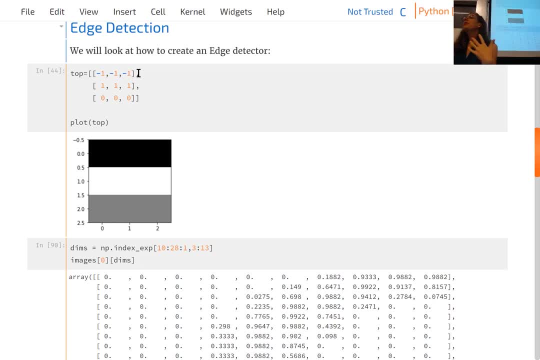 Right, Like there's not a yeah, That it's yeah, So it's really it's the same, and kind of in the math you take into account like oh okay, this has actually been rotated when you're doing a convolution. 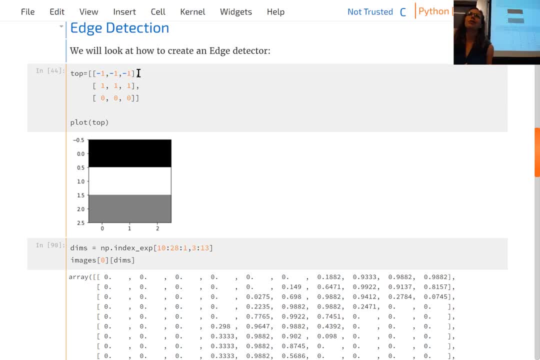 But it's the same idea as a correlation, And I think correlations are easier to think about. Otherwise you're just kind of flipping everything, but getting the same result. Yes, Oh, and let me give you the. So the question is that when you say correlation, are you talking about correlation between columns or between rows, or what type of? 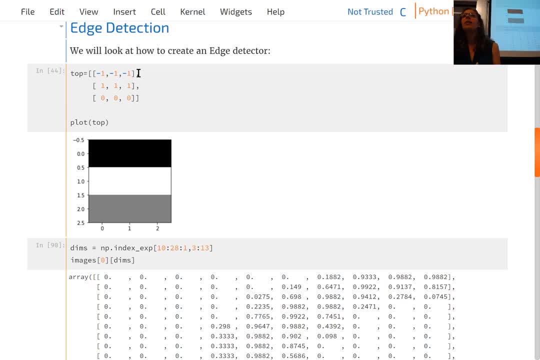 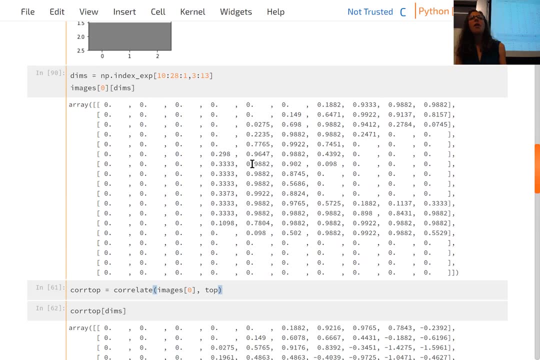 So this is actually element-wise, Element-wise, So you correlate one element. I think it's the confusion of the statistical. Oh, yes, Yeah, So this is. this is different from a correlation matrix that you hear about of in statistics. 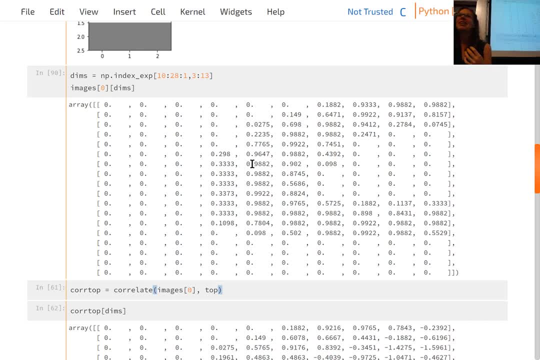 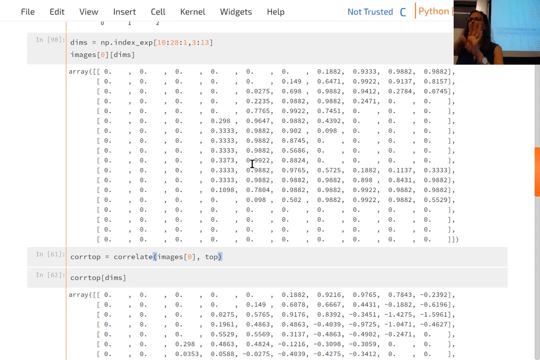 Yeah, So kind of overuse of the word correlation. Yeah, this is a different use. In deep learning, when they say convolution, they normally do this, So I think it was the same maybe. Yeah, But yeah, but think about that kind of in a separate bucket from the statistics idea of correlation between between different variables. 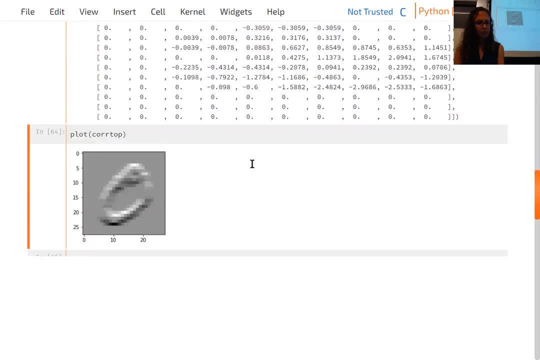 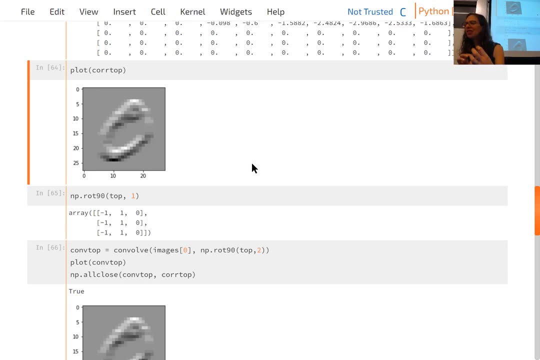 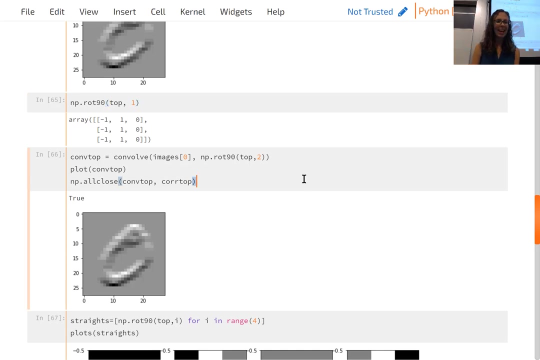 Yeah, So that was really kind of the key idea of how a matrix can be used for edge detection. Here we'll see if we rotate. So remember top was that three by three matrix, We can rotate it by 90 degrees. Oh, okay. 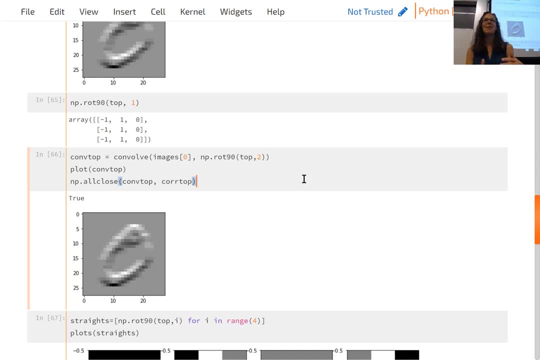 So now it's identical because we've rotated it, So it still does the same thing. I would. I would not worry too much about this distinction. The key thing here is just the idea of you can pick up edges by sliding a filter. 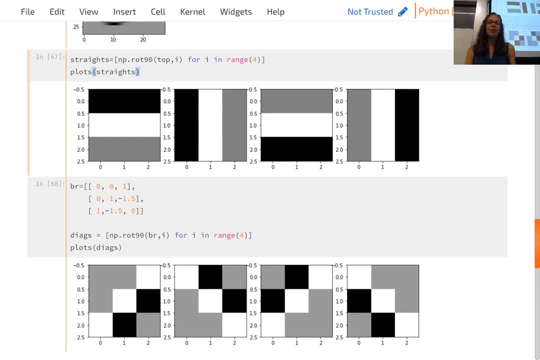 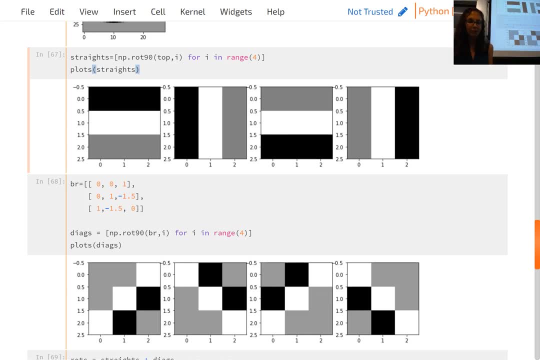 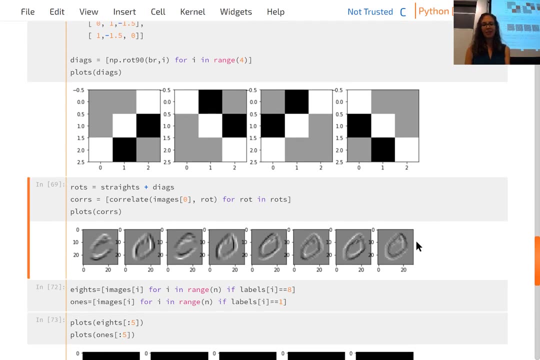 And then this is kind of nice: We rotate a number of times, kind of to get these different ones, And this will give us edge detection for bottom, top, left and right. You can also do diagonals, And so if we apply that kind of all these different filters to the picture of the Z, 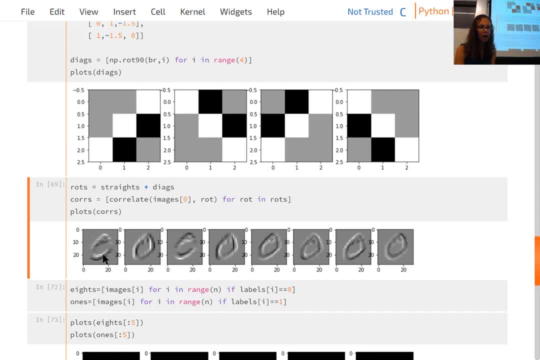 here. you see, we've picked off the top. This one's picked off the left-hand side, since that's where the white marks are Picking off the bottom right-hand side. This is picking off kind of the diagonals towards the bottom right corner. 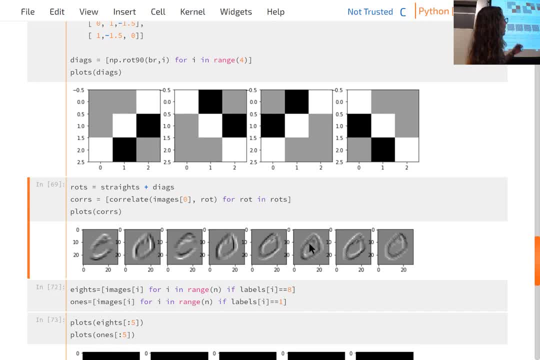 White here is kind of on the diagonals. I mean, you can almost think of it as like a light shining from the top right corner in this line Here, from the top right corner, From the top left, And then I guess this one is bottom left, although the edges are not as defined. 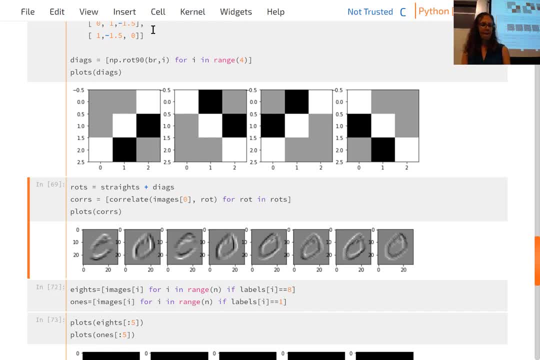 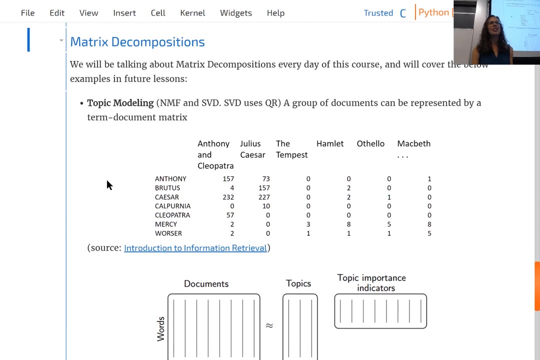 Okay, Any questions on this? Thanks, All right, so that's it for putting matrices together. I mean, we'll be using matrix products every day, but kind of in the intro applications. And now I'm just going to very briefly say some of the matrix decompositions we'll be seeing. 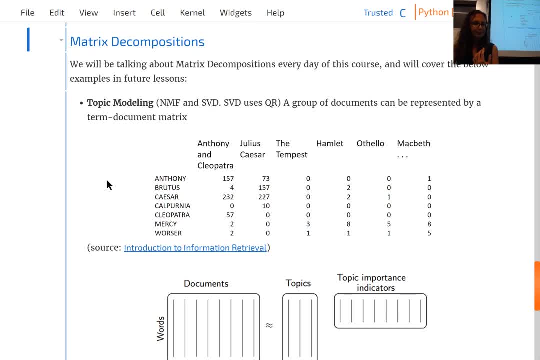 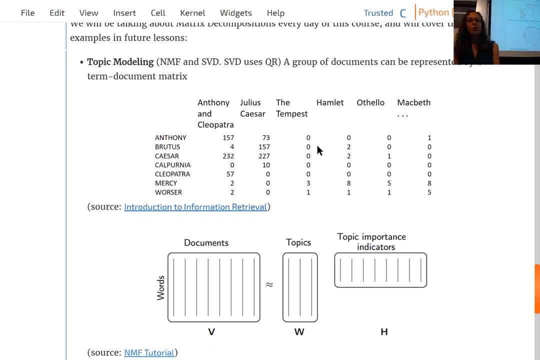 We'll be covering all of these in a lot of depth in the future lessons. So one is topic modeling, and we'll see it with NMF and SVD, And so a group of documents can be represented by a term document matrix. Here these are works of Shakespeare. 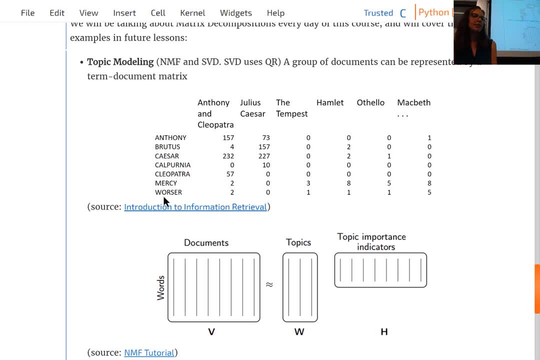 Along the top is the particular play. On the left is different words that appear in those plays And so you can see Anthony and Cleopatra. the word Anthony appears 157 times. In Julius Caesar the word Anthony appears 73 times. 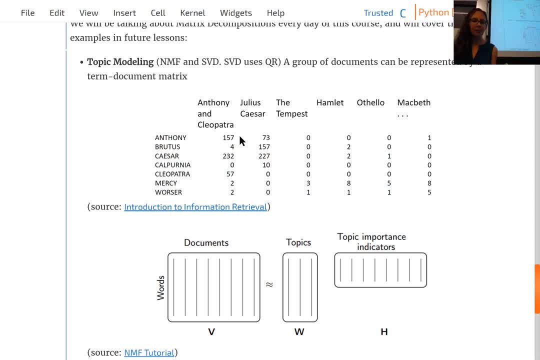 And this is a way that you can represent a group of documents as a matrix, And this is notice that nothing about syntax or order or structure is being included. This is treating them as a basis. This is a bag of words, basically. 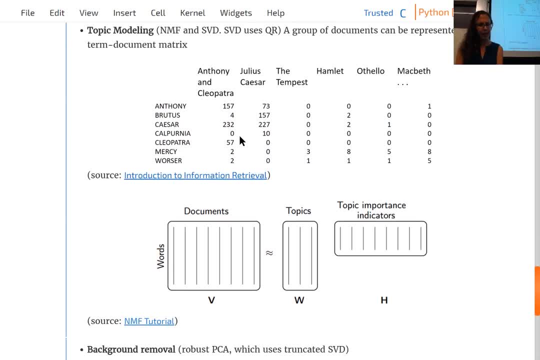 But it can let you figure out different topics And in matrices what that looks like. so this is for NMF. So the words are the rows, the documents are the columns And you can decompose that into a matrix of topics. so that would be topics by words. 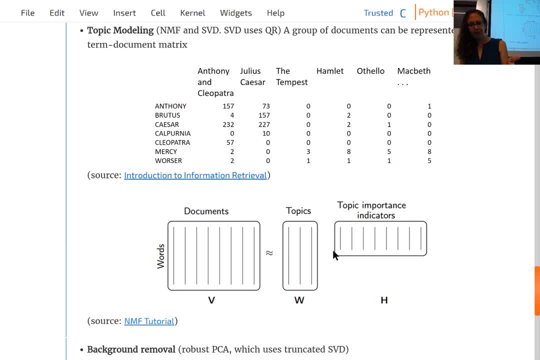 and then topics: importance indicators kind of by topics- Or I mean Really that's the kind of documents- by how important each topic is for that document, And I think it's always helpful to kind of write out what your dimensions are when thinking. 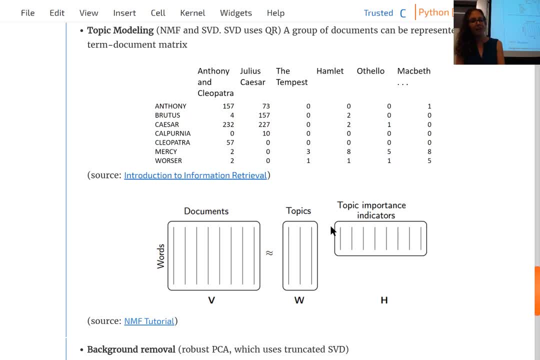 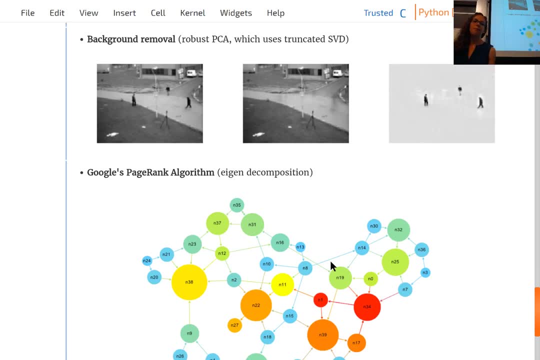 about it. But here topics is kind of going to be your short dimension that you're finding. We'll see background removal, which we'll use, robust PCA, which uses SVD, and SVD uses QR, So there's kind of some nesting going on. 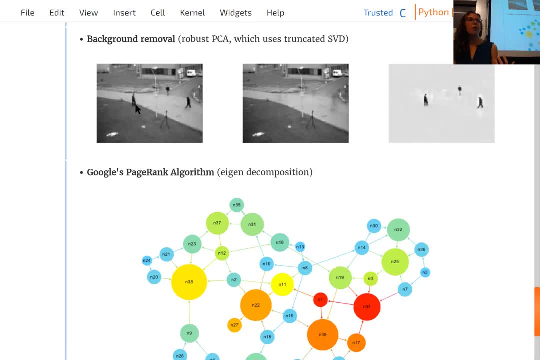 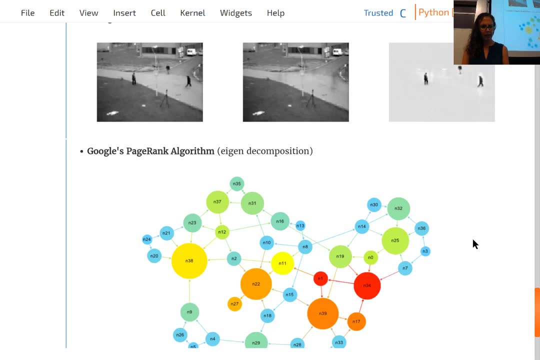 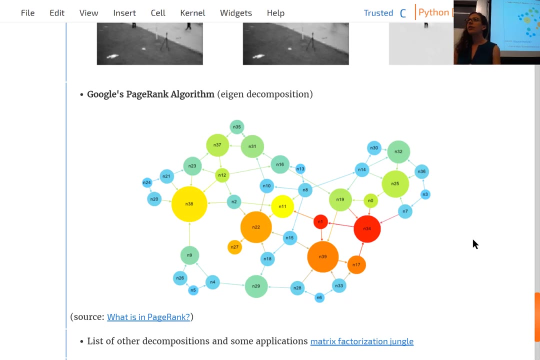 And that's to kind of remove. So we have this surveillance video and we can kind of pick out what's the background and what are the people which could be useful. The PageRank algorithm is all based off of eigen-decompositions and finding an eigenvector. 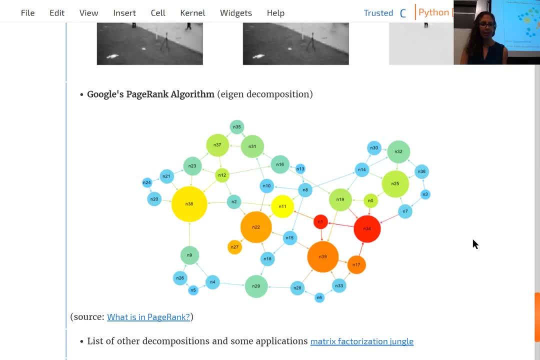 So we'll look at that And we'll look at that on a data set of Wikipedia pages. And then that page I linked to before of the matrix factory. So we'll look at that And we'll look at that on a data set of Wikipedia pages. 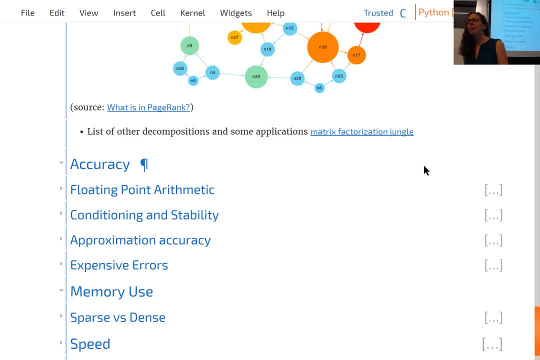 And then that page I linked to before of the matrix factory. So we'll look at that on a data set of Wikipedia pages. And we'll look at that on a data set of Wikipedia pages. So we've talked about quantum distanceウaging. 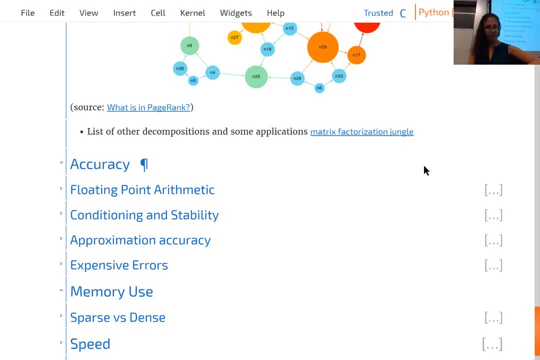 So those are some examples. this data set has some crossovers again and that's why we're looking at it. That other 10-minute screen has a many more crossovers and also a number of embodied graphs within the question of the time recording. 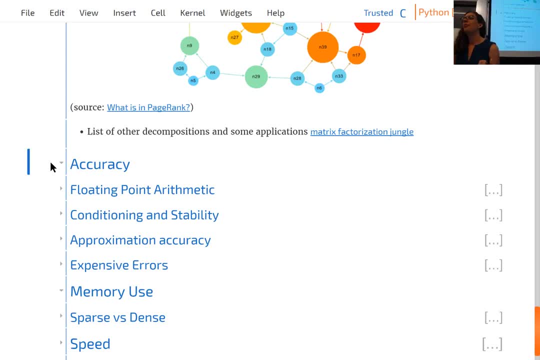 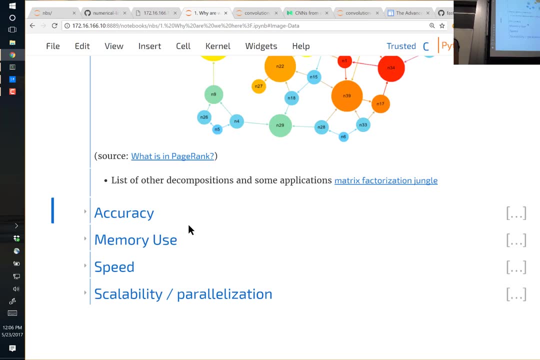 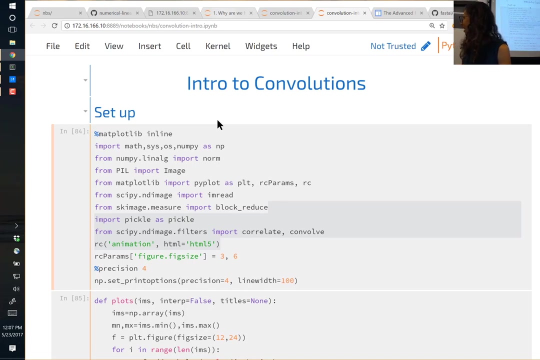 generator that would look quite similar to the map. This is one of the ways that we think about it. So that's an example. All right, so it's 12.07, we're going to start back, and actually, Jeremy said that everyone. 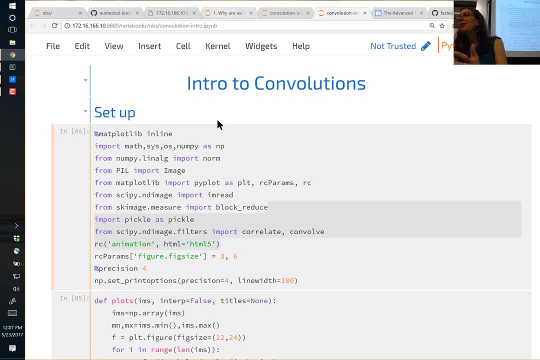 is using, or that the MSAN recommends Python 2.. So he's just going to briefly talk about having both 2 and 3 installed so that you can switch between them. So for those who are interested in trying Python 3, there's only two things you need. 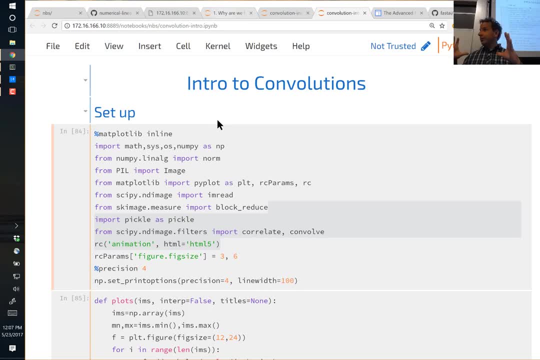 to really know. The first is that print statements now have parentheses around them. The second is that when you divide an integer by an integer, you get a float rather than integer, which makes a lot more sense. But if you're used to the Python 2 behavior, you'll find that surprising. 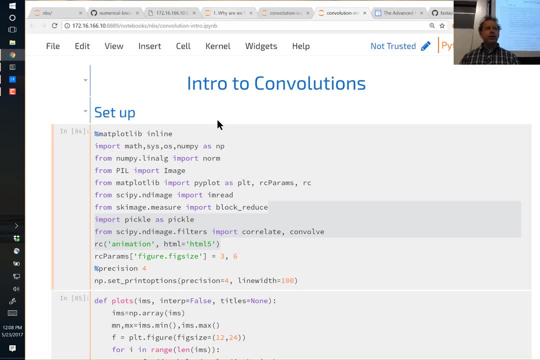 There's a really fantastic thing called Anaconda, which some of you may have come across. It's a Python distribution that, when you install it, it'll offer by default to install it in your home directory rather than replacing your system Python, So you can install Anaconda. 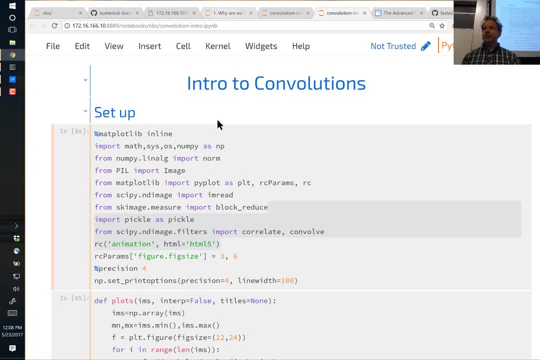 And that'll give you the latest Python 3.6 that supports all the cool linear algebra stuff virtual is showing, And it won't replace your current Python in any way. So then you've got a choice: With Anaconda, you can actually run multiple versions of Python inside Anaconda. 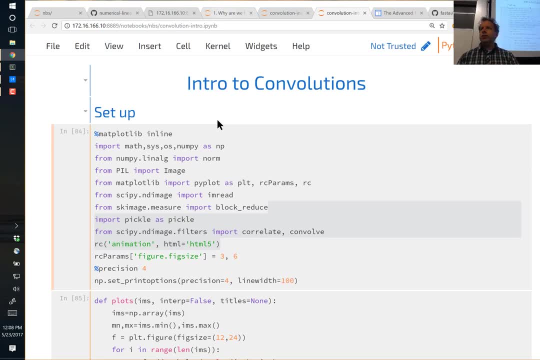 So we can help you do that on Slack if you guys want to do that, Or you can just switch between the two by changing your path to add or remove your home directory Python from there. So that's definitely an option there. I don't suggest you replace your system Python with Python 3.. 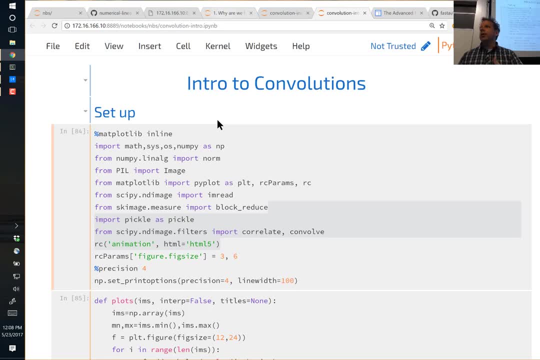 That's going to cause you a lot of confusion, But instead install Anaconda. And another nice thing about Anaconda is that, all of the well, for example, PyTorch, which we'll be using later for using the GPU, by far the easiest way to install it is with. 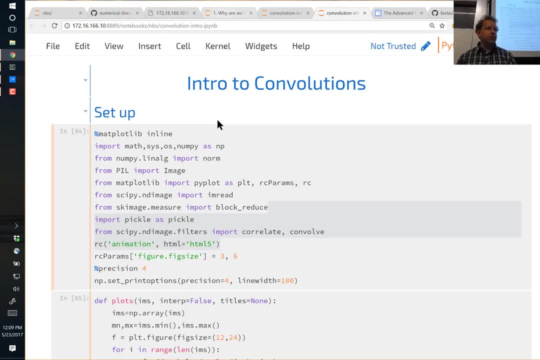 Anaconda. In fact, that's the officially sanctioned method, So there's an option there, So that's a nice thing. There's a number of reasons maybe to try out Anaconda, But definitely don't replace your system. Python Great. 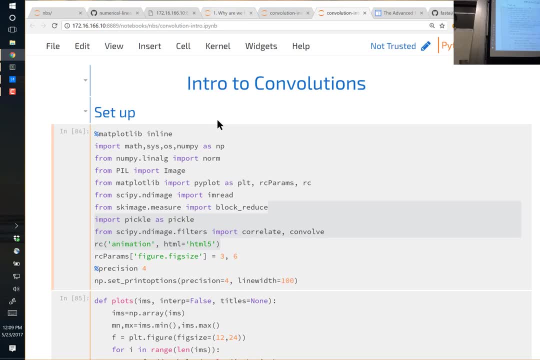 Thanks, Jeremy. Yeah, So feel free to ask on Slack or ask either of us if you have questions about that. And then also I want to say Python 3 is not required for this course. So if you want to keep using Python 2, that's fine as well. 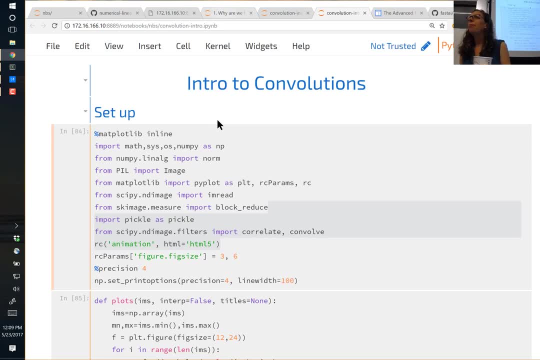 But it is a neat option, And Anaconda and Jupyter both make it pretty easy, Something that's nice about Jupyter: When you start a new notebook, it will ask you which kernel you want to use, And so, if you have both installed, you can choose whichever one you want. 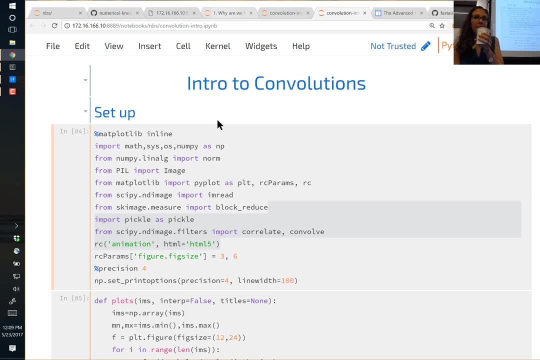 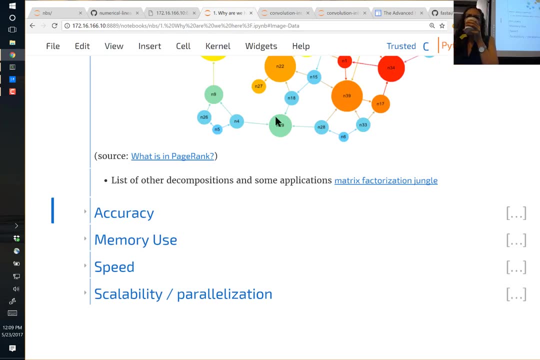 Rachel's code often won't run as is in Python 2, if you are using Python 2.. But we can also show you a couple of lines you can add to the top of every page, which makes a Python 3 file largely compatible with Python 2.. 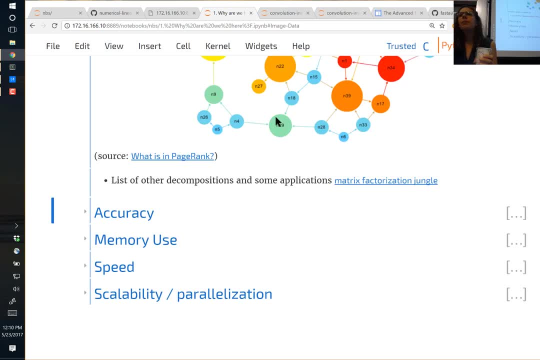 So we should probably start adding that to our notes. Yeah, And then also, as Jeremy said, many of the things that don't make Python 3 compatible with Python 2.. And it's adding parentheses around your print statements or, I guess, some casting if we were. 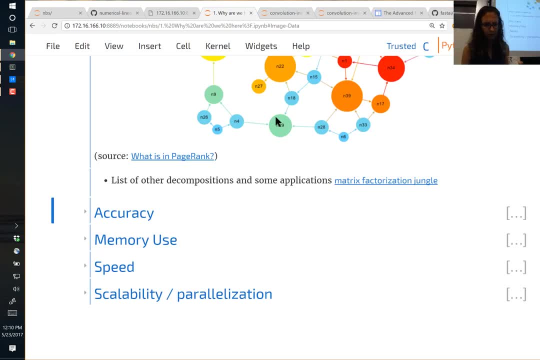 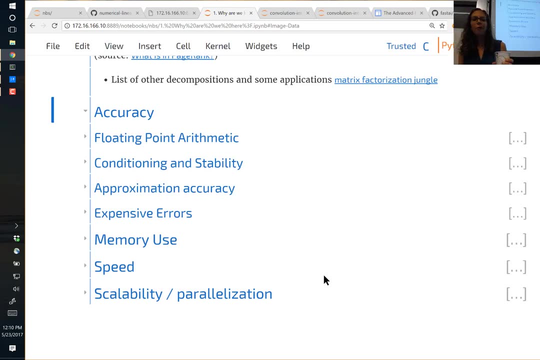 dividing integers by integers to get floats, Okay. So yeah, In this part I'm going to talk about kind of four huge areas of concern in numerical linear algebra Or when doing matrix computations on a computer. So I'm going to talk a little bit more about that. 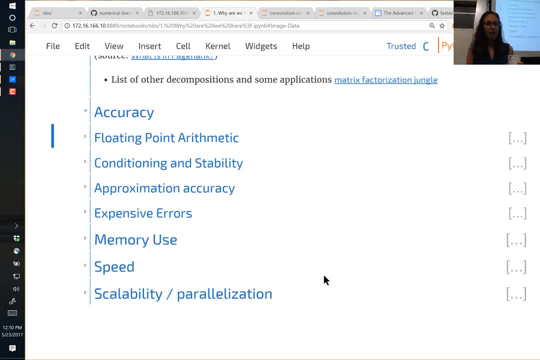 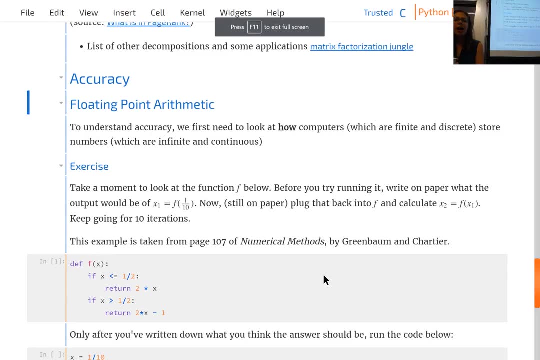 And then I'm going to talk a little bit more about some of the other things that we can do to get those computations on a computer in general. So the first is: let me go to full screen again. The first is floating point arithmetic. 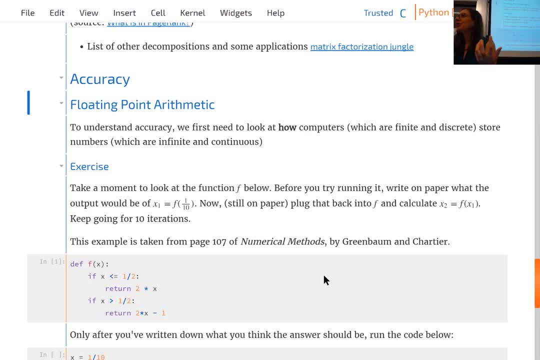 And so, to understand accuracy, we need to look at how computers store numbers, Because it's- and this is something that really I hadn't thought about until I got to grad school- is when you're doing math: it's continuous and it's infinite. 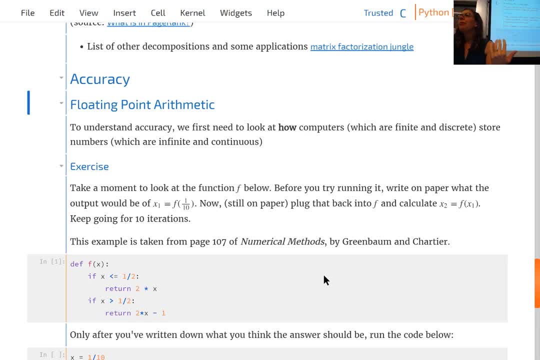 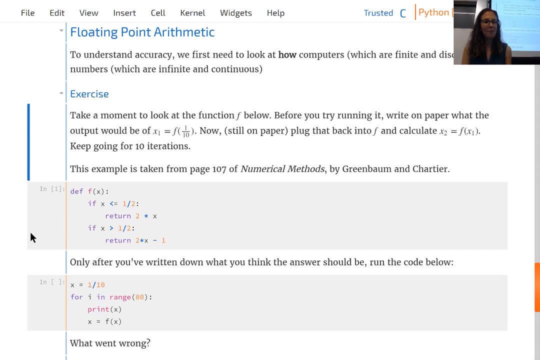 You know, And you kind of have this infinite precision as possible, But computers are inherently finite And inherently discrete. So it's really kind of important to think about how computers deal with numbers in math. So for an exercise, I want you to look at this method F that I have defined. 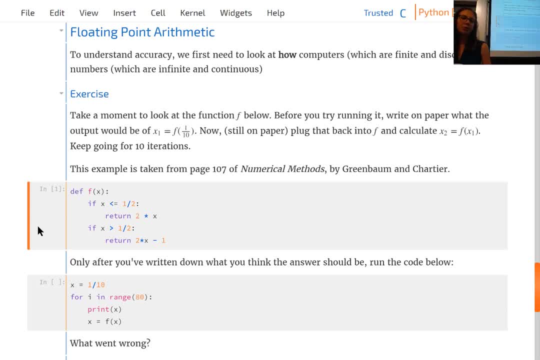 So F takes a value, If the value is less than or equal to a half, it returns two times that value. If X is greater than a half, it returns two times the value minus one. And imagine that we feed one-tenth into that. 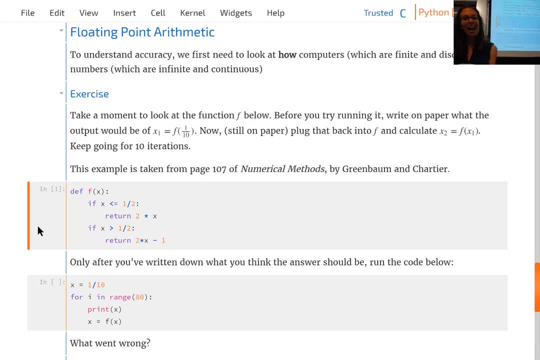 And so that would be one-tenth is less than a half, So it's going to return two-tenths And now feed that two-tenths back into F And I want you to keep doing that and just write out on paper kind of what you would get for the first ten iterations of kind of starting with one-tenth, doing F of that and then do F of your answer. 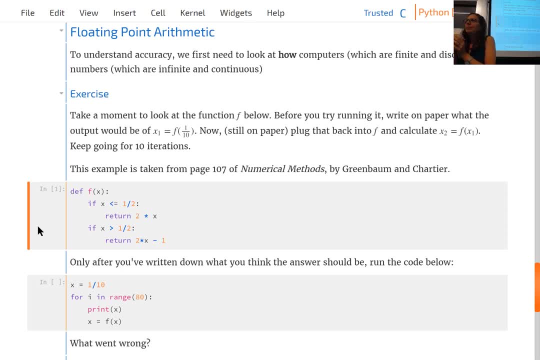 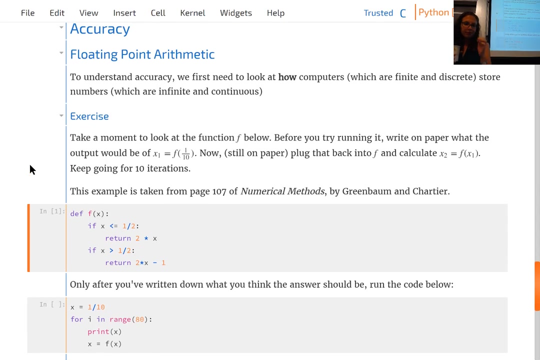 All right, Okay, All right, Cool, All right, Awesome. And this I definitely want you to kind of write out before you run the code: Did I get that right? Yeah, This thing is great, Thank you, Thank you. 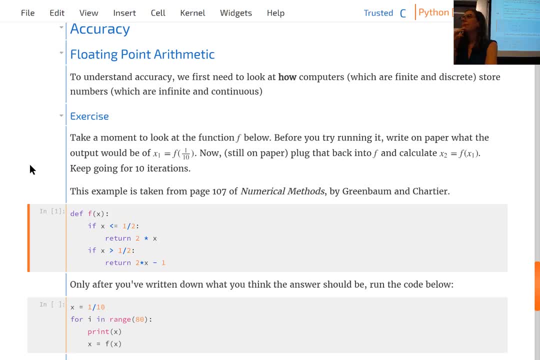 All right, raise your hand if you want more time. All right, can someone tell me what you got for kind of working this by hand? Yeah, that was not great. So I got first one tenth and then two tenths, four tenths, six tenths and then go back to two tenths. 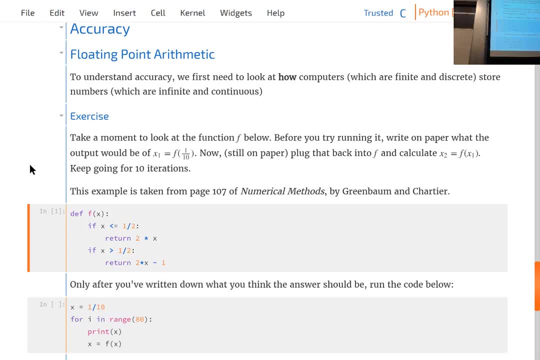 Right, yeah, so it's a cycle. Great, thank you, It's fine. Okay, yeah, so this is a cycle. Okay, So now we're going to try running. We're running it for 80 iterations to see what happens. 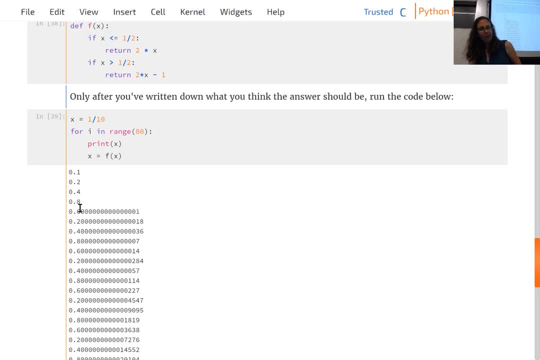 So it starts off: 0.1, 0.2, 0.4, 0.8, 0.6, 0.2, 0.4, 0.8, 0.6.. But what's happening? as this goes on? 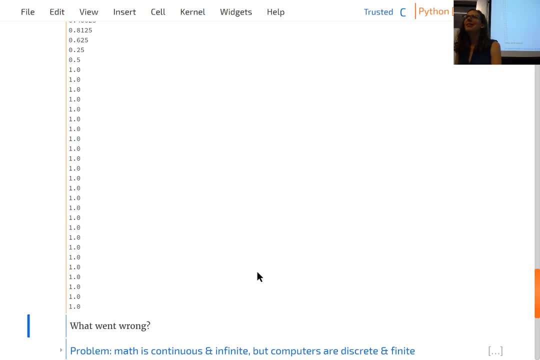 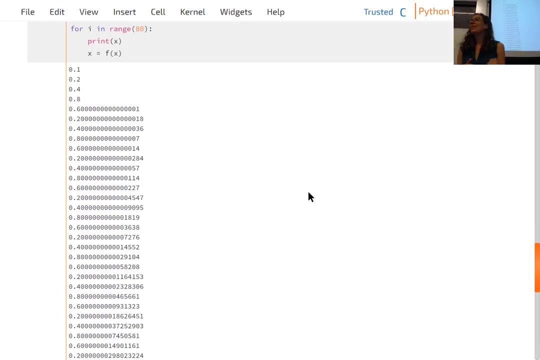 And then we actually end up getting one just over and over again. So the method on the computer has converged, So it's going to be 1 over 1 being the answer, And I think this is pretty cool, Like it's a fairly simple example and it's something that you can work by hand and work. 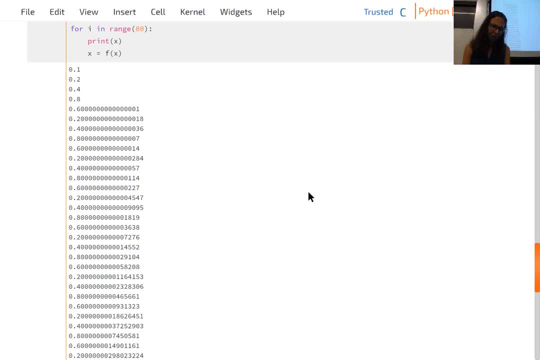 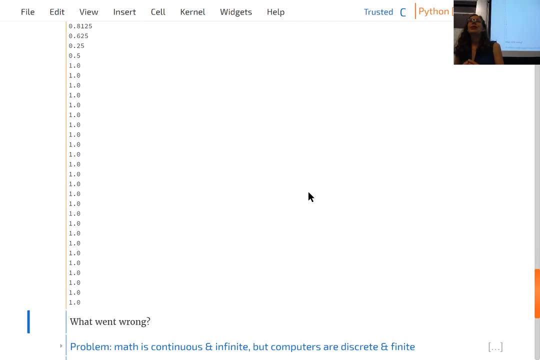 on the computer and you're clearly getting two different things, And so we'll talk about this in a moment. Something to keep in mind is that when you do get kind of these computer kind of numeric errors, it's often happening with repetition, when an error is kind of getting multiplied. 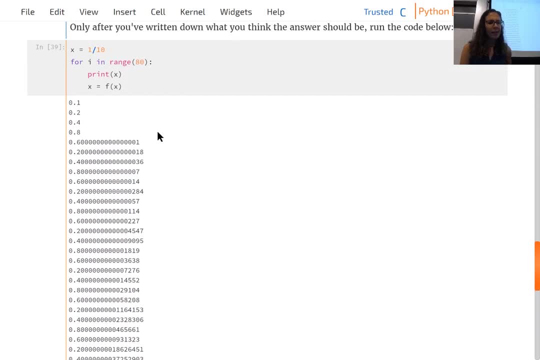 Because you'll notice that this- oops, let me go back up. You know this wasn't exactly 0.6, but it was pretty close. right, It was 0.6, I don't know how many- 10 zeroes or something, and then a 1.. 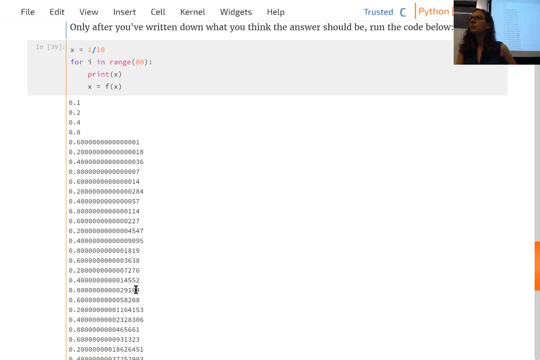 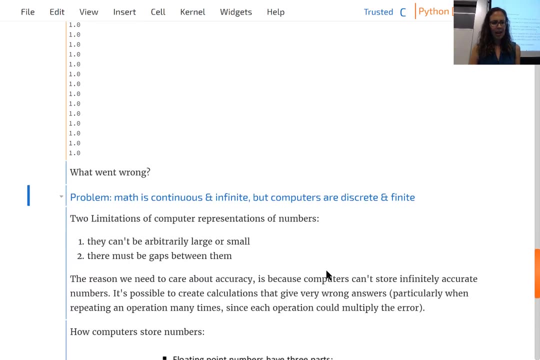 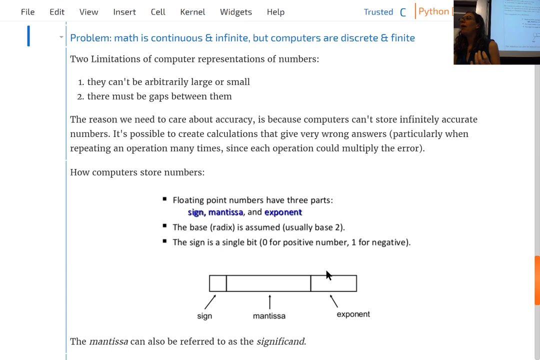 So that's a pretty small error, But those got bigger and bigger, kind of how far it was off. Yeah, and so the kind of the two limitations of how computers represent numbers are numbers can't be arbitrarily large or small, Like there has to be some limit. 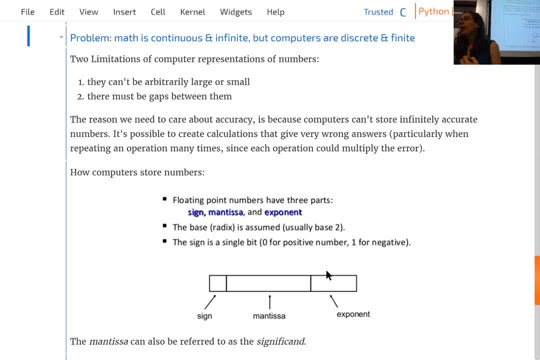 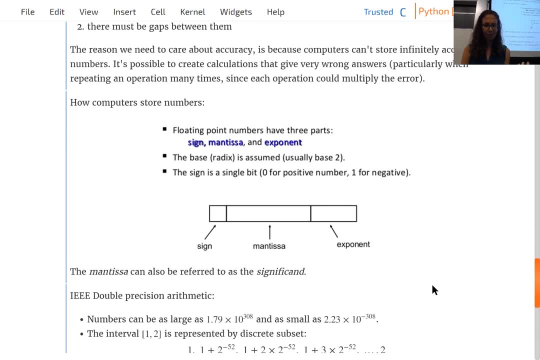 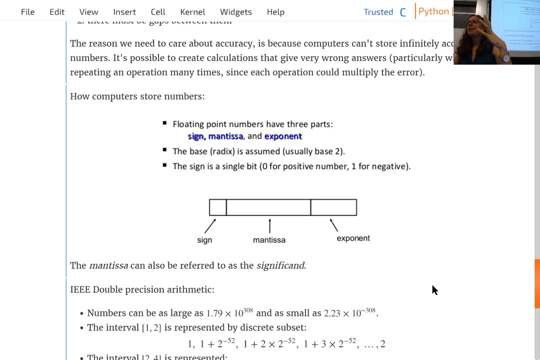 And there have to be gaps between them. They can't be continuous. And so the way that computers store numbers, and this is called floating point arithmetic- And I want to specify: floating point arithmetic is just one piece of accuracy, So we're kind of talking about the broader concept of accuracy on a computer. 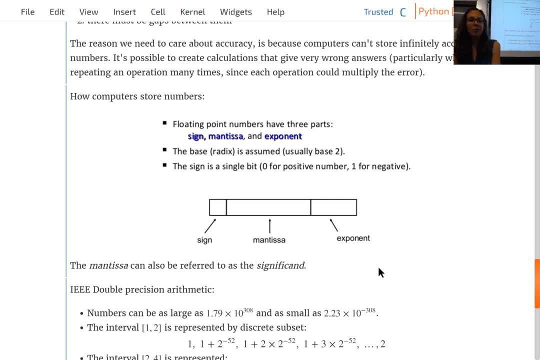 and this is one component to consider. But floating point numbers have three parts. There's a sign- This is just a single bit- positive or negative- And then there's a number, And then there's a number, And then there's a number. 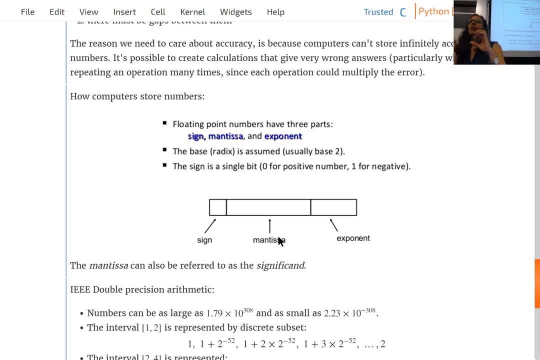 Now what's called the mantissa, or often the significant, And that kind of has the digits. If you're familiar with scientific notation, when you have the like 1.73, that's you know that's the mantissa. and then in scientific notation the ratex is 10,, which is the base. 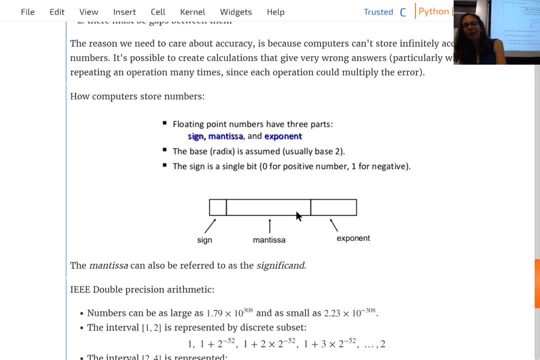 And you know you have an exponent. So you've actually kind of seen this before of having significant and exponent In computers. the ratex is 2.. But this is the idea And that you- I mean the computer- has to be the exponent. 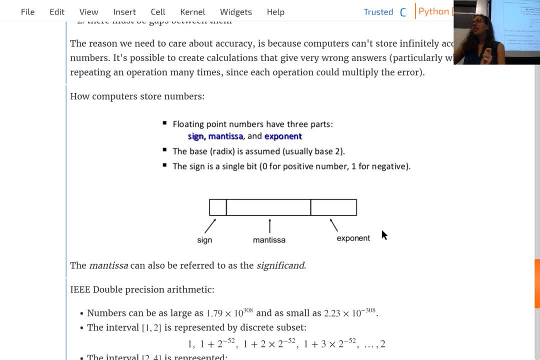 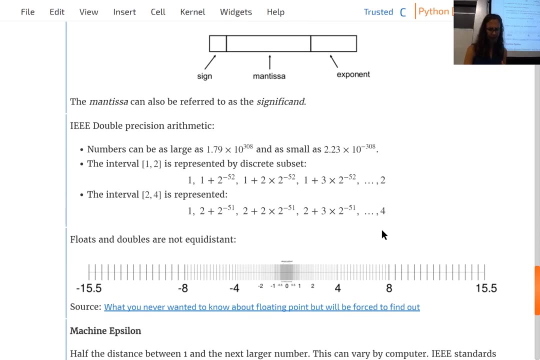 has to make space to sort store these things: the sign, the number of digits, and are the significant kind of the value or precision of those digits, and then the exponent, and so I Triple. E is a set of standards that came out and I haven't written down. I think it was maybe like mid 80s about how computers should store. 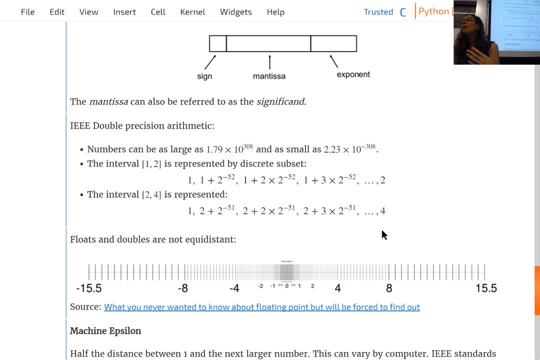 numbers, and it's really great to have something that's consistent, no matter what type of computer you're using, because that could be a big issue and in the early days of computing there people were doing different things. so this is just- and we will talk about this a little bit- Python. so if you've primarily 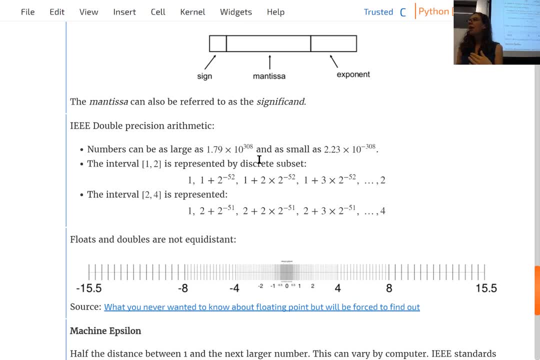 been using Python. Python doesn't require you to say what your types are and kind of hides that from you. many languages, and particularly older languages, you had to say what type something was and that's what the computer knew, how much memory to set aside, and so, for what we think of decimal numbers, they're. 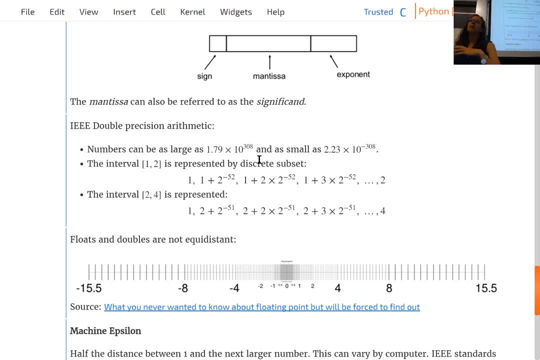 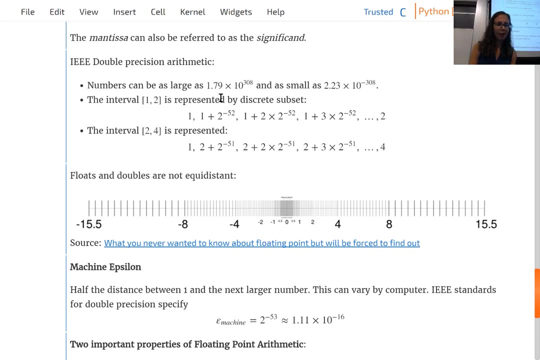 actually, you know, typically a float or a double, those are both kind of same type of numbers, but double saying you want more space to store it, and so here I've just said: and Python is handling all this stuff behind the scenes. it just kind of hides that from you. yeah, so here are what the requirements for doubles. 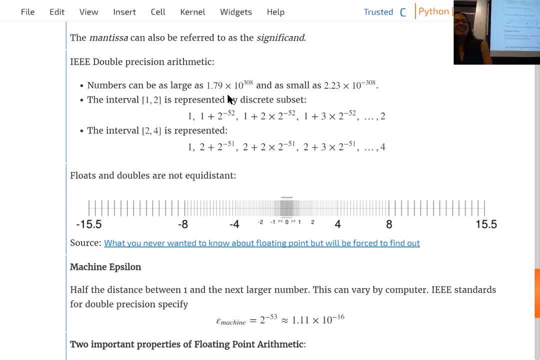 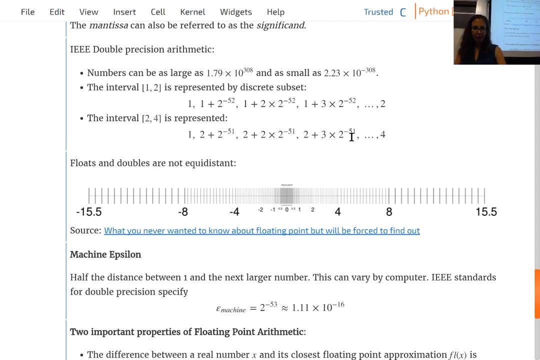 are. numbers can be as large as this is something- 10 to the 308th, which is that's pretty big, or as small as 10 to the negative 308th, and then I think I think this is really interesting the way that they're represented. so we'll think about the interval from 1 to 2. you can. 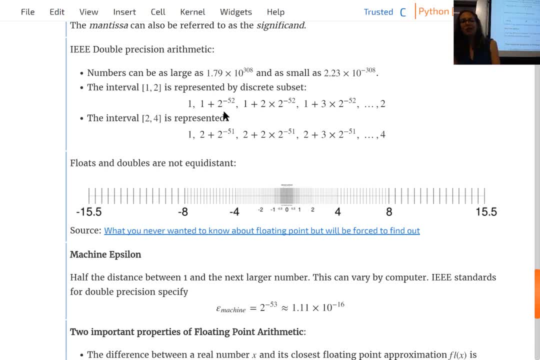 represent 1, and then 1 plus 2 to the negative 52, 1 plus 2 times 2 to the negative 52, 1 plus 3 times 2 to the negative 52, and so on up to 2, and then the interval from the interval from 2 to 4 is going: oh, and this is an. 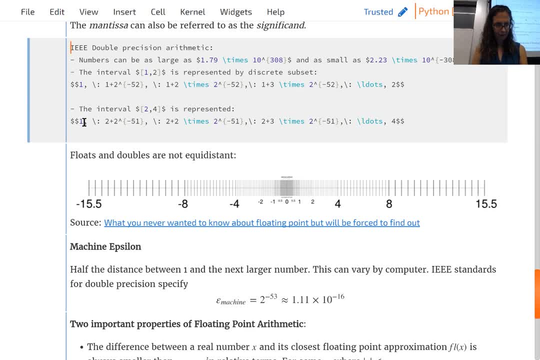 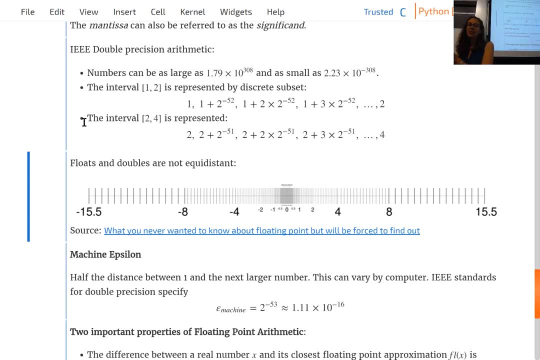 error change. that should be a 2 is going kind of. you can represent 2 and then 2 plus 2 to the negative 51, 2 plus 2 times 2 to the negative 52 plus 3 times 2 to the negative 52. 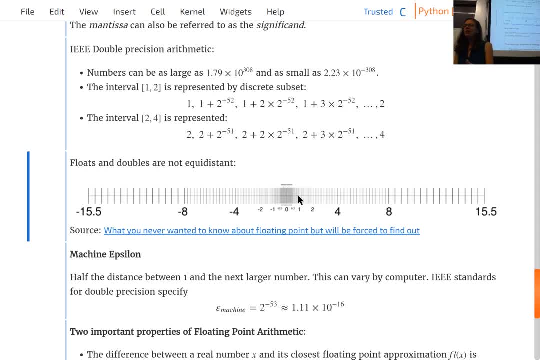 and so the you'll notice the numbers are not equidistant apart. basically, the bigger that the magnitude of the numbers get the kind of, the more they're spaced out, which I think is kind of weird and interesting. so this is a nice kind of a graphic showing that that close to, kind of for small numbers they're closer. 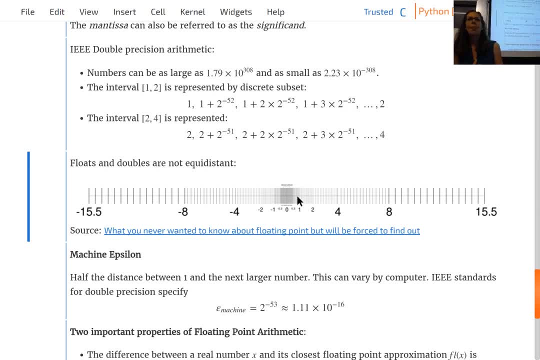 together. Jeremy, I just thought it was worth pointing out that the two things that we're using in this class two to represent numbers- being numpy and pytorch, both are typed, given that python isn't. so with numpy, if you feed it a float, it will create a double precision float. if you feed it a float, if anything is a float, it will create a double precision float array. if anything, if they're all ints, it'll create a long integer array and then when we use pytorch, we'll also be explicitly saying what type it is. so we are using typed libraries pretty much explicitly in this course. 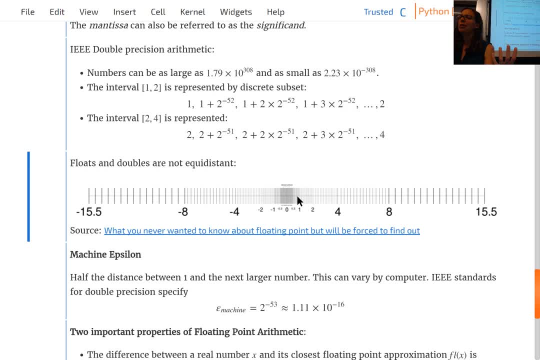 Thank you, That's a great point, And also even another library we'll use is Numba, which lets you add types to Python in general. Oh, just Cython. Okay, Sorry, Cython is the one that lets you add types to Python, So that is something that you will. 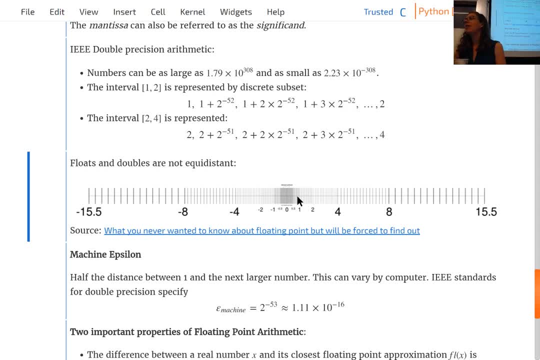 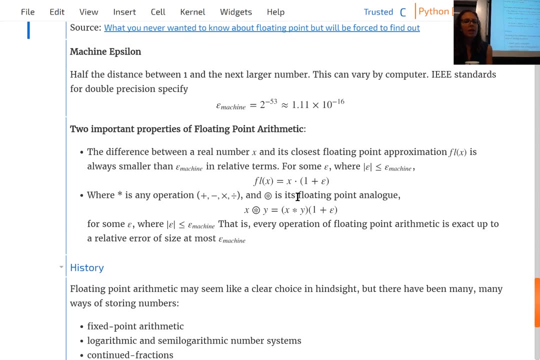 often want to add and that, yeah, NumPy kind of has built in. when you're doing scientific computing and also for improving performance, It typically lets you kind of go faster to handle it yourself, And so machine epsilon that's kind of defined to. 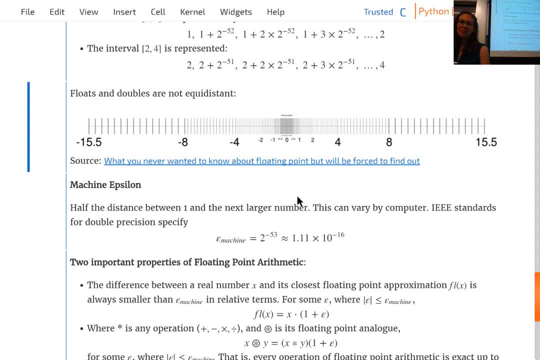 be half the distance between one and the next larger number. So for double precision machine epsilon is two to the negative 53. You can kind of see that up here that the thing kind of the next number after one is two to the negative 52 more. So half of that is two to the. 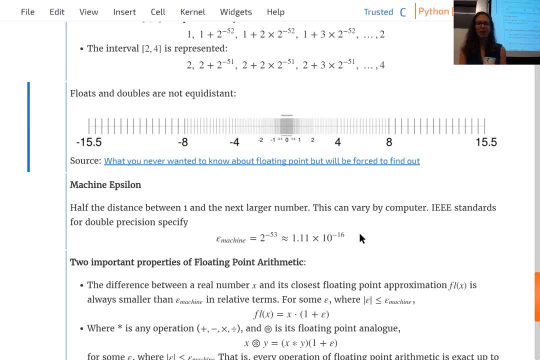 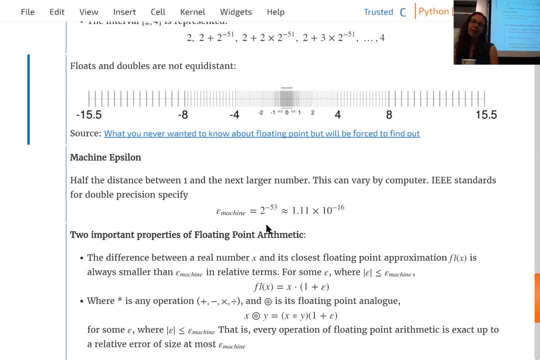 negative 53. And this is kind of a term that you'll hear people talk about, And then converting from base two to base 10, that's equivalent to about 10 to the negative 16th, And we'll see this kind of show up an example later. Any questions? Why does that matter? 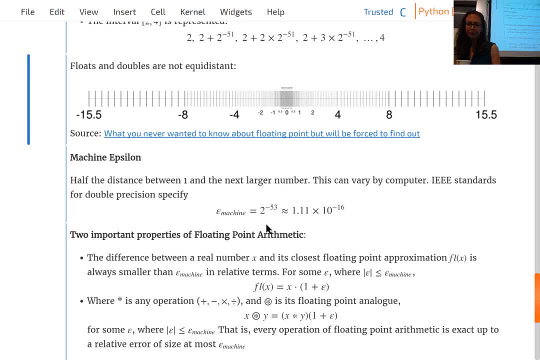 Why does machine epsilon matter? So machine epsilon. often you'll talk about your error as a in terms of machine epsilon, Because that's something that's kind of inescapable that you know the computer can't represent something smaller than that, And so you'll just kind of talk about 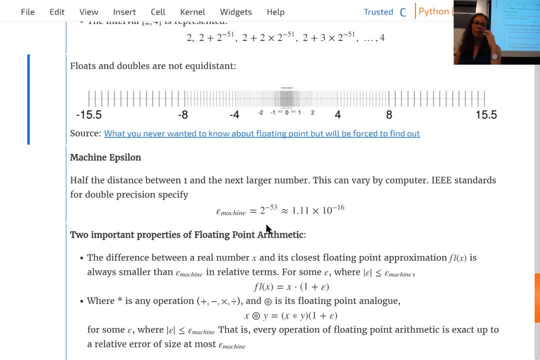 I mean, if you have an algorithm that makes that worse or is, in terms of you know the square root of that, then that's kind of worse than the computer could be doing, And depending on what you're trying to do, it varies what's possible, But this is kind of a good unit. 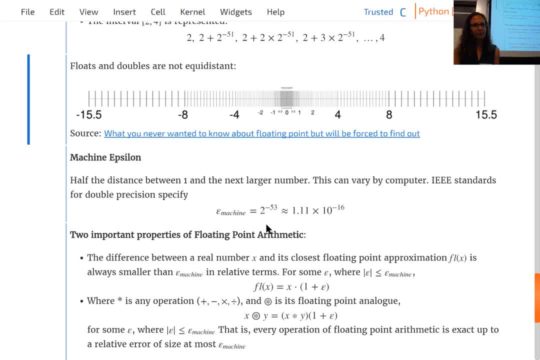 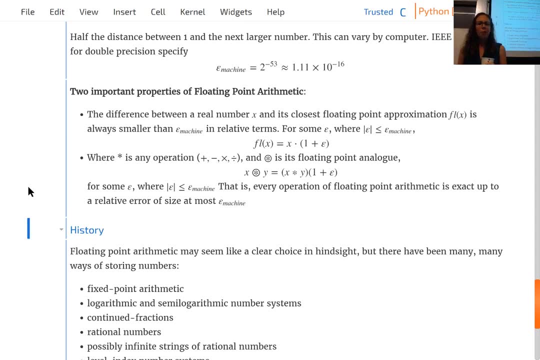 to talk about how you're, how you're doing, And then two important properties of floating point arithmetic. One is that the difference between a real number and its closest floating point approximation is always smaller than machine epsilon in relative terms. So here fl of x is the floating point representation And then the x is kind of the true number. you're. 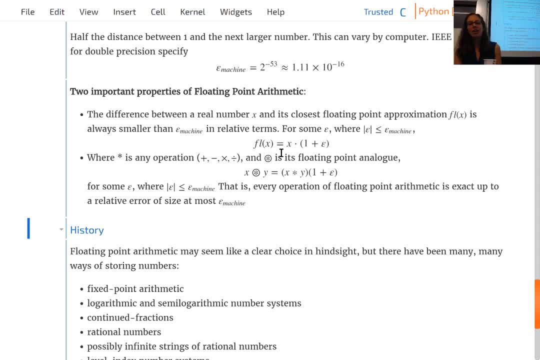 wanting to represent And it's saying the floating point representation is going to be equal to x times 1 plus some epsilon, And that epsilon is less than or equal to machine epsilon. So it's kind of nice. It gives you a bound on your accuracy. 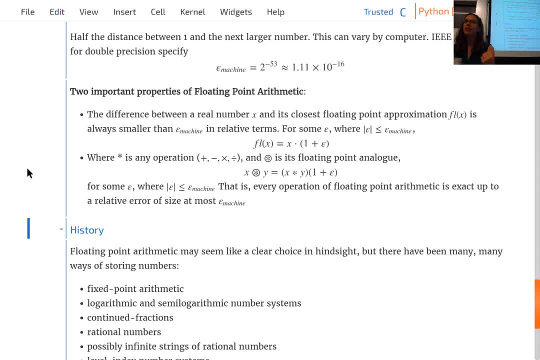 And then for the kind of key floating point operations which are addition, subtraction, multiplication and division. so we'll let star represent that operation And then circle star is the floating point equivalent of that kind of how it's implemented. Your result is going to be no more than a multiple of 1 plus. 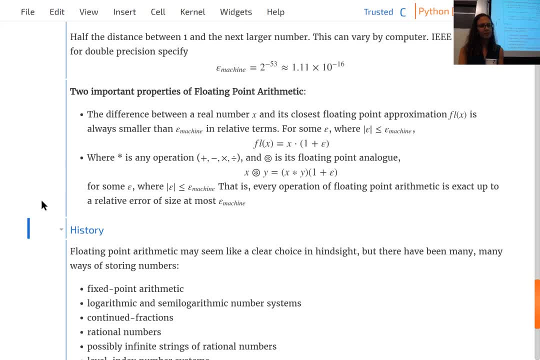 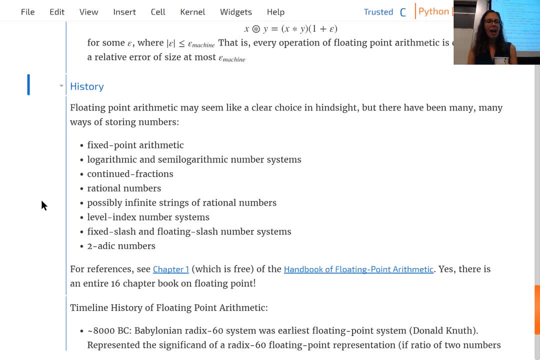 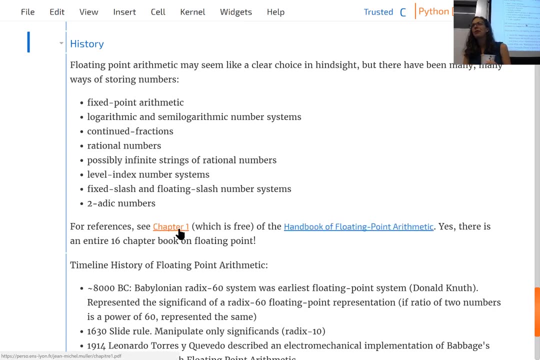 epsilon off. And then this next part I included because I just found it was really interesting to read about. I found there's a book called Handbook of Floating Points Arithmetic, and Chapter One is available for free, But it lists a lot of other types of 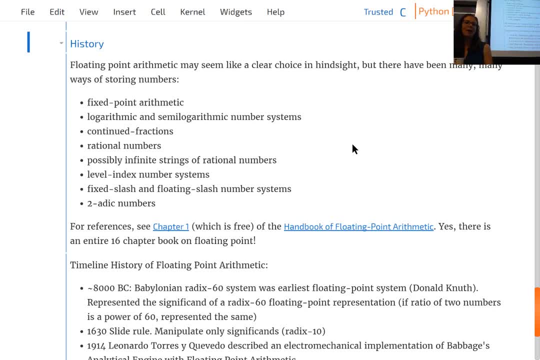 storage schemes that were tried with numbers at various points, And so I don't know what all of these are, but I thought it was an interesting list that people tried kind of possibly infinite strings of rational numbers, floating slash number systems. So there's been a lot of different. 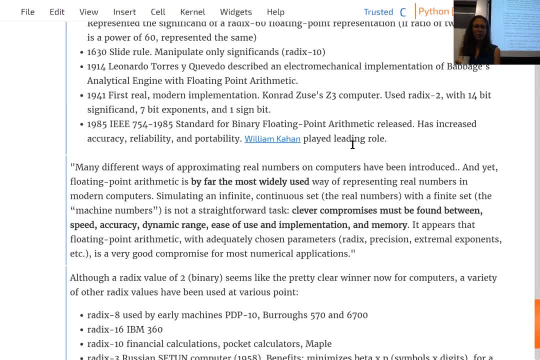 approaches that have tried. And actually let me skip ahead. There's a really nice quote from the book that really you're having to make compromises between speed, accuracy, dynamic range, ease of use, implementation and memory. They're kind of like all these different considerations And that. 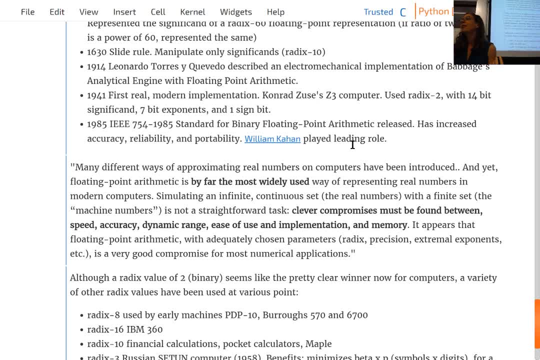 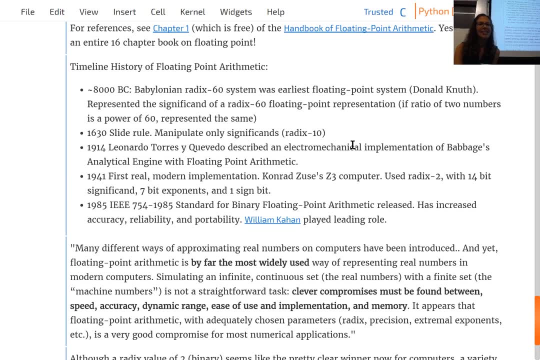 floating point arithmetic seemed to be a good compromise for kind of all of this, And a lot of people kind of converged to accepting this. Here is an interesting history of floating point arithmetic. Donald Newth cites the Babylonians as being the you know, the you know. 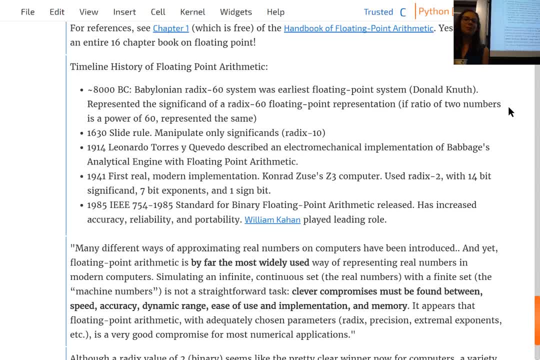 first to have a floating point arithmetic system And theirs was base 60. And that was 8,000 BC. In 1630, the slide rule was invented, And there you're manipulating only significance. That's base 10. And radix and base are kind of the same thing. 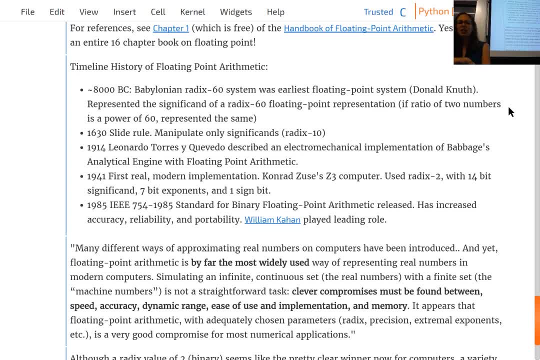 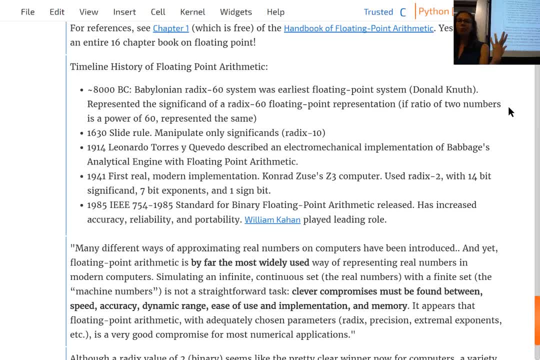 the Z3 computer. Conrad Seuss made the Z3 computer. Conrad Seuss made the Z3 computer, And Conrad Seuss lived and worked in Nazi Germany, And so he was really cut off from the rest of the scientific community, And so he built some very interesting computers that kind of nobody else knew about. for 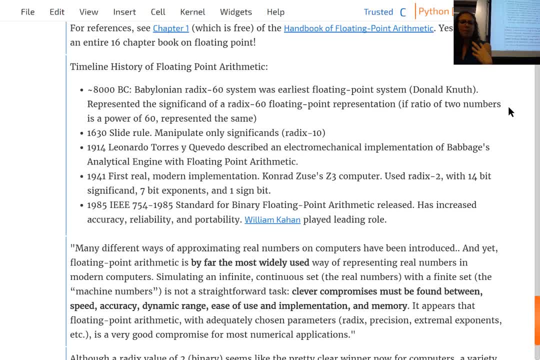 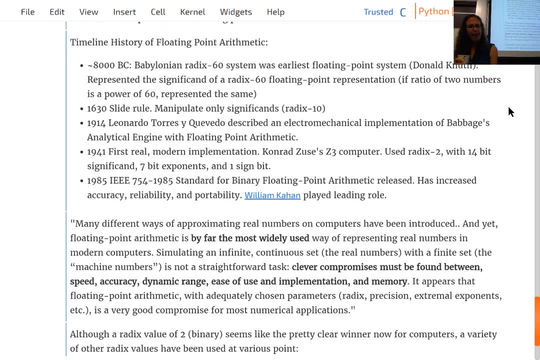 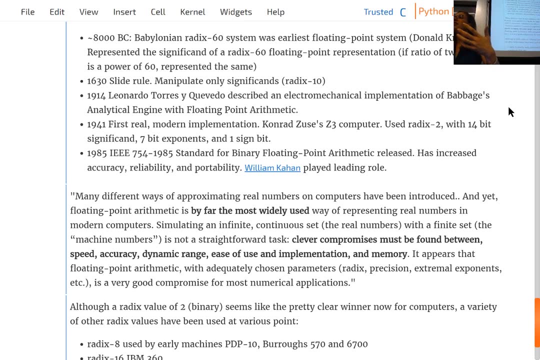 quite some time, although many of them were destroyed in bombings, But he was the first to kind of kind of implement this in a modern computer. And then, yeah, 1985, and William Cahan, who was, I believe, at Berkeley, played a huge role in kind of pushing for this standardism. 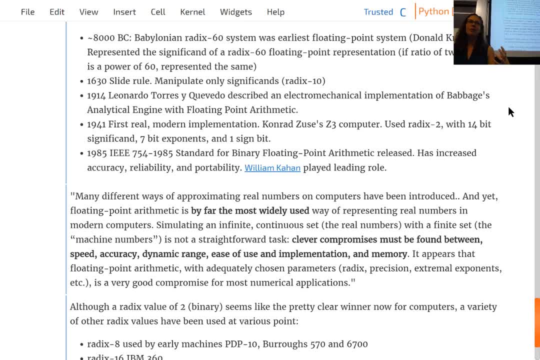 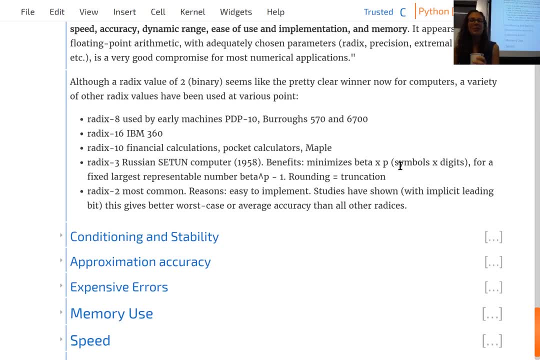 And then, yeah, 1985, and William Cahan, who was, I believe, at Berkeley, played a huge role in kind of pushing for this standardization, of wanting different computer manufacturers to be doing the same thing. And then, just real quick, so I think with computers you know kind of zeros and ones. 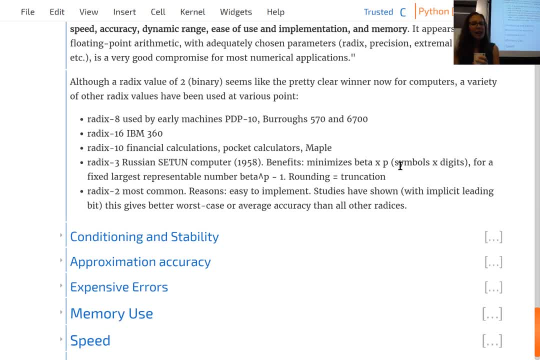 Radix. having base two seems to make a lot of sense. Apparently, the Russians were using Radix 3 for a while and there are some benefits to that. I mean, this was in the 50s, Everyone's. The Russians actually had a whole series of ternary-based computers, so that was a good idea. 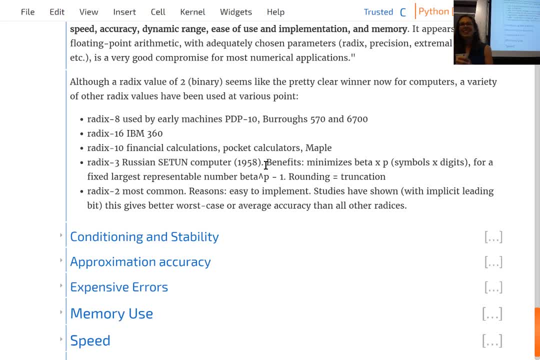 That was actually the hardware level where you could see 3-bit, 3-level stuff. Pretty cool, Yeah, and it was. I mean, it was neat because it says that this does kind of minimize in some ways, like the number of symbols times digits you have to use. Also, rounding gets nicer. 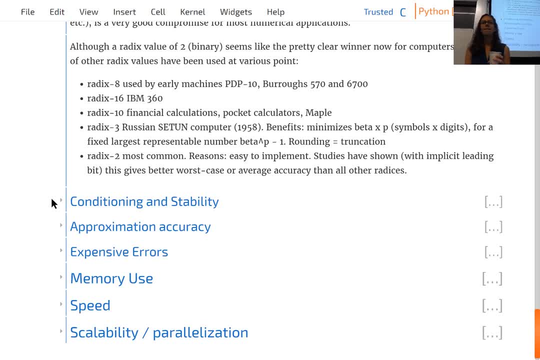 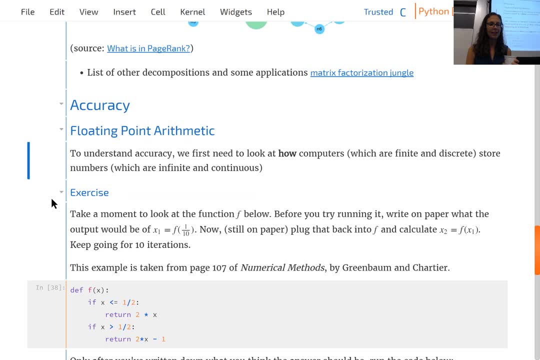 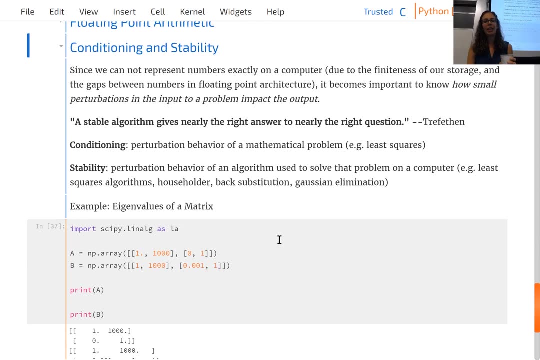 Okay, any questions about floating point? Okay, so we're still under. Let me pull these up. We're still under the sub-point of accuracy right now, but the next thing to think about with accuracy is conditioning and stability. And so, since we can't represent numbers exactly on a computer, 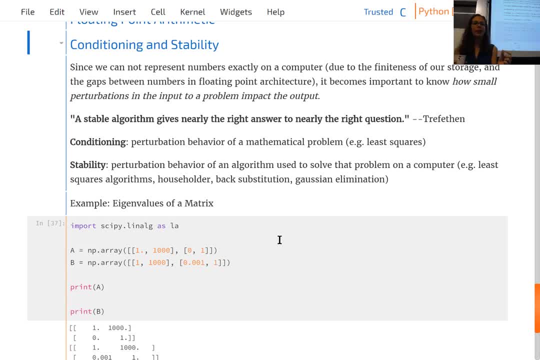 it becomes really important to know how having a small change in your input affects the output, because sometimes that's going to happen inevitably with how you're representing your numbers. Okay, And so Trevathan had a quote- author of this book, kind of a classic- saying: 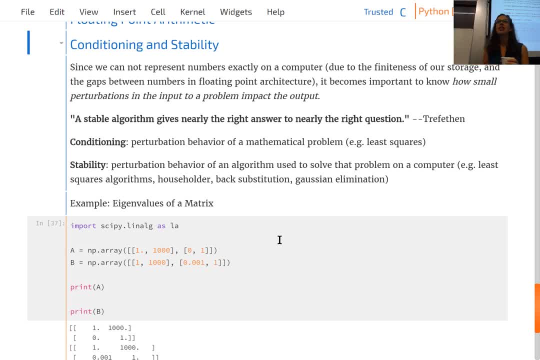 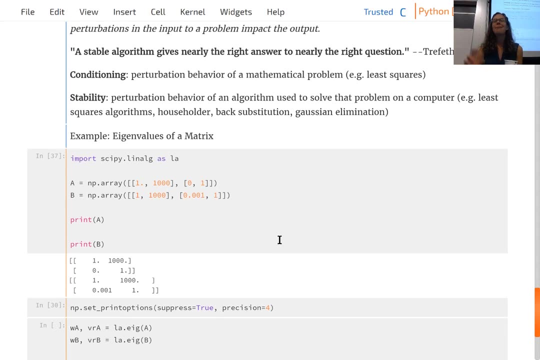 a stable algorithm gives nearly the right answer to nearly the right question, And so that kind of nearly the right question is referring to. you can't represent your numbers exactly, and then you want your algorithm to be doing nearly the right thing. Conditioning and stability- and I think many people kind of use them as synonyms- 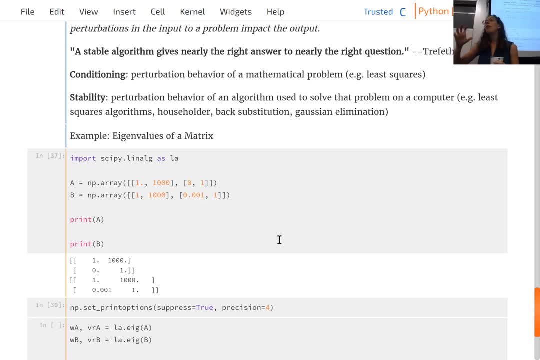 Technically, conditioning is referring to the problem itself: how it behaves under perturbations which are small changes to input. Stability is about the behavior of an algorithm, And so we'll be talking about it in the context of a few different algorithms. 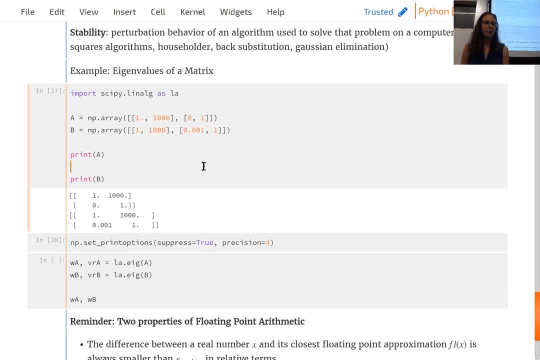 And so then a kind of simple example is: we look at the matrices A and B, So A is 1, 1001,, B being 1, 1000, .001, and 1. These are very similar matrices, right? 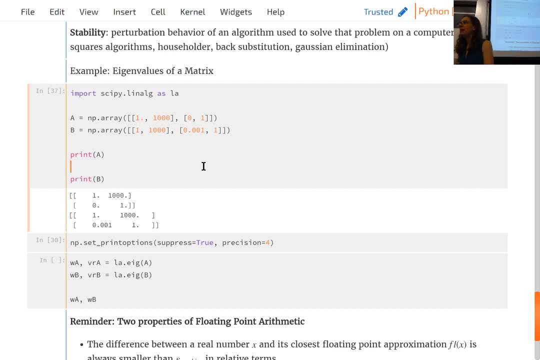 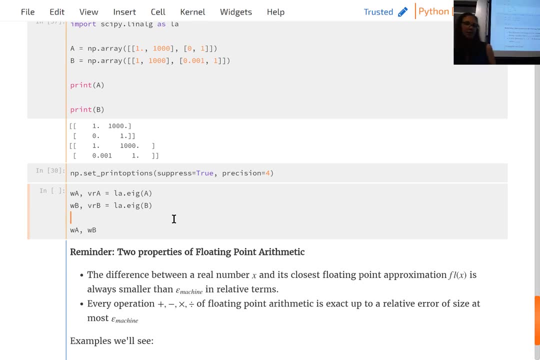 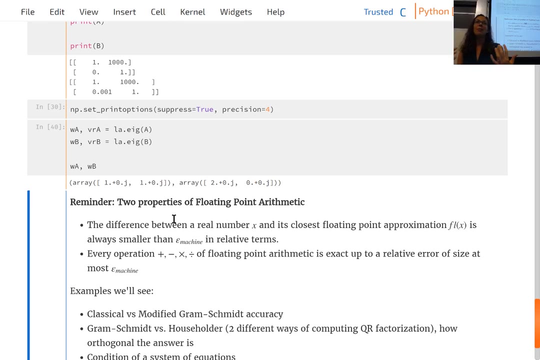 There's only a .001 difference in one entry between A and B. If you calculate so, you would actually kind of hope that these would have similar eigenvalues, and they don't, And that's not because of how we're calculating them. 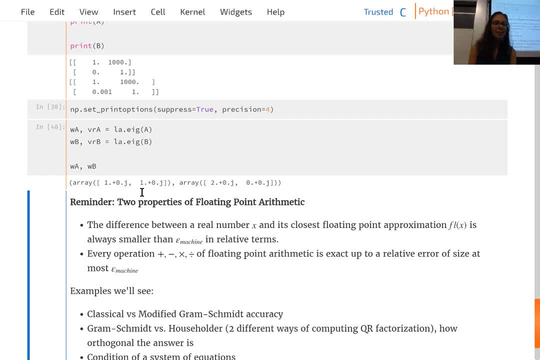 That's kind of an issue of the problem of finding algorithms. Oops, I don't know why it's so happy about highlighting So here. for A, the eigenvalues are 1 and 1.. It has a kind of multiplicity: 2 for the eigenvalue 1.. 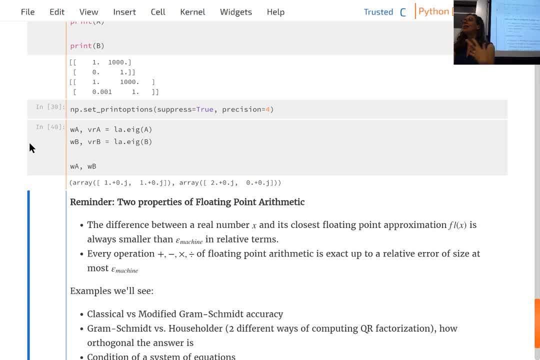 And then for B they're 2 and 0. So those are very different. What's the J And J is for the imaginary term? A lot. we are just- we're just going to focus on real numbers in this course, but a lot of these. 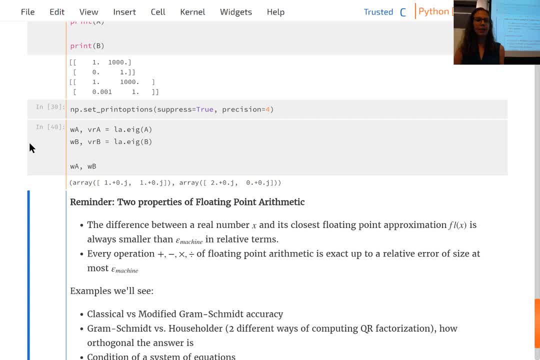 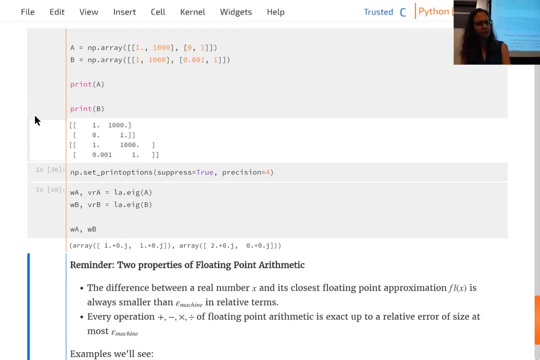 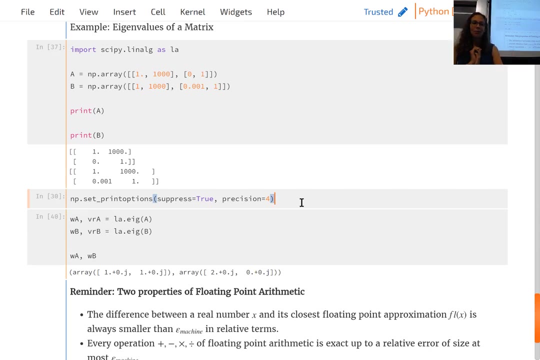 problems in general can give complex values, And so real valued matrices can have complex valued eigenvalues or eigenvectors. And then I also just wanted to highlight, because I think this command is so useful: npsetprintoptions- suppressed equals true. 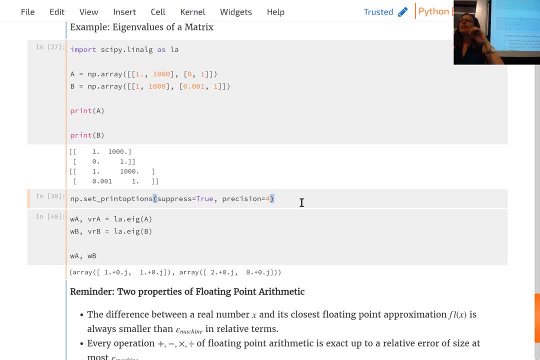 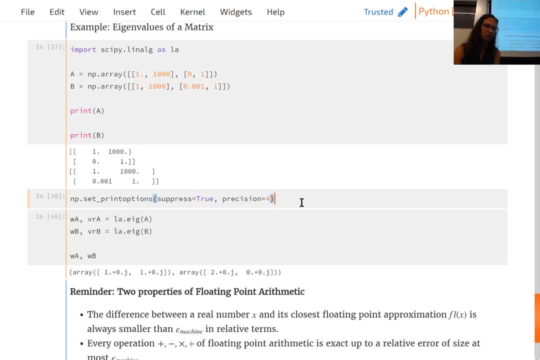 So suppressed equals true, turns that off and makes makes your zeros just show up as 0.. Any questions about the eigenvalue example And so that is something kind of to keep in mind, kind of things you'll see that relate to the math, because this is something even if you weren't using a computer and you solved. 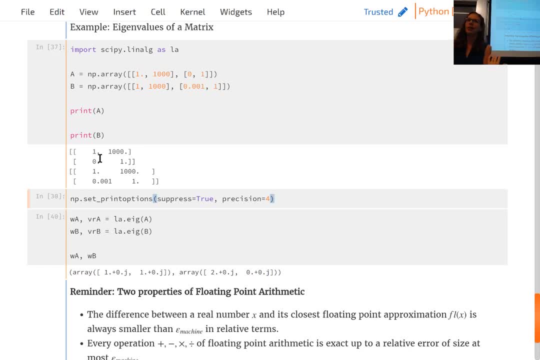 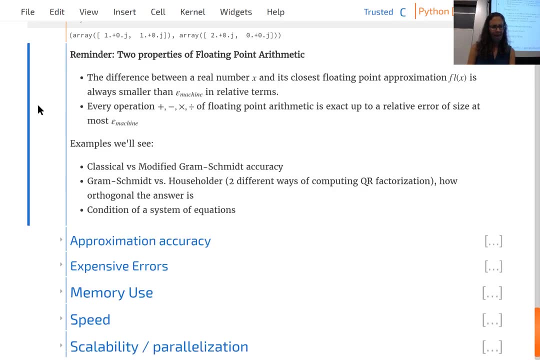 for the eigenvalues by hand, you would still get these different answers for what are fairly similar inputs. Yeah, and then just looking ahead, this will come up again when we talk about classic versus modified Gram-Schmidt, which are methods for the QR factorization, also with Gram-Schmidt. 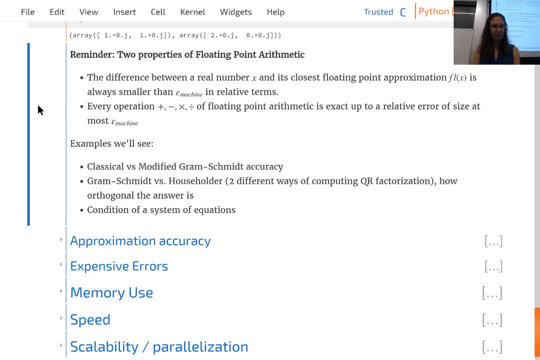 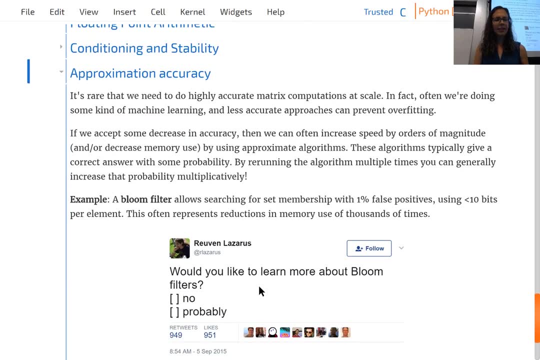 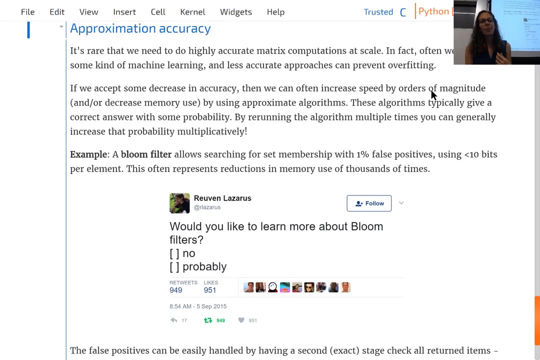 versus Householder and conditioning a system of equations. And then another area to kind of think about with accuracy is approximations. It's actually pretty rare that we need to do highly accurate matrix computations at scale, particularly if you are doing machine learning. 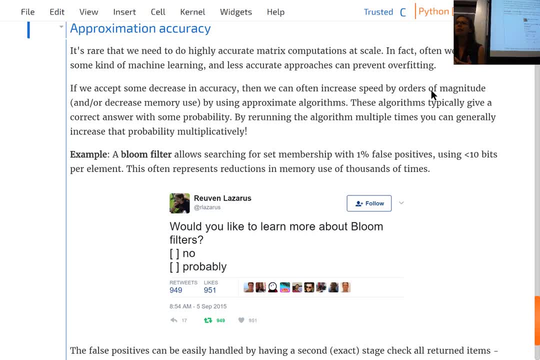 Often being slightly less accurate, is a form of regularization that can help you prevent overfitting, And, if you are willing to accept some decrease in accuracy, you can often increase your speed by orders of magnitude, which could let you calculate an answer several times and kind of. 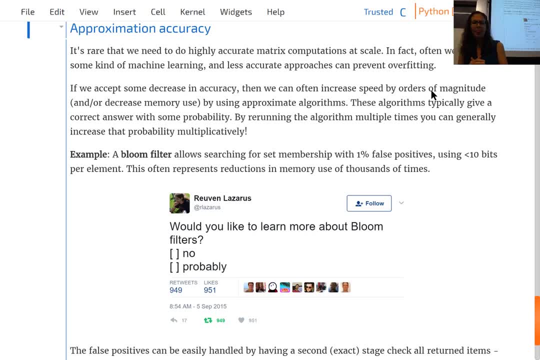 regain some accuracy with that approach. And then I guess an issue that I didn't write down here but to think about is also the quality of your data. Kind of, if you're aware that your data may not be super precise, it's then bizarre to 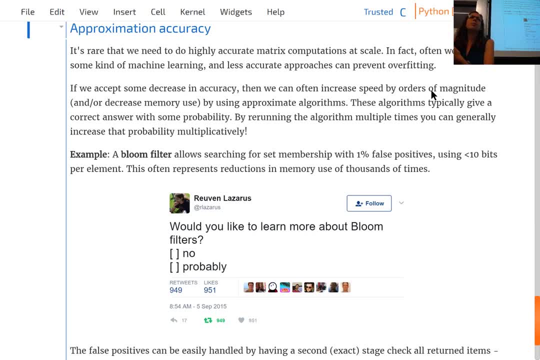 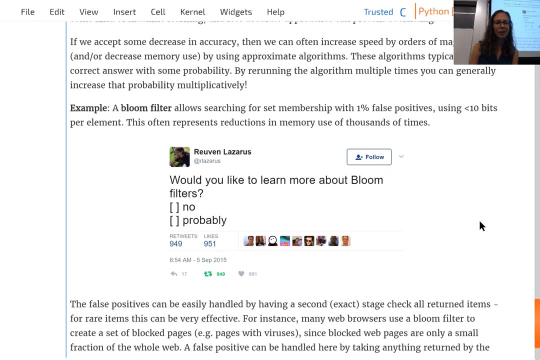 spend a lot of time trying to get the kind of most accurate answer possible when you know that your data wasn't even collected in the most precise way- And I think this happens really a lot in the kind of tech world- And then a kind of popular example. 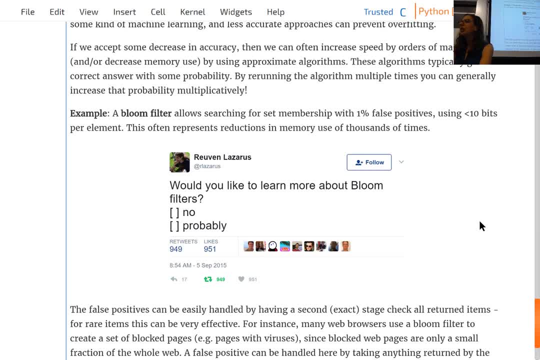 So this idea of kind of inserting randomization or approximation into algorithms, yeah, it's very powerful And a really kind of popular example is a bloom filter and that's something that allows you to search for, set membership with 1% false positives. if you were using that uses less. 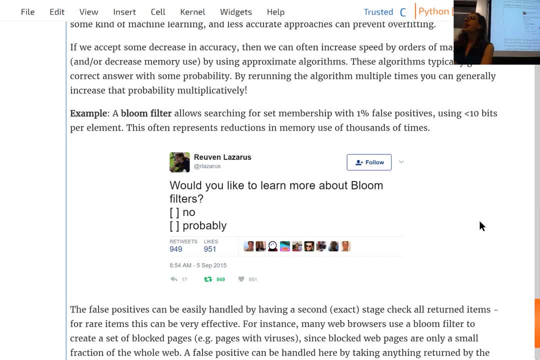 than 10 bits per element. A good idea that Entãos a kind of general idea, is with a bloom filter. if it tells you no, it's definitely no, like you know that's correct. If it tells you yes, that's probably right. there could be some error there. 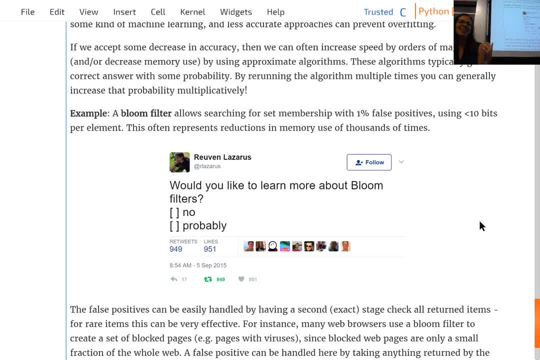 And so this is a tweet. joke about it. Would you like to learn more about bloom filters? No, or probably Because you can never get a definite yes with, but you can get a definite no, And then a kind of a place that they're used is. 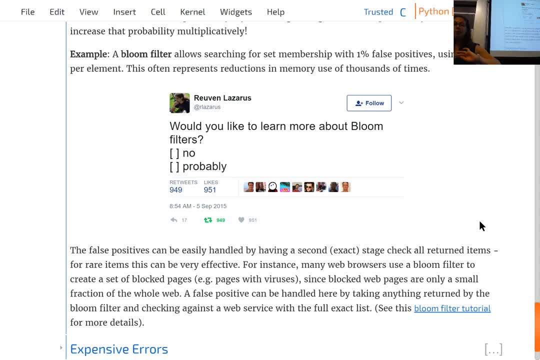 looking for uh kind of: if you want a web browser wants to block pages with viruses, it could use a bloom filter, and if it says no, then it, you know, lets you view the the web page, no problem. 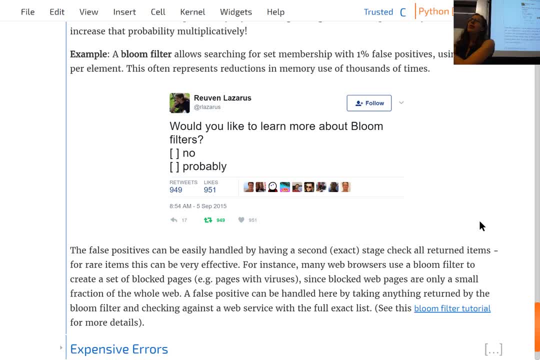 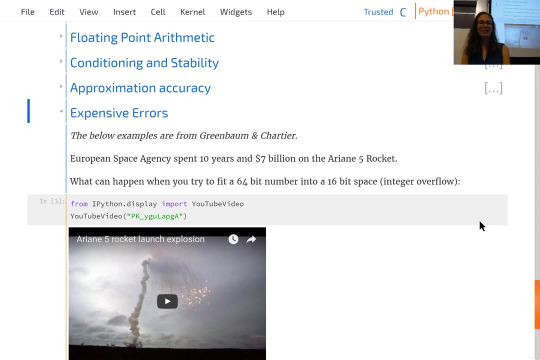 if it says maybe, then it can look it up. um, you know, and that takes a little bit longer, but it's only having to do it for a small percentage of the pages. any questions? okay, oh, and then this is also kind of just for fun, but kind of expensive, expensive airs. 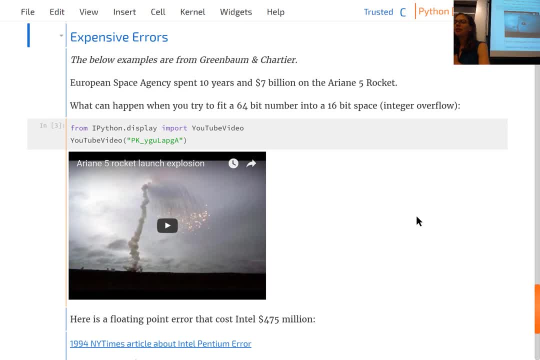 the european space agency spent 10 years and 7 billion dollars on the arian 5 rocket. um, but it was trying to fit a 64-bit number into a 16-bit space at one place, and so it exploded. let me just skip ahead to that. 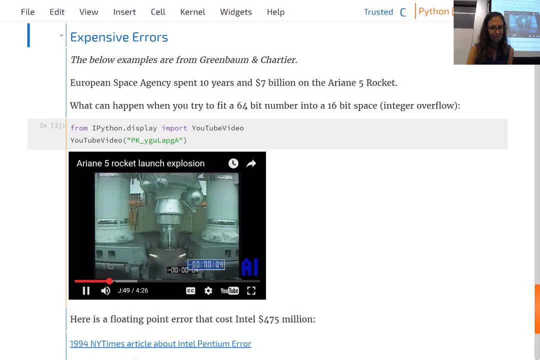 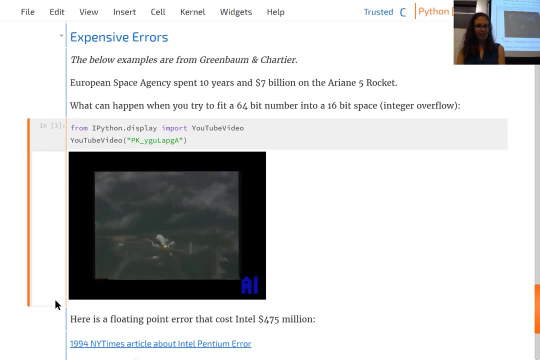 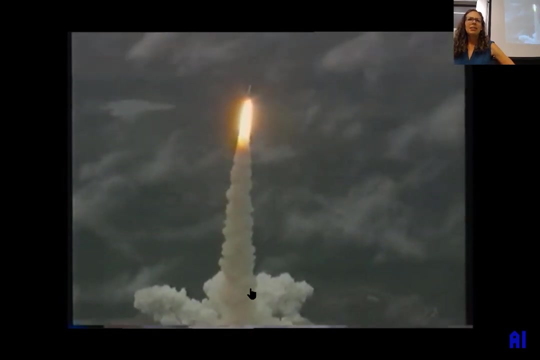 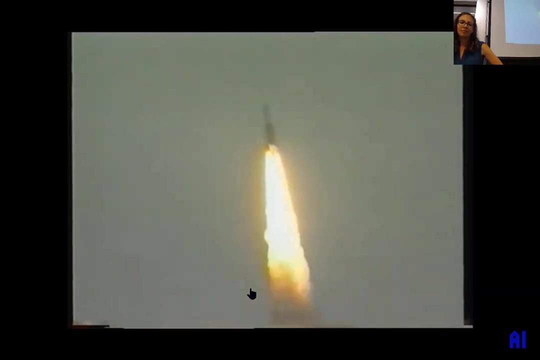 sign alimaj decollage. this happened, i think, in the 90s, 94. yeah, there was also. i can say, as this is going off, i didn't include it- um that the us had a, a patriot missile defense system um in the middle east, um, and that 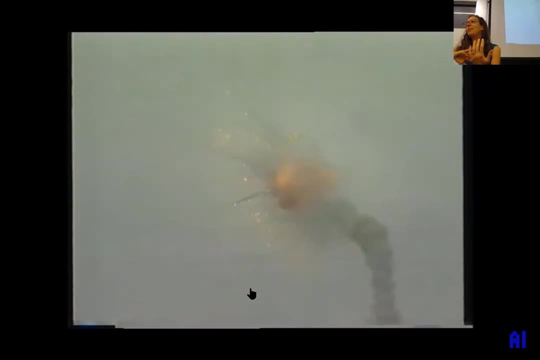 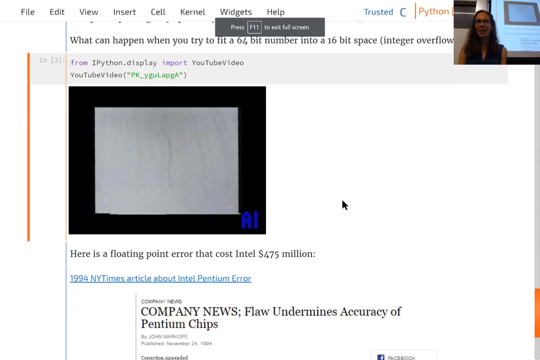 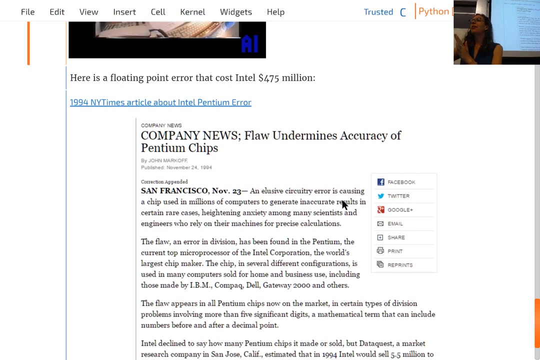 37 seconds into the launch. this was what we were supposed to do, but yeah, so this stuff can have big implications. um, but yeah, as i say, a us kind of missile defense system, um its clock like gradually got more inaccurate and it actually they made i think 28 people were like killed by a missile that it failed to recognize. 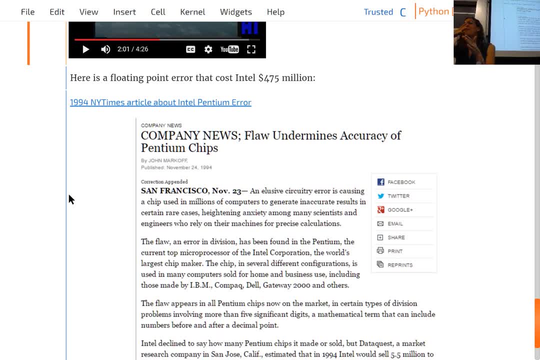 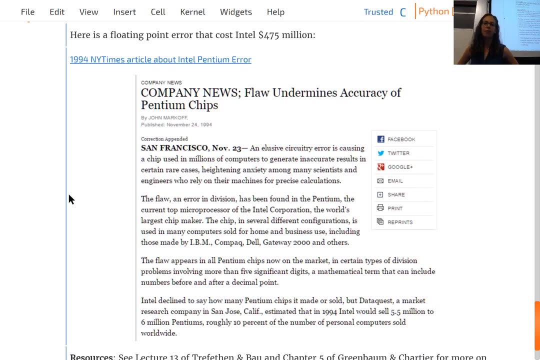 because it was like you have to look it up, i think the clock what might have was significantly off because it hadn't been reset, whereas this- um yeah, the kind of error accumulated and then another very expensive error is intel released a chip in 94 that in just in certain cases only had like five digits of accuracy. 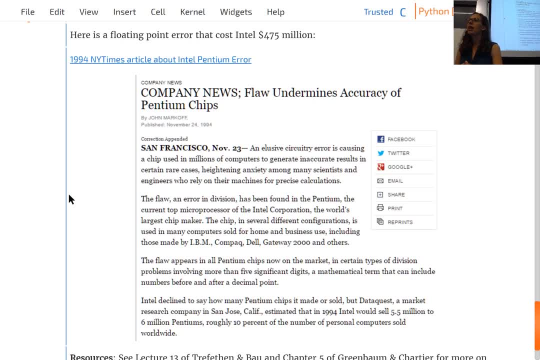 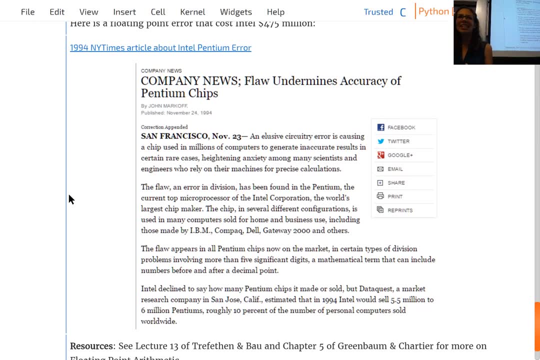 um, and so they ended up having to kind of do a recall on that and it cost them close to half a billion dollars. so just to highlight that this stuff does have a real world implications. i actually remember when that happened and i remember like a lot of the math libraries that were released had 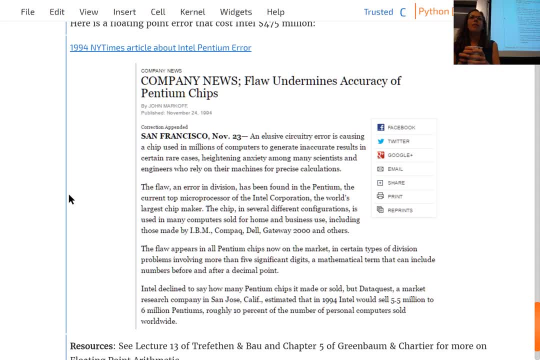 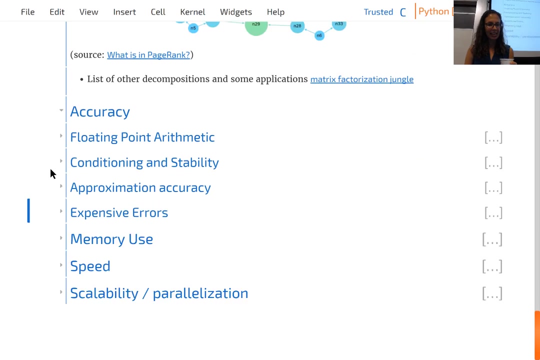 to be humble because they couldn't rely on this thing get sent back. so it was probably more than 475 million because, like i personally, wow, yeah, so that was just the cost to entail, not to people who, yes, yeah, so that's a. that's it for accuracy, and all these concepts will be. 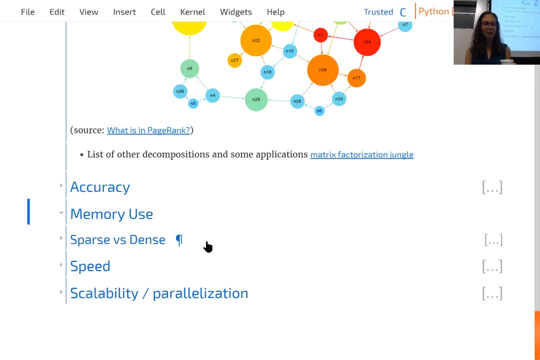 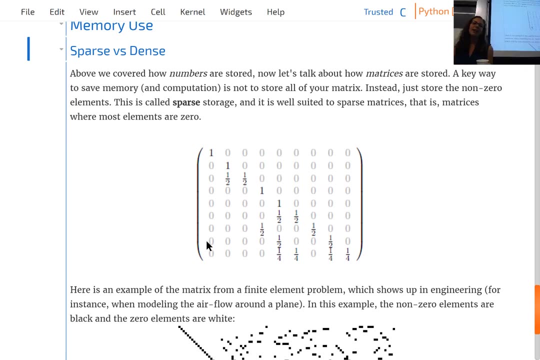 kind of return to as the course goes on. This is just introducing them. So memory use. So we've talked about how numbers are stored, now looking at how matrices are stored, And so a key way to save memory and also computation is not to store all of your matrix. 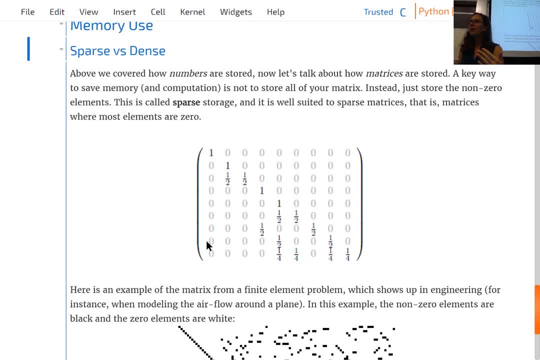 You could just store the non-zero elements and then you know, anything that you're not storing must be zero. This is called sparse storage, well suited to sparse matrices. Here's an example- And these actually show up a lot in problems- where you kind of have some sort of structure. 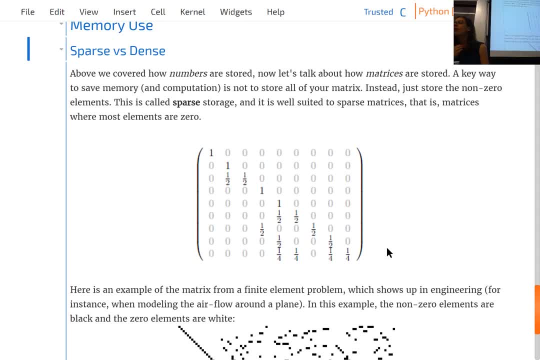 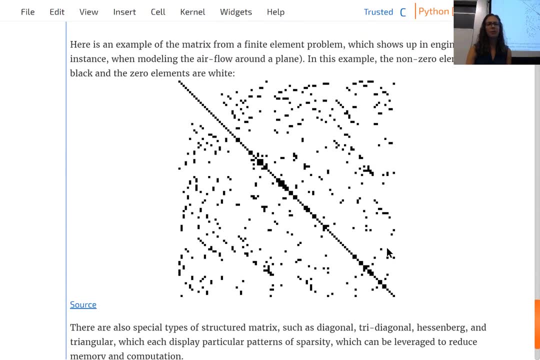 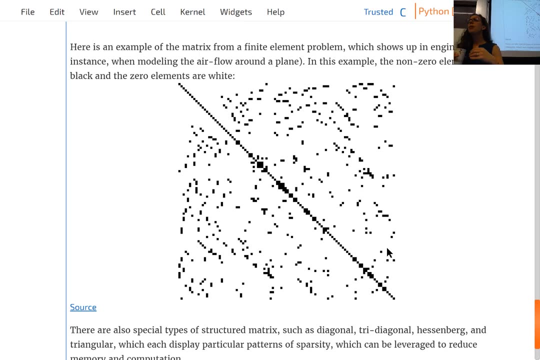 and maybe things on the diagonal or tri-diagonal are non-zero but that you have zeros elsewhere. This picture is from something called a finite element problem and they show up in engineering. We won't cover them here, but it's also a multi-grid problem. whenever you're kind of 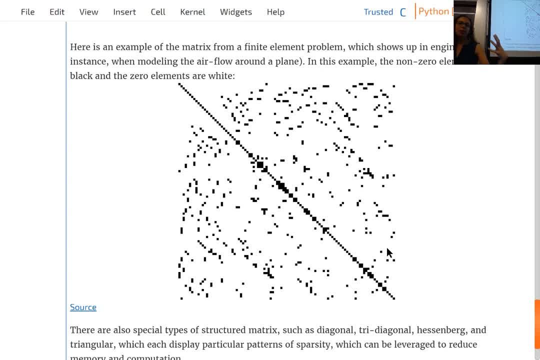 having to model, like I don't know, airflow around a plane engine or something, or nose of a plane. You get these matrices with sometimes very pretty patterns of where the non-zero elements are, And so in this picture this is, you know, like a hundred by a hundred. 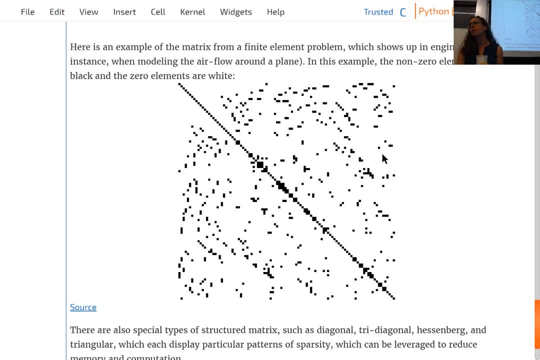 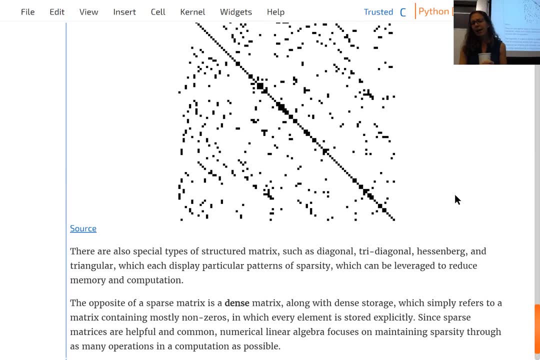 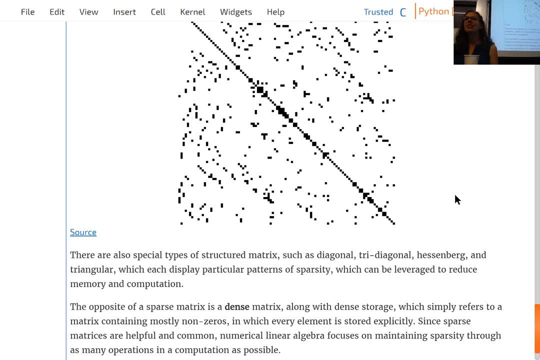 matrices, and black squares are non zero values, white squares are zero values, And so we'll come back to this, um, because SciPy- in a future lesson we'll kind of talk about SciPy- gives you three different ways to store a sparse matrix. So you, you know, once you've decided, like 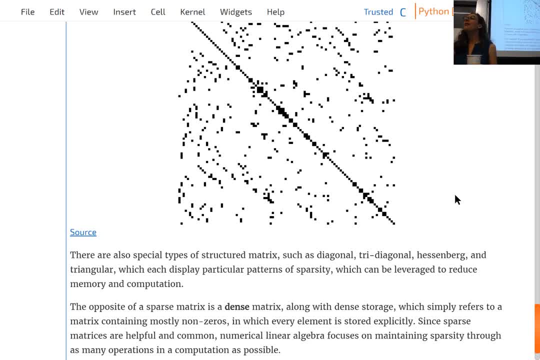 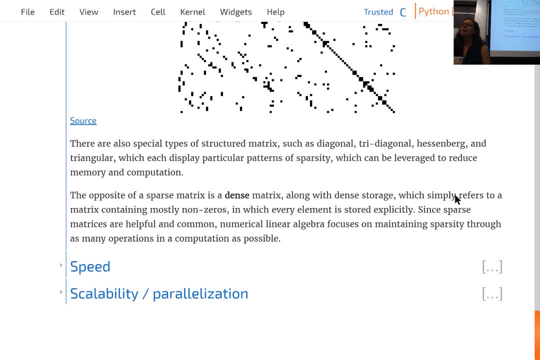 okay, I'm not gonna have a cell for everything you do have to kind of talk about like, okay, what are you gonna store to keep track of? so we'll return to that. and then the opposite of sparse is dense, which is probably kind of what you're. 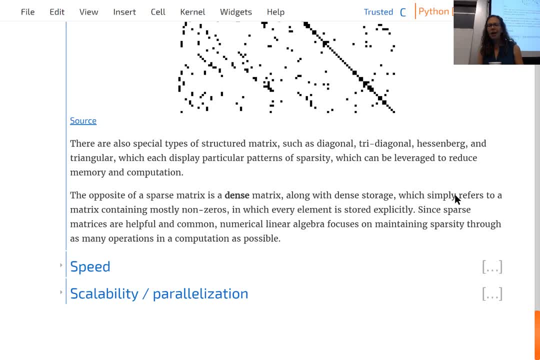 most used to, with both matrices and storage. and then, kind of as a rule of thumb, some people say that you can consider a matrix sparse if the number of nonzero elements scales with either the number of rows or the number of columns, whereas a dense matrix, the number of nonzero elements is scaling. 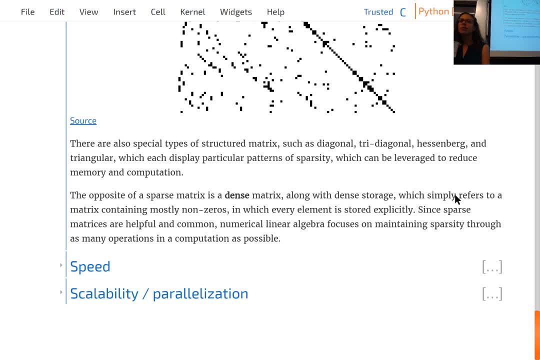 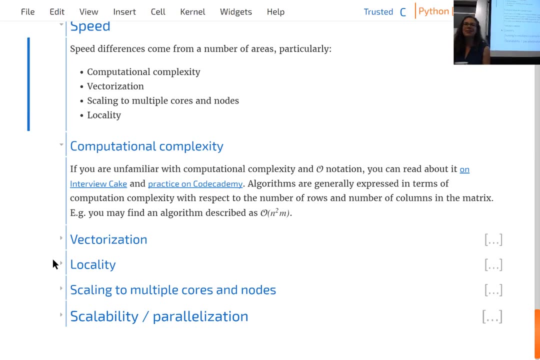 with the product of the number of rows and the number of columns. any questions about that? okay, so speed and speed is another one that has several kind of sub sub points underneath it, and things that affect the speed of your algorithm are the computational complexity of the number of rows and the number of columns, and 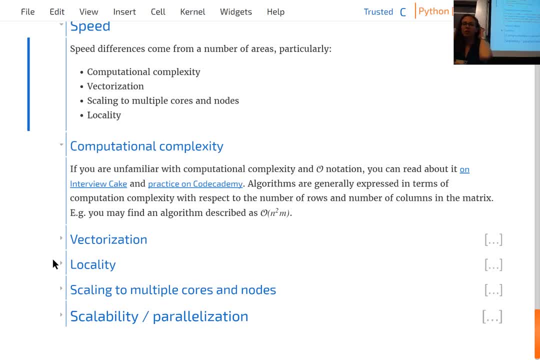 things that affect the speed of your algorithm are the number of columns, and things that affect the speed of your algorithm are the number of columns and vectorization, scaling to multiple cores and nodes and locality. we're not gonna- I'm really gonna- get into computational complexity and big O notation in here. 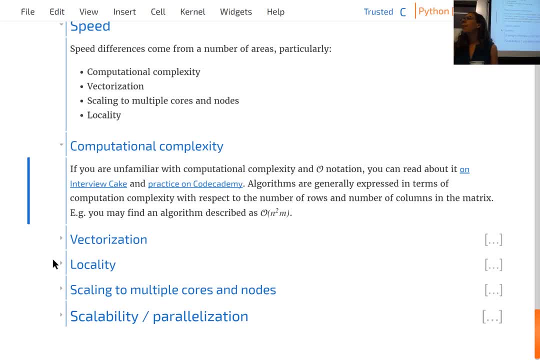 just to check who's familiar with big O notation. okay, I've linked to a few resources. kind of interview cake has a nice overview. and then I went through that kind of the start of Codecademy. I think has a really nice kind of buildup of it. has you doing? starts with simple. 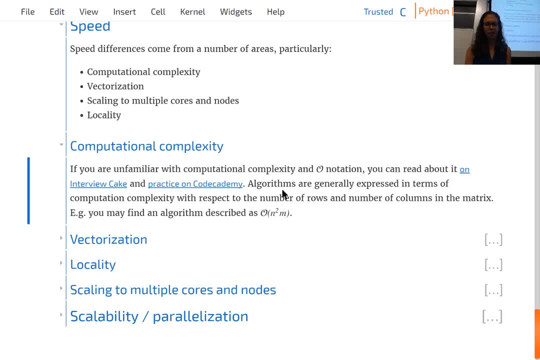 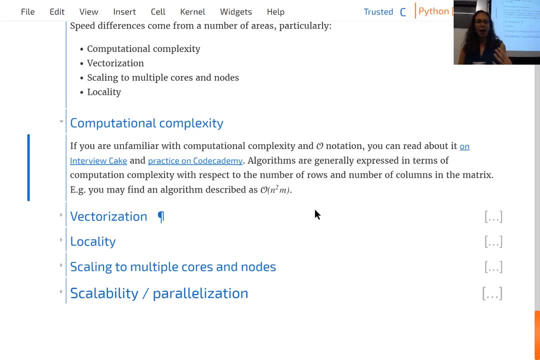 problems that kind of get more complex. but I think those are kind of useful tools if you do want to review it or learn about it. and typically, yeah, and this is something that in software engineering definitely comes up in every interview. data science, I would see, is more mixed, but will come up. 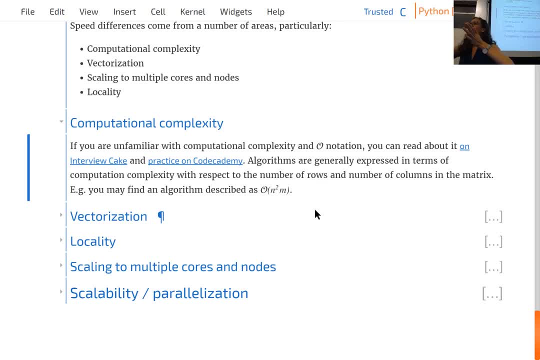 but like, yeah, like in coding boot camps, people kind of spend the first 80% of the course actually learning to build, web, develop, you know, build web apps and stuff, and then at the end it's like just study the theory of computational complexity because that's what you'll see on interviews and that kind of idea. 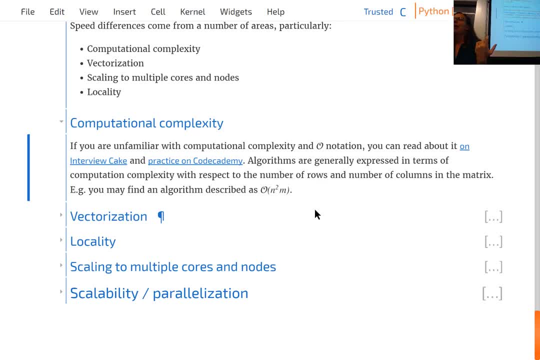 behind it is that it's giving you just this approximation, that's kind of like an order of magnitude. you're not interested in, kind, of your constant terms or even your coefficients of how, how slow things would be, and so if you had an m by n matrix, you might have you. 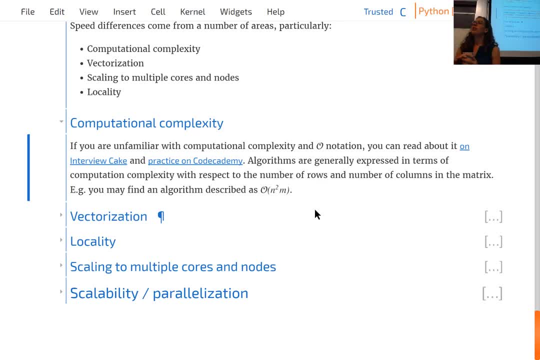 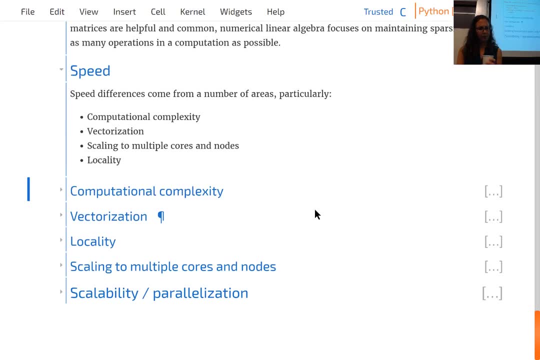 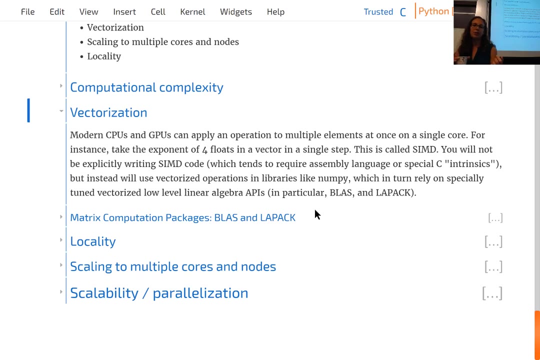 might describe an algorithm as being n squared times n if you were having to do- if that's kind of how many operations you had to do for your algorithm- vectorization, so modern CPUs and GPUs can apply the same operation to multiple elements at the same time. this is called SIMD: single instruction, multiple data. you will not be. 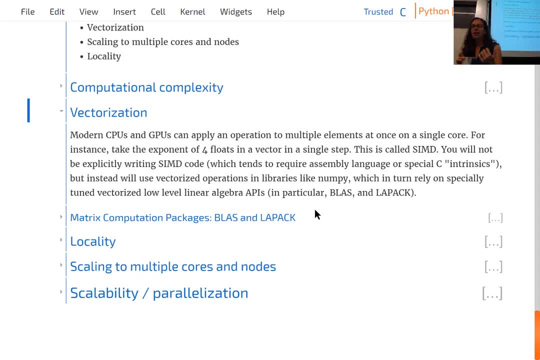 explicitly writing SIMD code and this is typically done in assembly. but libraries like NumPy, which we will use a lot, have been vectorized to do that and those rely on low level linear algebra. libraries such as Blass and LawPAC, which I want to say a little bit about, cuz you'll. probably hear about them and they're. they're like everywhere and so many ways to do this, because people think, well, this is actually a onto my left, that's a fair share, andcase as well is that that, and it's basically everything designed out of the library itself and done in the last week and that's what I wanted to show to the next part of the movies I've been. I'm working on other things here this morning. 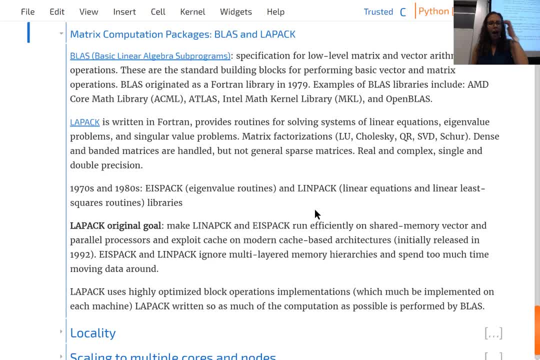 Diving Terrarium and you would- would maybe encourage anyone to with, would you know, enhancedSo. So BLAST started out as a Fortran library in 1979, and it's a specification for low-level matrix and vector arithmetic operations, so kind of the more basic like you're doing. 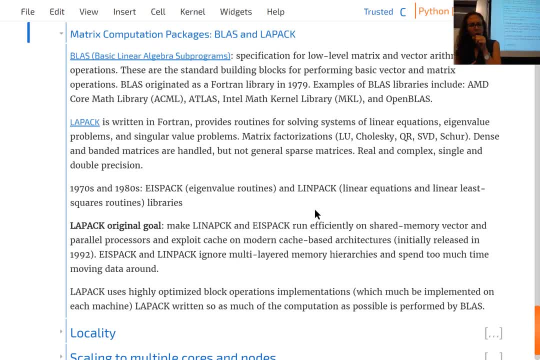 matrix multiplication or matrix vector product. Some examples of it include AMD, ATLAS, MKL and OpenBLAST, so you may hear about these. Then LAWPACK uses BLAST, and so it's kind of like a layer above it. 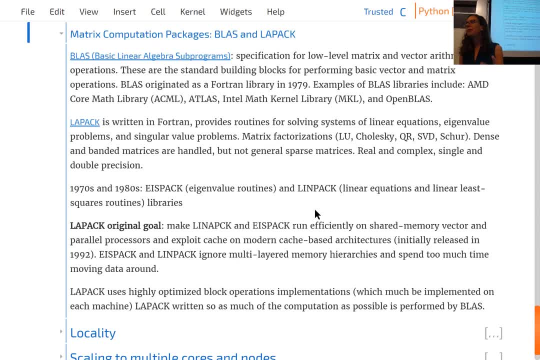 And LAWPACK is for matrix factorizations, which is what we'll be seeing in this course. So LU Tulesky, QR SVD. yeah, and LAWPACK arose out of Kind of previously there were two separate libraries, ICEPACK and LINPACK. 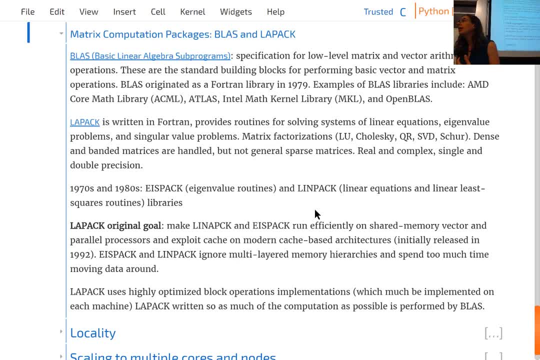 ICEPACK was for eigenvalue routines, LINPACK was for linear equations and neither of those were really taking advantage of cache. so they were developed in the 70s and 80s and I think LAWPACK came out in the early 90s to kind of take advantage of cache in modern 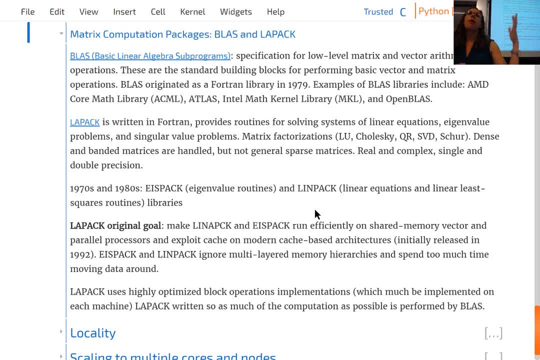 systems And you'll see, like if you're reading the SciPy source code, at many points you'll see it calling LAWPACK routines, and so there are points where, if you wanted to go in-depth, you can kind of look at that. 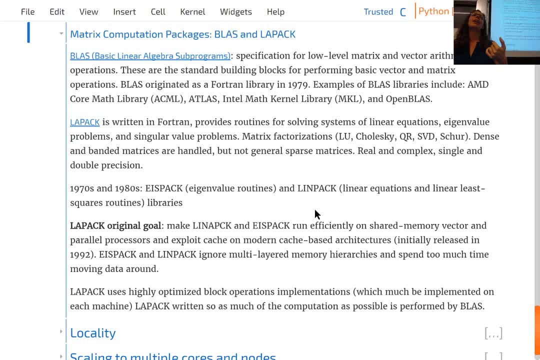 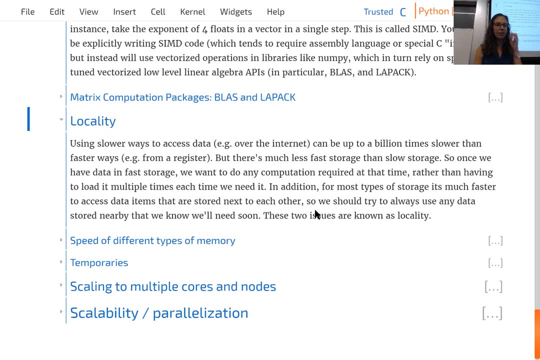 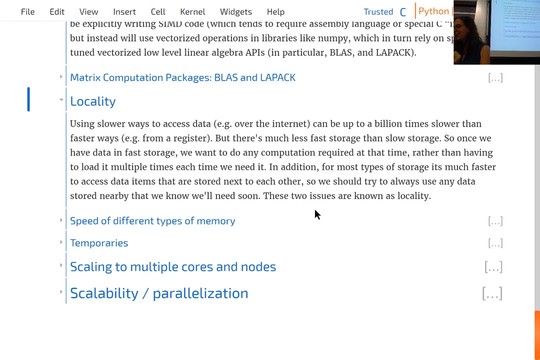 There's a lot of LAWPACK documentation to kind of see: okay, this is what is happening when SciPy calls this LAWPACK routine, Well, and then the next concept is locality, And so a lot of the kind of slowness from computers nowadays comes from when they're having to move data around from one location to another. So you know, if you're looking at- let's say you know- a lot of the data that's coming from the internet, you're looking at a lot of the data that's coming from one. 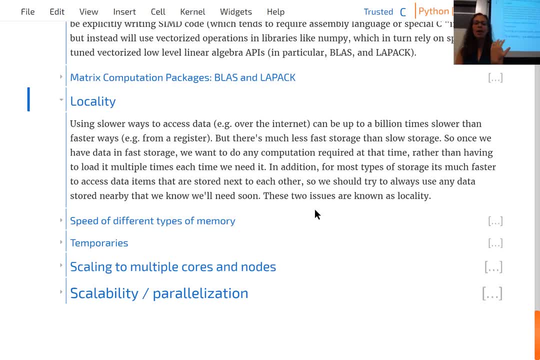 location to another, And slower ways to access data, such as getting something from the internet, can be up to a billion times slower than faster ways such as the register, which is basically the fastest memory, And it's important to remember that, basically, the faster memory is, the less you have of. 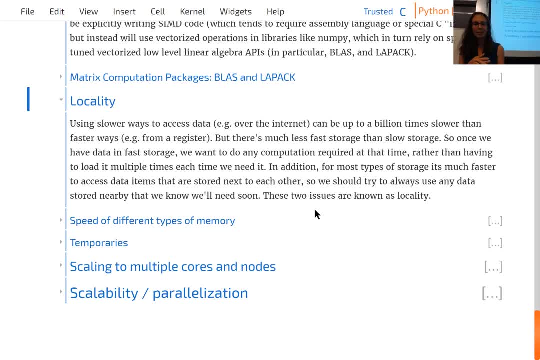 it, and so your fastest types of memory are much more limited in space, And so once you have data in fast storage, it would be great to- I don't know if you're going to have to do three computations with that data- to do a lot of that. 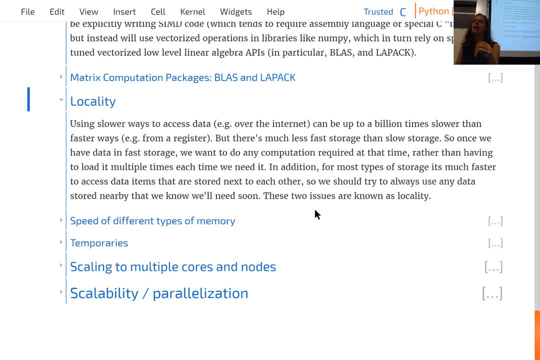 While it's in fast storage, as opposed to like putting it back in slow storage, retrieving it doing your second computation, putting it back in slow storage doing something else and then retrieving it for your third computation, because it's that you know having to retrieve. 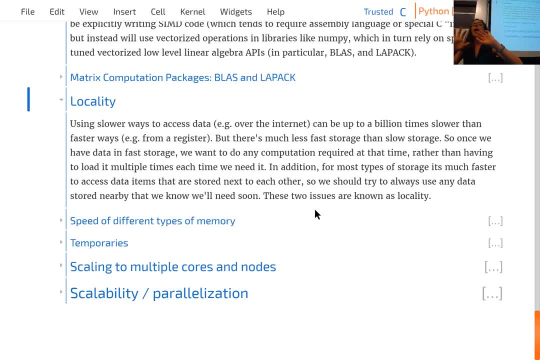 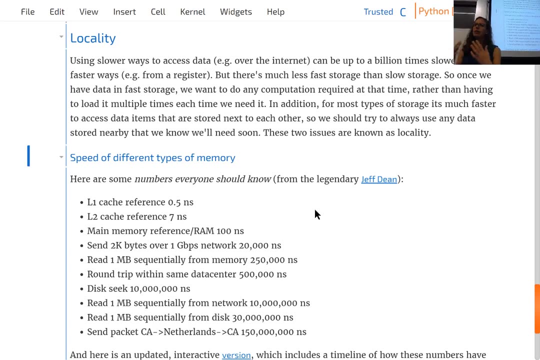 it. that's slow and so you really want to minimize those, and so kind of ways that you can group together you know times that you're going to use a particular piece of data are really helpful, And so kind of issues in that category are known as locality. 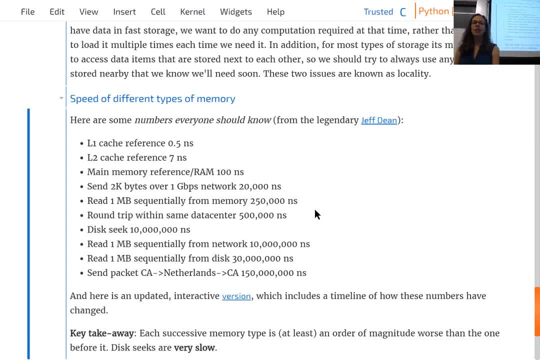 This is so. Jeff Dean of Google gave a presentation on numbers every programmer should know And these versions are from, and a lot of people still so. it's been years. a lot of people still share the slide show. There's an updated version. 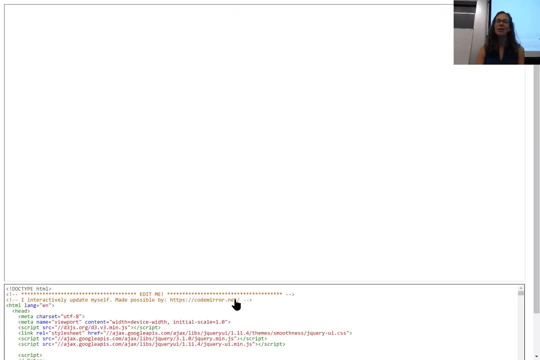 I would say the actually. let me open this because it's kind of neat. the updated version has like a slider So you can even look at like what the data is Okay, So you can see like what the numbers were in different years. 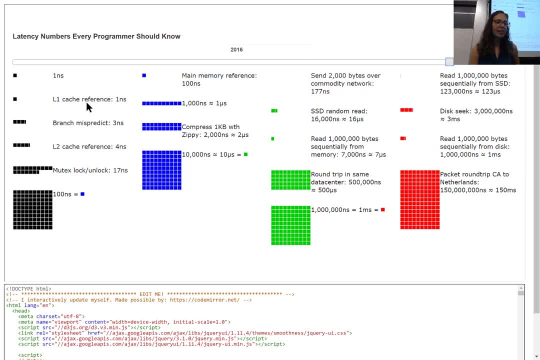 And the key thing to kind of look at is that an L1 cache reference- one nanosecond- that's kind of the fastest, fastest you can do- Main memory reference- and this is also kind of RAM- would be 100 nanoseconds. 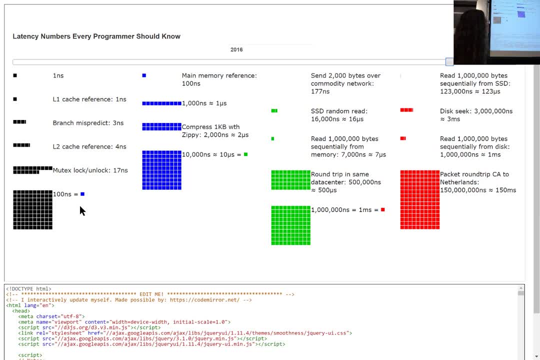 And here- I don't know if you can read this from there- they're switching colors, so they're changing colors. So 100 nanoseconds is you know, 100 black boxes is one blue box. So that's kind of what's going on with the colors in this picture. 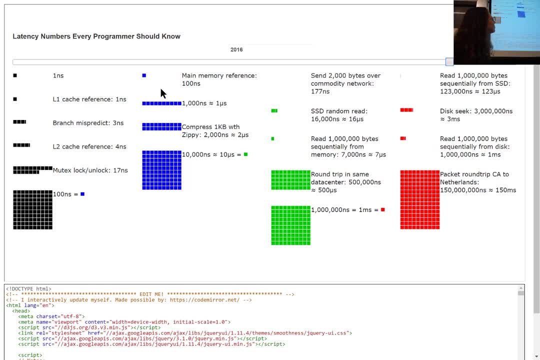 So main memory reference, okay, that's 100 times slower. And then if you get to disk seek, that's really slow. So that's 3 million nanoseconds. So it's kind of important to keep these in mind, Or the idea of kind of the orders of magnitude that you're seeing, as opposed to memorizing. 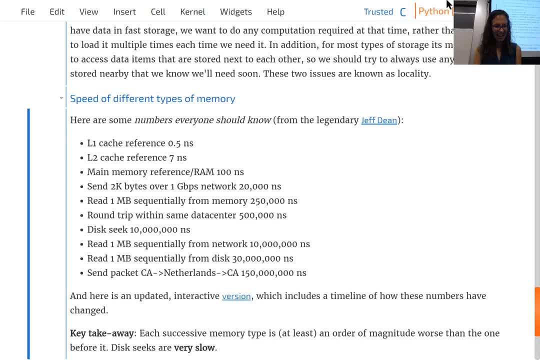 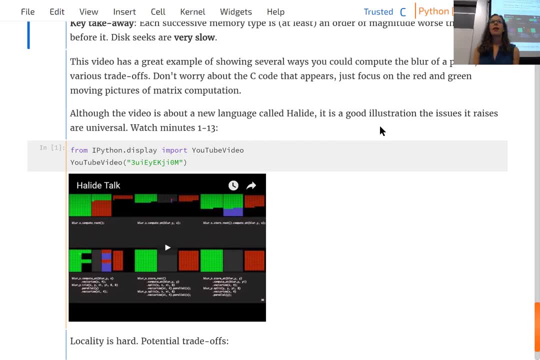 specific numbers. Okay, any questions, And I definitely encourage you to check out a lot of these links. So now I'm going to show part of this video, And so this video is about a language- It's kind of a language called Halide, which we will not be using, but it's just a really 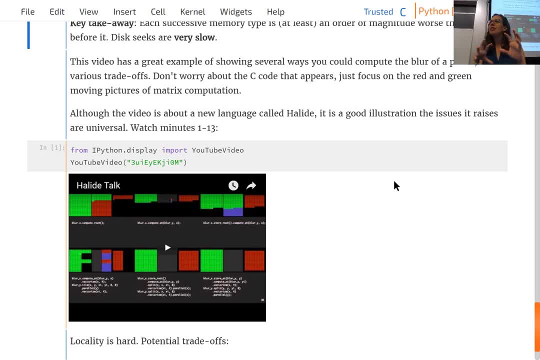 good illustration of some of the things you would have to think about in kind of thinking about what order to do things in. And so in the video- don't worry about just briefly- at the beginning he shows kind of a bunch of code. There will be these kind of visualizations, though, with green boxes and green means. 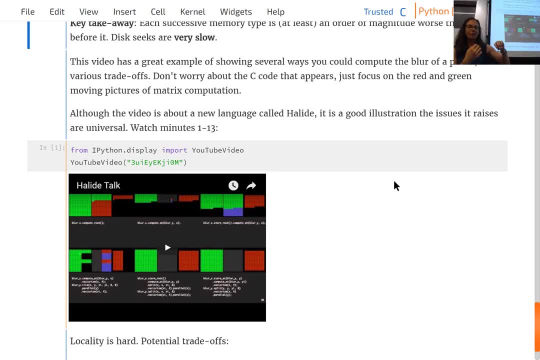 that you're reading something and red means that you're writing kind of what order things are happening in. Okay, So what we're looking at is just the blur of a photo, so kind of taking. a lot of the developers on Halide work at Adobe so they do a lot of kind of photo processing. 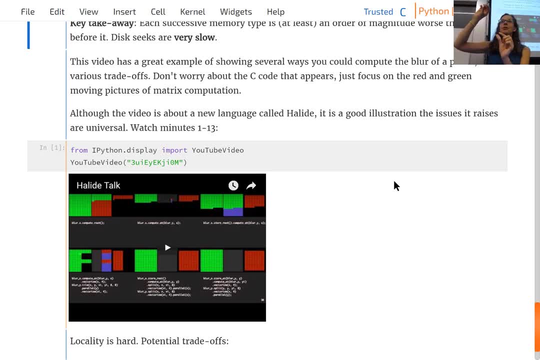 But the idea of just you need to read, you know, a few pixels to be able to give the XY blur. So you're kind of taking this photo and then we want to look at a few pixels around it to get what the blurred version would be. 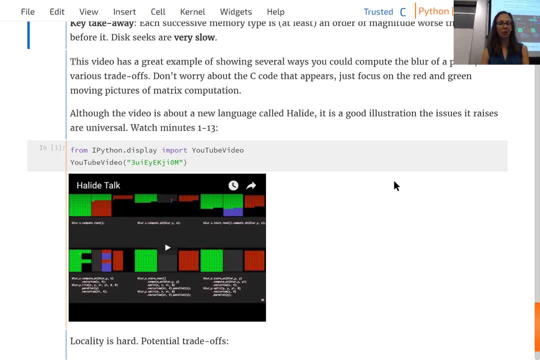 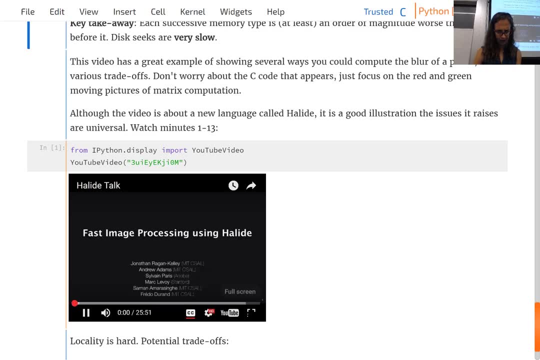 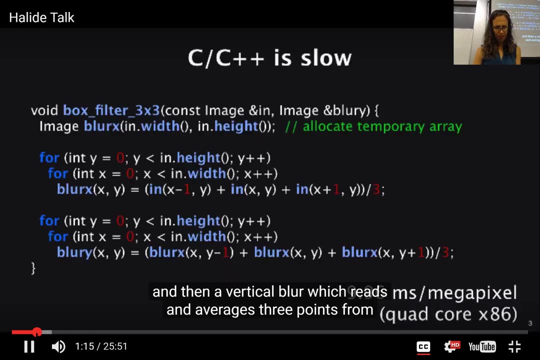 Oh yes, this is a convolution, So kind of similar to what we saw before, that idea of kind of sliding a filter. Okay, So this is a convolution. Okay, Let's try that. Hi, I'm Andrew Adams and this video is about Halide: a new language and then a vertical. 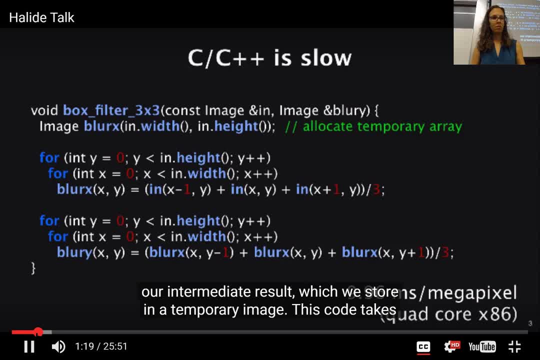 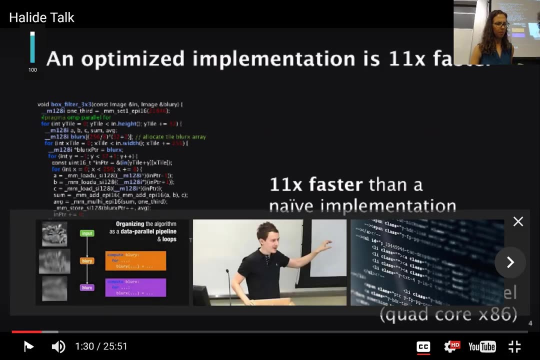 blur, which reads and averages three points from our intermediate result, which we store in a temporary image. This code takes about 10 milliseconds per megapixel on the quad core x86 that I benchmarked it on, But an optimized implementation for this machine is more than 10 times faster. 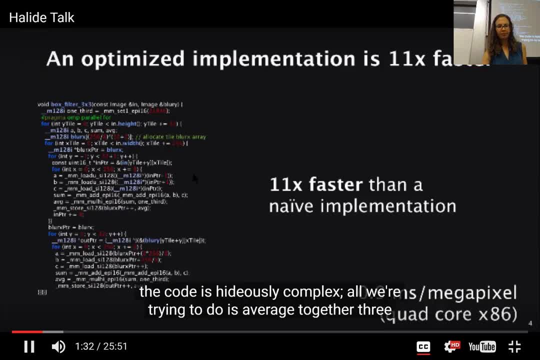 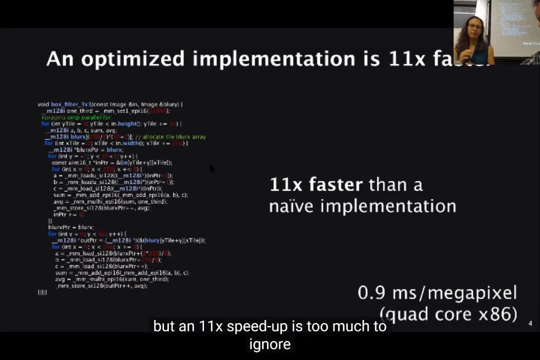 Do you think I should turn the volume on for the computer? Let's try that. Okay, So the code is hideously complex. All we're trying to do is average together 3 by 3 pixels, But an 11x speedup is too much to ignore. 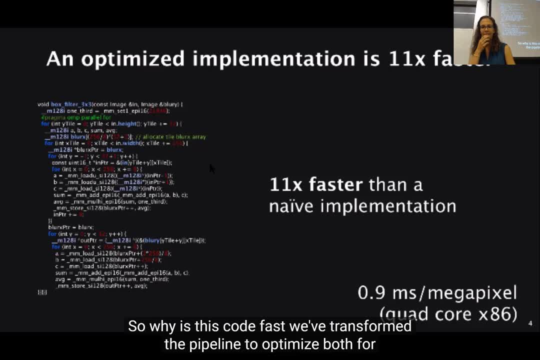 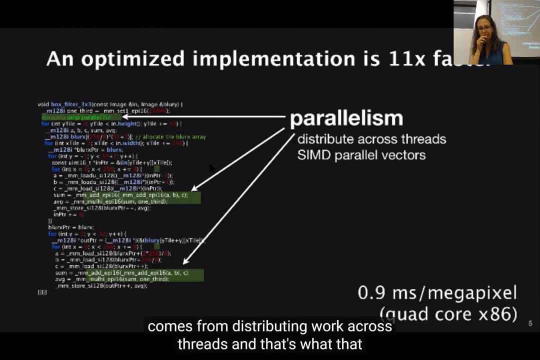 So why is this code fast? We've transformed the pipeline to optimize for both parallelism and locality. The parallelism comes from distributing work across threads- and that's what that pragma omp parallel 4 at the top does, and also from computing an eight wide SIMD chunks on each. 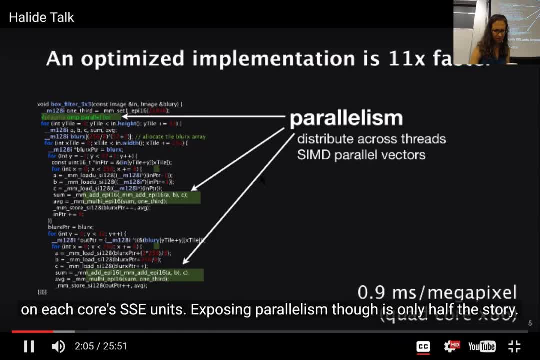 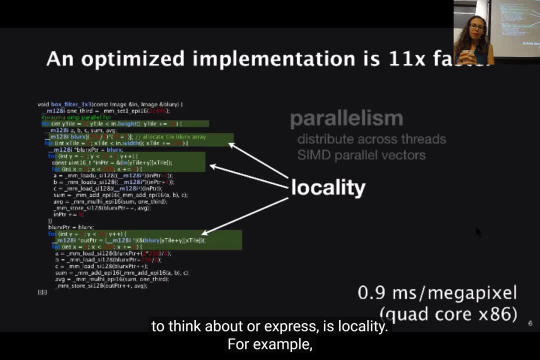 core's SSE units. Exposing parallelism, though, is only half the story. Just as important, and often much harder to think about or express, is locality, For example, making sure the pixels produced by one stage are still in cache when the next. 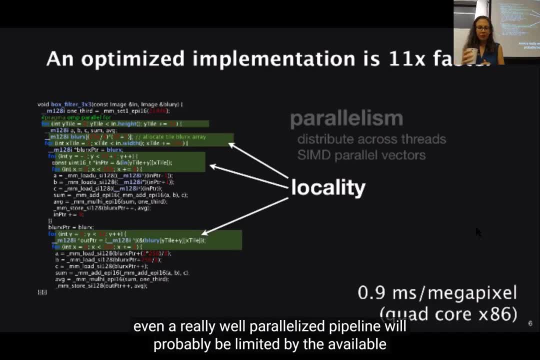 stage reads them, And without locality optimization even a really well parallelized pipeline will probably be limited by the available memory bandwidth. So here the optimized code improves locality by computing each stage individually. So let's see what we can do. First, we compute the computation of tiles, interleaving the computation of tiles across. 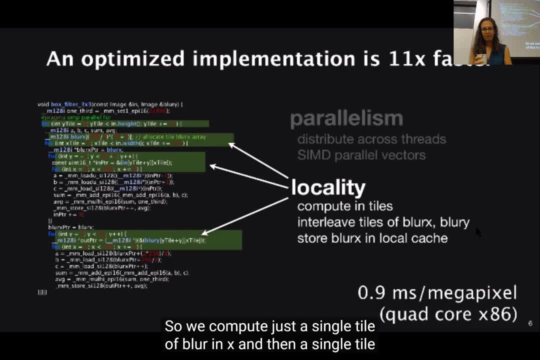 stages. So we compute just a single tile of blur in x and then a single tile of blur in y And then we go back to compute the next tile of blur in x. So this hopefully keeps all that intermediate data in small buffers that never leave cache. 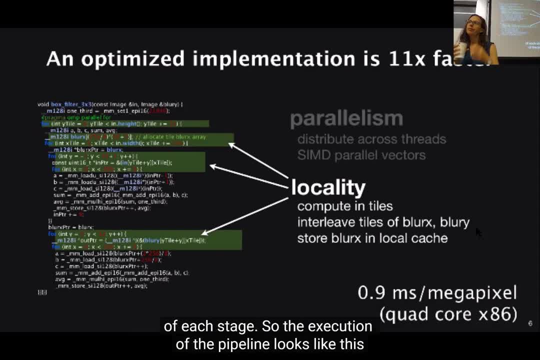 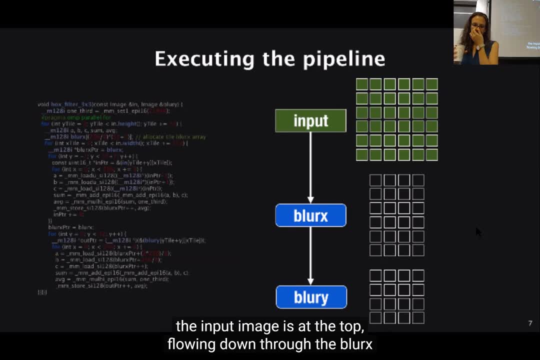 But it complicates the code because it's interleaved the computation of each stage. So the execution of the pipeline looks like this: The input image is at the top, Flowing down through the blur x and blur y stages below. The earlier stages are evaluated over larger buffers because we're computing filters that 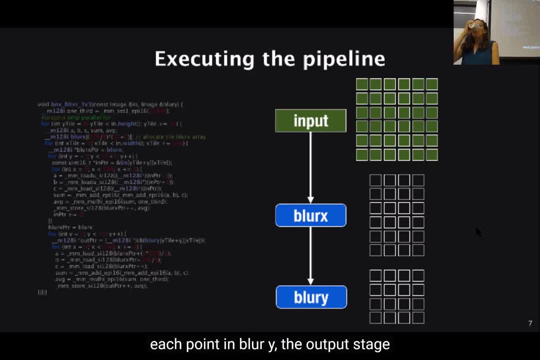 have a footprint. so we need more inputs than there are outputs. Each point in blur y, the output stage, depends on three pixels in blur x, which in turn depend on nine pixels total in the input. So the unoptimized version that we looked at first computes every pixel in the first 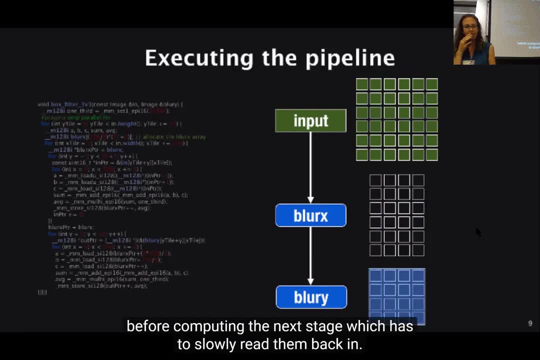 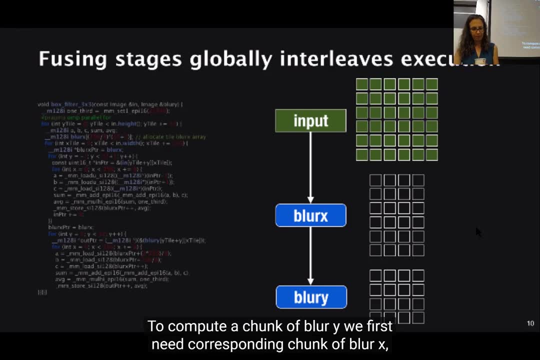 stage, writing them out to memory before computing the next one, Or computing the next stage, which has to slowly read them back in. The optimized version interleaves the stages. instead, To compute a chunk of blur y, we first need the corresponding chunk of blur x, which loads. 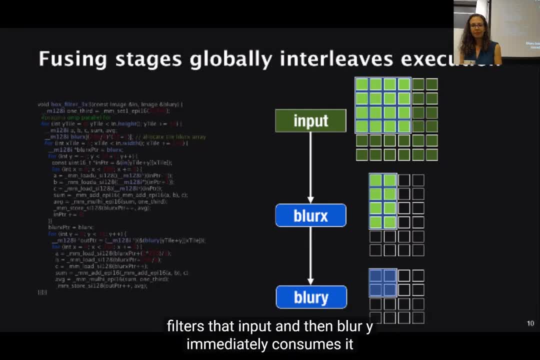 a chunk of the input. The blur x stage filters that input and then blur y immediately consumes it to compute a chunk of the output. So next we throw away that intermediate data, that chunk of blur x, load the next chunk of the input. 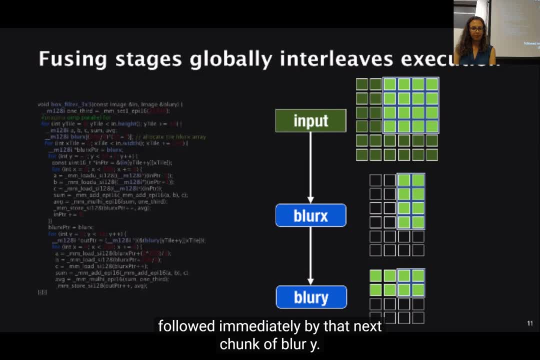 The next chunk of blur x, followed immediately by that next chunk of blur y. So we've moved the computation of each chunk of pixels in a consumer stage, closer in time to the computation of its inputs. This improves producer-consumer locality by keeping all the intermediate data nearby. 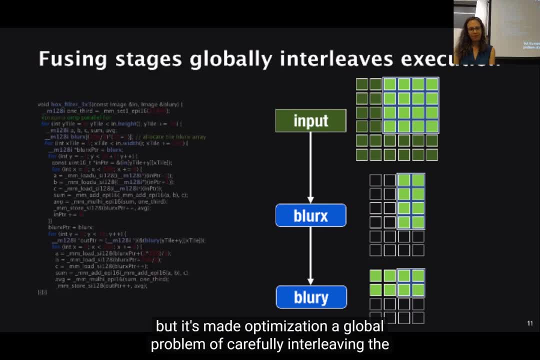 in local caches. But it's made optimization a global problem of carefully interleaving the computation and storage down an entire imaging pipeline. You can't address locality just by optimizing stages in isolation or by just tweaking operations in your interleaves. Also, we're making a trade-off here. 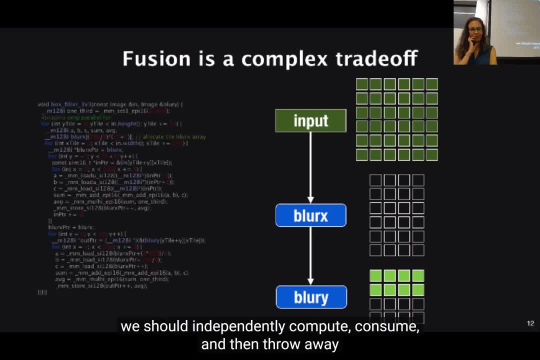 We're saying that for each chunk of blur y we should independently compute, consume and then throw away the required chunk of blur x. This means that neighboring chunks which depend on overlapping pixels from higher up in the pipeline do redundant work where they overlap. 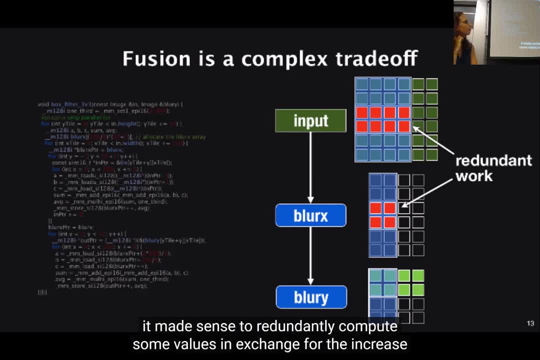 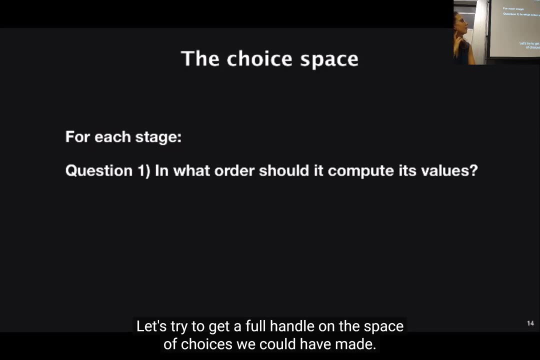 Now for this pipeline. it made sense to redundantly compute In exchange for the increase in locality that we get by never letting the intermediate values move out of cache into main memory, But this is not always the right choice. Let's try to get a full handle on the space of choices we could have made. 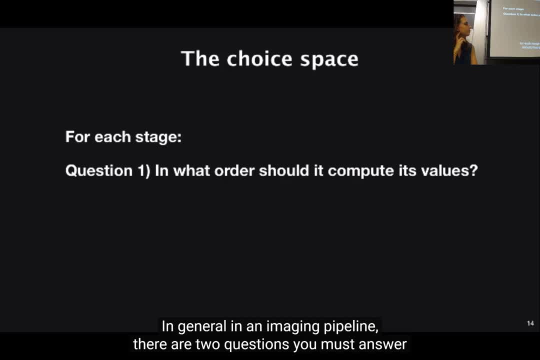 In general, in an imaging pipeline, there are two questions you must answer for each stage. The first is: in what order should that stage compute its values? Let's look at some choices. The most common way to traverse a pipeline is to compute the value of each chunk of blur y. 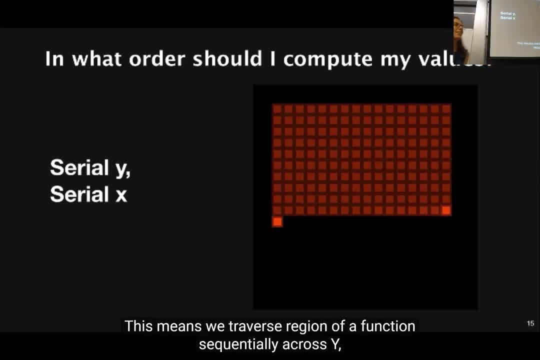 The most common way to traverse a pipeline is to compute the value of each chunk of blur y. The most common way to traverse a region is in scanline order. This means we traverse a region of a function sequentially across y and within that sequentially. 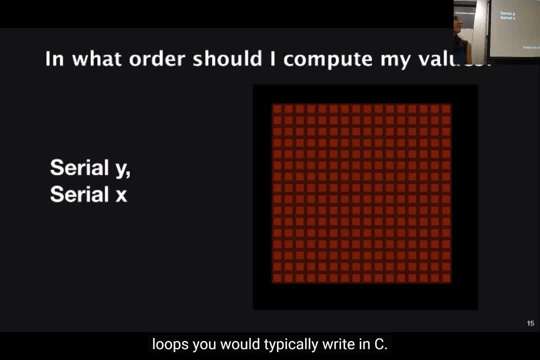 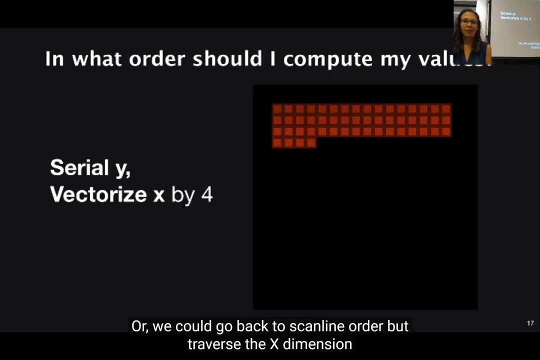 across x. This walks down scanlines, just like the loops you would typically write in C. We can transpose the x and y dimensions, which gives a column-major traversal which walks down each column in turn. Or we could go back to scanline order but traverse the x dimension in vectors of width 4.. 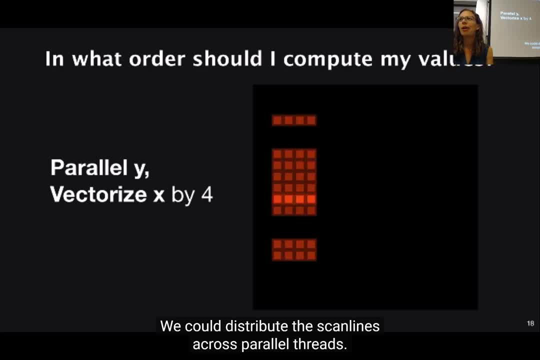 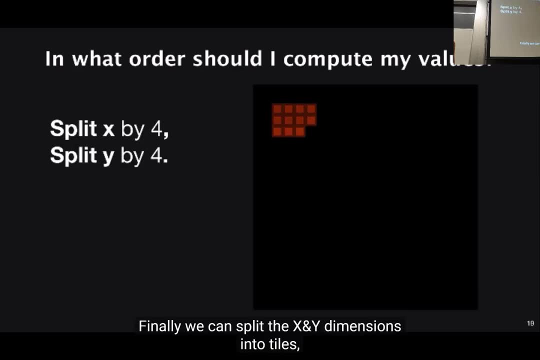 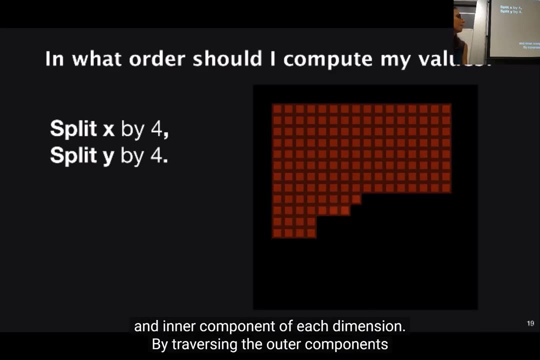 We could distribute the scanlines across parallel threads. Finally, we can split the x and y dimension into tiles, which opens up further recursive choices for the order of the outer and inner components of each dimension. By traversing the outer components outside the inner components, we get a simple tiled. 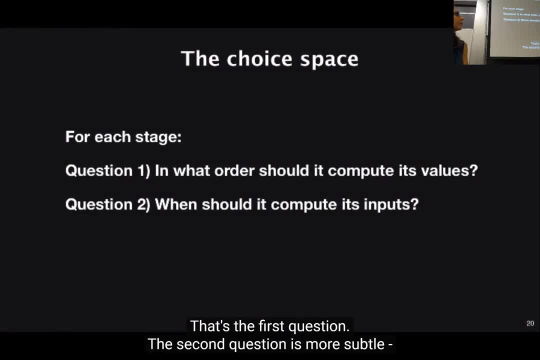 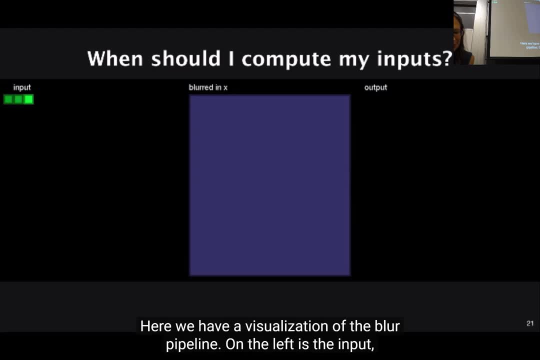 traversal. That's the first question. The second question is more subtle: When should each stage compute the value of x and y dimensions? Let's look at some options. Here we have a visualization of the blur pipeline. On the left is the input, on the right is the output and in the middle is the blur. 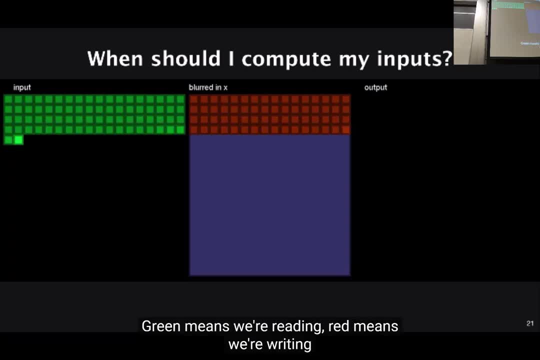 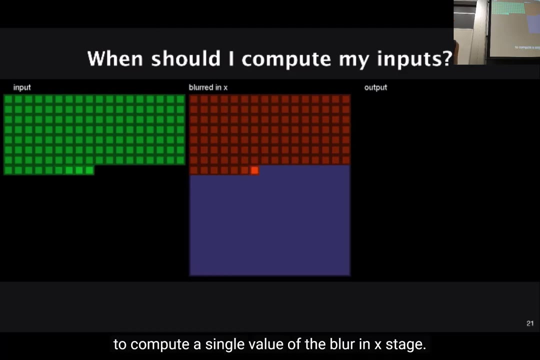 and x stage: Green means we're reading, red means we're writing and blue means we've allocated a temporary buffer. So right now we're reading from the input and using it to write. to the blur and x stage, We read three values from the input: one, two, three. to compute a single value of the. 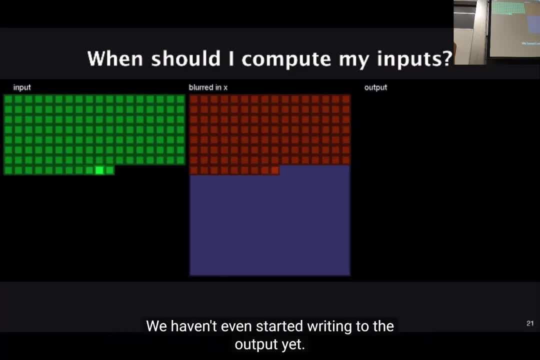 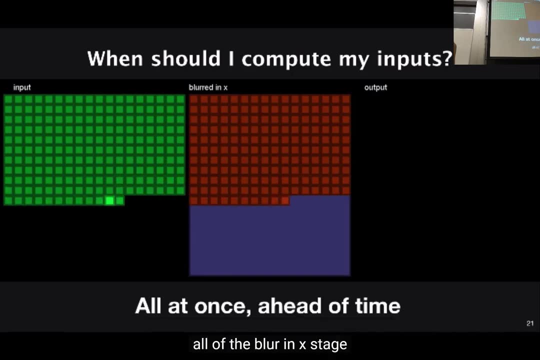 blur and x stage. We haven't even started writing to the output yet, So the choice we've made here is that we're going to compute all of the blur and x stage before computing any of the blur and y stage. If we phrase this as a decision made by blur and y, that decision is compute all of my. 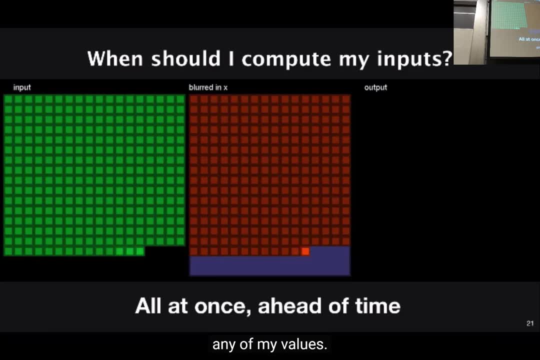 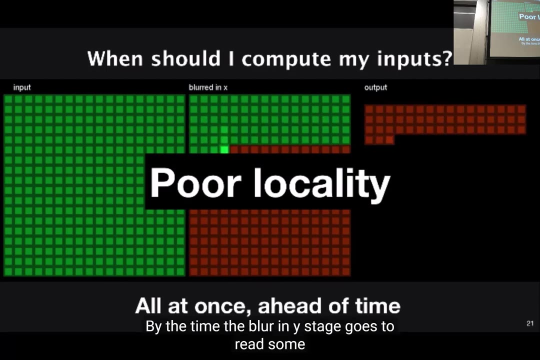 inputs ahead of time, before I start computing any of my values. So what's the pitfall with this approach? Why is this slow? Well, it's not that slow. The answer is, of course, locality. By the time the blur and y stage goes to read some of the intermediate data, it's probably. 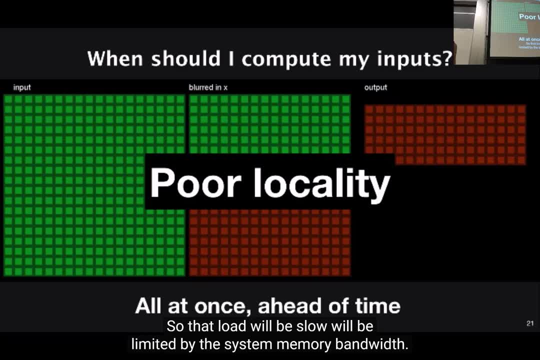 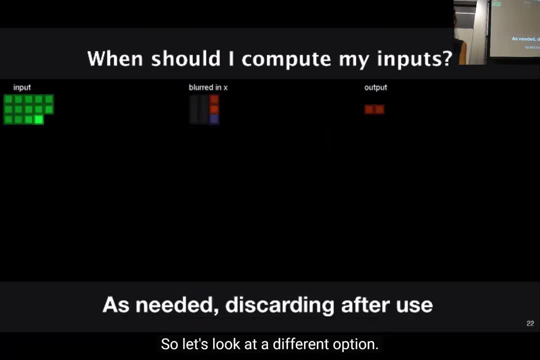 been evicted from cache, So that load will be slow and it will be limited by the system memory bandwidth. So let's look at a different option Here. we compute three values of blur and x by reading nine values from the input and 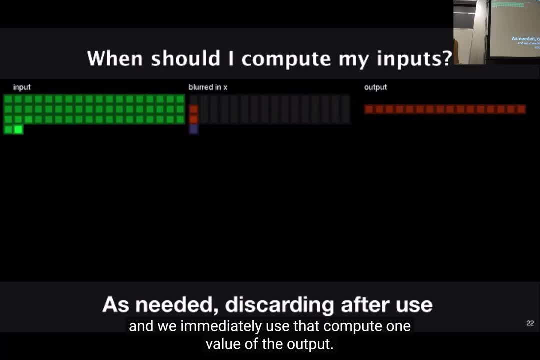 we immediately use that to compute one. So here we get maximum locality. We're using data as soon as it's available, without giving it any time to be evicted from a cache. What's the pitfall here? Well, if you look carefully at what the blur and x stage is doing, you'll realize that. 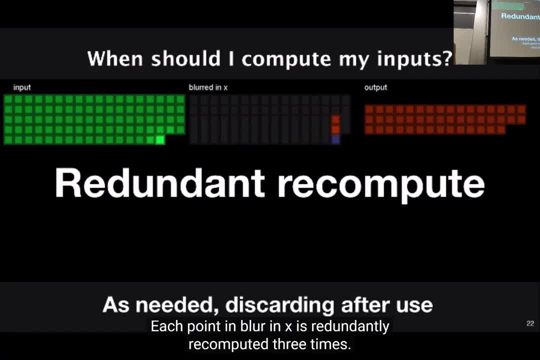 we're doing a lot of wasted work. Each point in blur and x is redundantly recomputed three times. OK, Well, we're done, We're done. So maybe we can figure out how to get around that. Here's another choice. 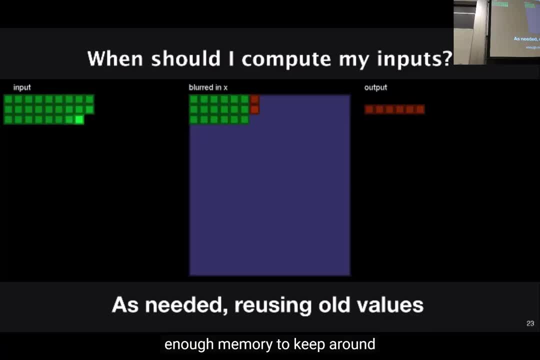 At first it's going to look similar, but notice that we've allocated enough memory to keep around all of the intermediate stage and we're not throwing away values as we go. That means when we get to the second scan line, we can start reusing values that we 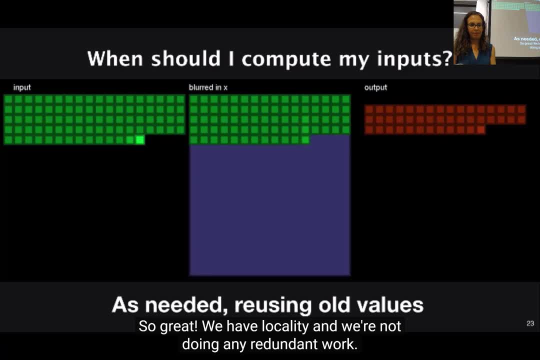 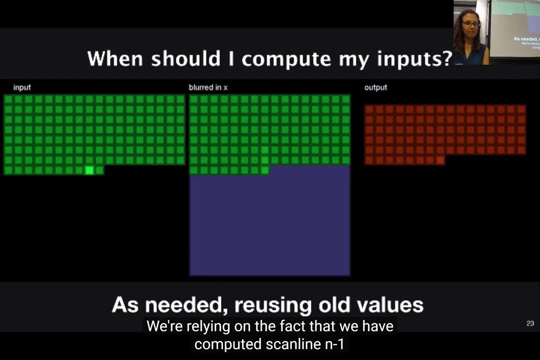 computed earlier. So great, We have locality and we're not doing any redundant work. What's the pitfall here? We've introduced a blur. We've introduced a serial dependence in the scan lines of the output. We're relying on the fact that we've computed scan line n-1 before we can start computing. 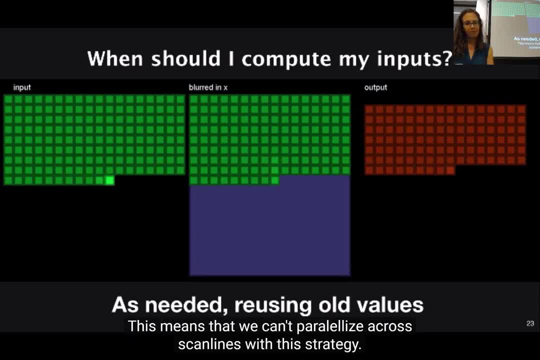 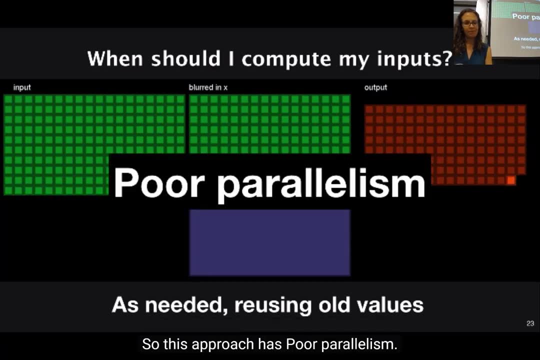 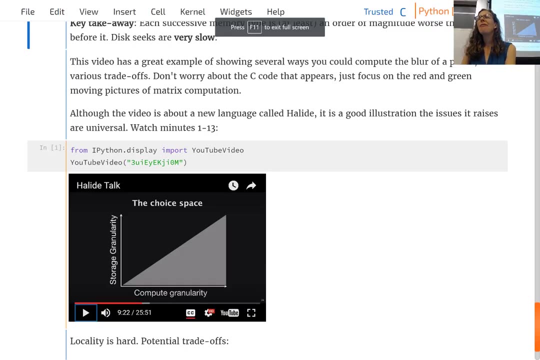 scan line n. This means that we can't parallelize across scan lines with this strategy. With the previous two strategies we could, So this approach has poor parallelism. I'll go ahead and stop it here. I really like OK. 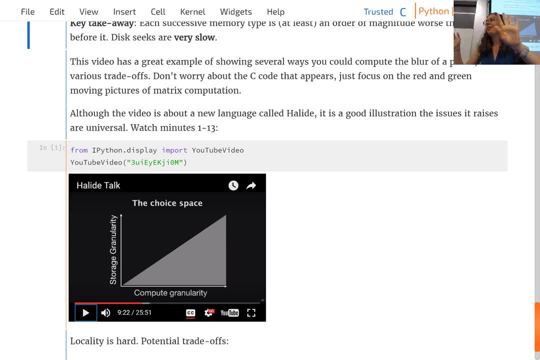 It's not very interesting, So I'm going to just go ahead and take a second and go back to the first one. All the things that I've shown you are all very different And I think it's important to know whether the algorithm is going to be using kind of. 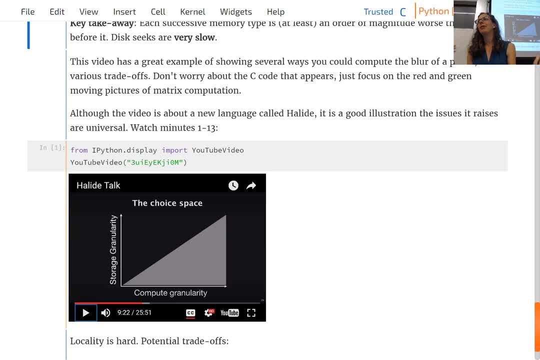 that visual approach, if he's kind of showing these different ways of doing the same computation and that each one has different positives and negatives And in fact none of them seems ideal because there's kind of a tradeoff, no matter what. I was just going to mention that later on we are actually going to build an algorithm. 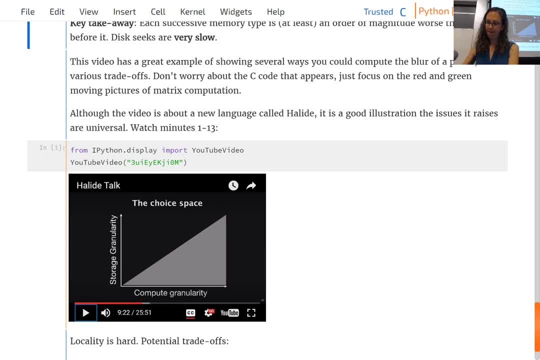 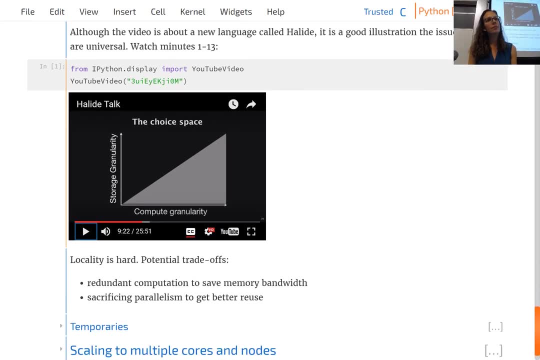 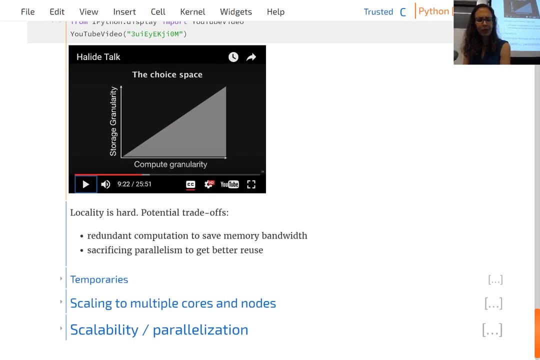 in all of those different ways in Python and see how they are different. So keep that video in mind, because when we get there, we'll be using the algorithm in Python and see how they are different there. it'll be useful to think about those pictures. yeah, thank you, um, and then something. 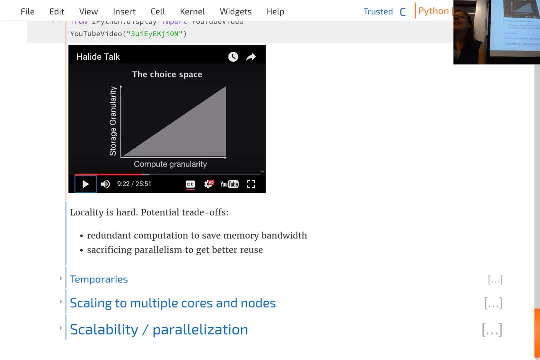 kind of that he said in the video. it's just locality is really hard because you kind of have trade-offs. it feels like, no matter what you do, sometimes redundant computation can save you memory, bandwidth, um so kind of computing things multiple times means that you, you know, you don't. 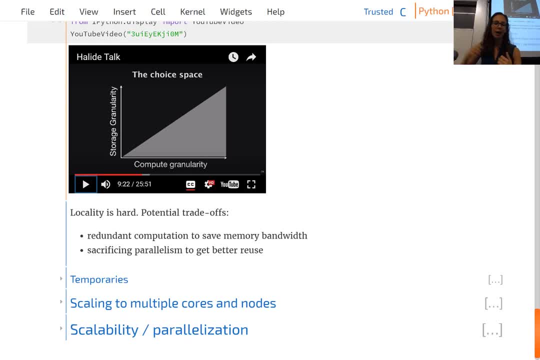 have to kind of be pulling them in and out of memory as much, or you can sacrifice parallelism to get better reuse, but then you can't parallelize and he kind of says- and the people building this are experts who have been working in adobe for a long time, like they really often just have to try. 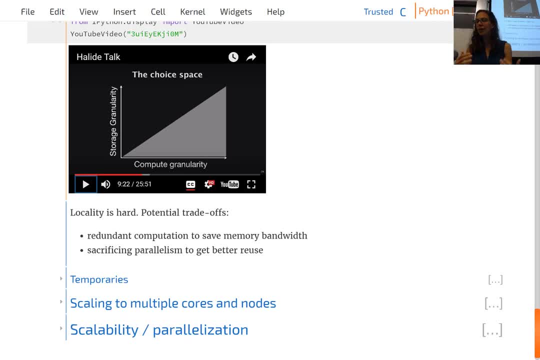 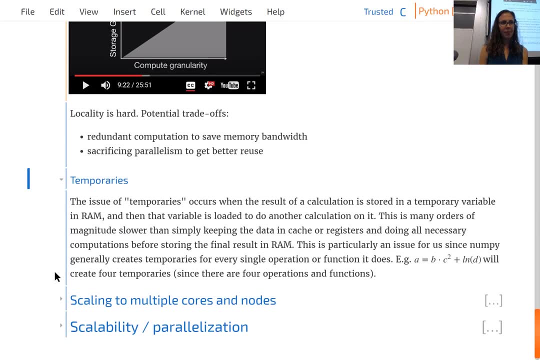 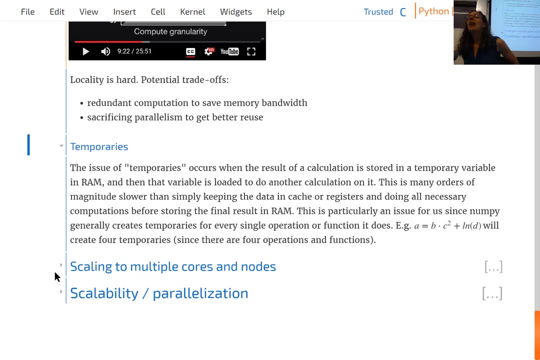 a bunch of different stuff and it can be hard to predict what's going to end up being fastest and then kind of another, um, oh yeah, the difference in speed that rachel's talking about is many orders of magnitude, not a few percent, so this isn't like a minor thing. these are things where, like in practice, 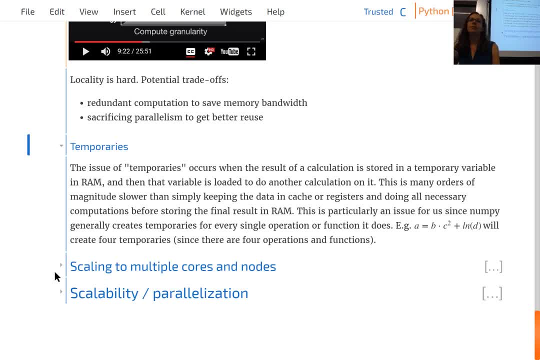 you'll run something overnight. it hasn't finished. you'll make one of these small changes and it runs in three seconds. it can be that big. yes, thank you. yeah, if it was a minor difference in speed it wouldn't be worth the bother. um and something, even, i think, in the 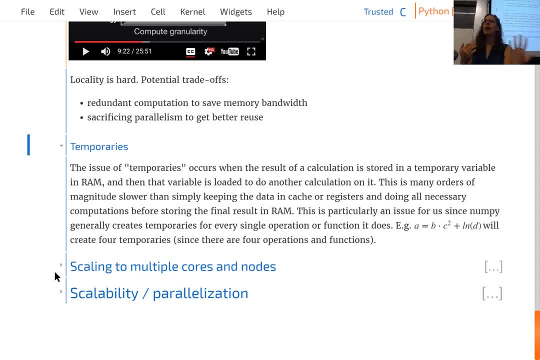 part i showed you. he mentioned kind of getting an 11x speed up by writing this more complicated version, and it's- i mean, i couldn't even see what the code said, but it was a full screen of code just to do this blur and x, blur and y operation. and then another issue that comes up is temporaries. 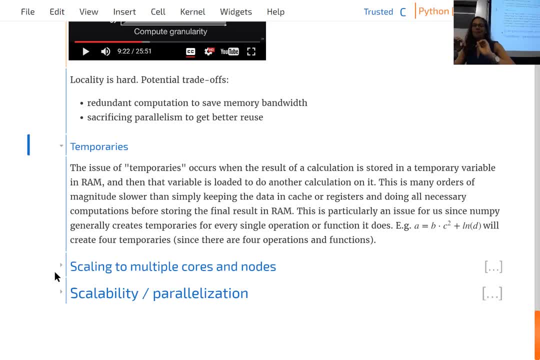 and that's when you're doing a calculation and kind of temporary variables end up getting stored, and so this can be a lot, a lot slower than if you're able to keep all the data in cache. so this is if the temporary variables are stored in ram. 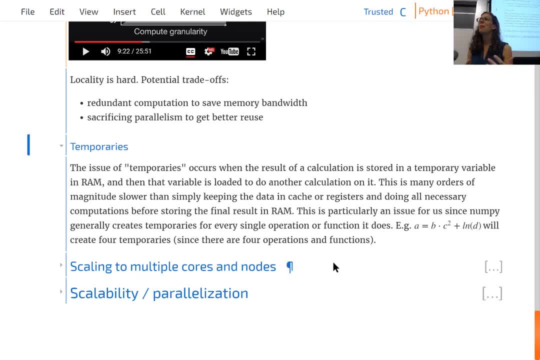 um, numpy creates temporaries for kind of every operation. it does. so if you were doing a equals b times c squared plus the natural log of d, what numpy would have to do is calculate c squared. store that, multiply that by b. store that result. take the natural log of d. store that somewhere. 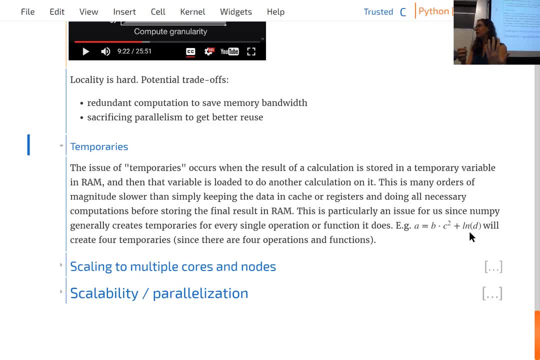 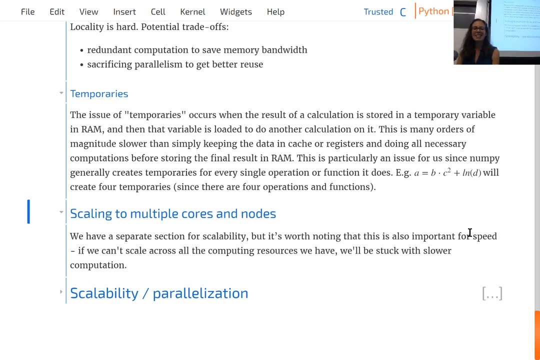 and then use those two variables that's stored, you know, to add them together and give you the answer you want, and so kind of along the way, numpy is having to deal with that a lot more than just creating temporary variables and putting them somewhere. and then i'm about to get to the scalability section. 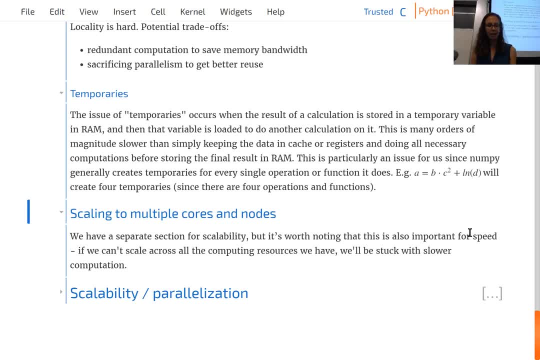 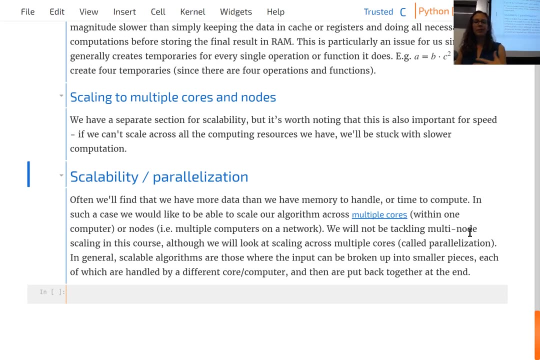 but i just want to note that scalability definitely impacts the, the speed of what you're doing and whether you're kind of fully taking advantage of the resources that you have. so for scalability, um kind of there's, the one approach is to be able to scale an algorithm across multiple cores within a 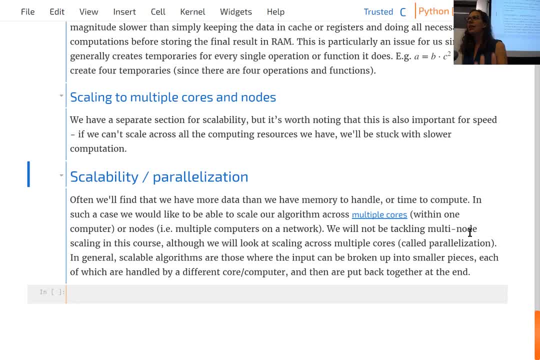 single computer or scaling across multiple computers in a network, which we will not be covering. um, but yeah, we will talk about kind of parallelizing, which is scaling across multiple, multiple cores in a computer. um, yeah, and i think this is great timing. um, i can take questions. oh, yes, 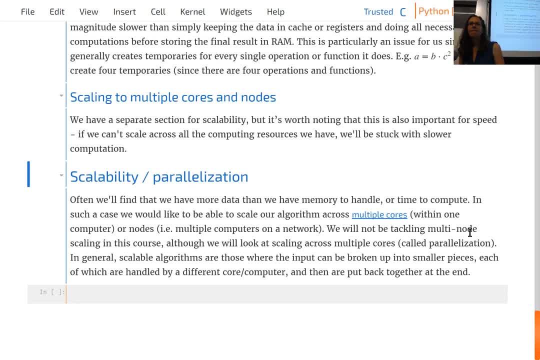 just a tip. um, you'll see that rachel's used a lot of hierarchical headings and it's really easy to navigate those and understand her thought process by collapsing sections. you need to install a num, a jupyter extension called collapsible headings for that to work. 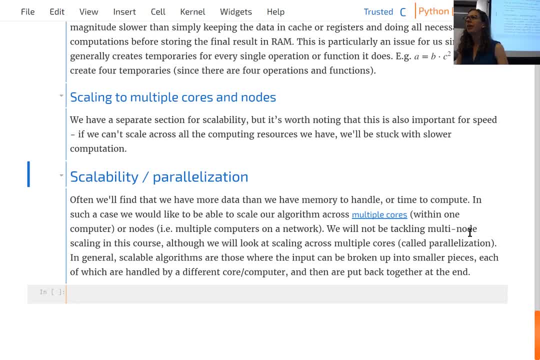 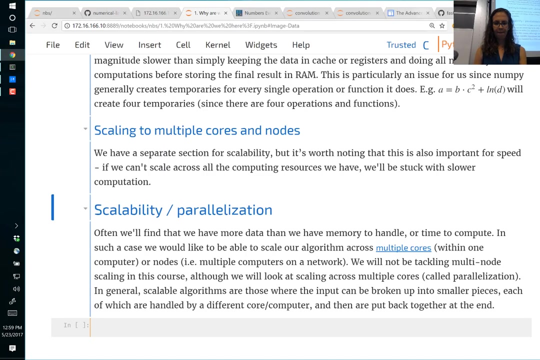 so you might want to look at installing that extension. yes, yeah, that's a great extension, any questions? okay, well, i'll see you on thursday, thanks you.